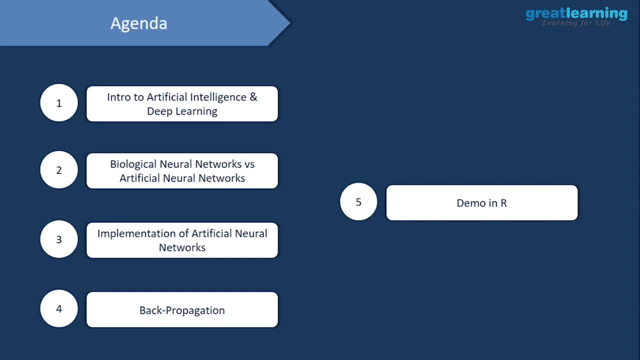 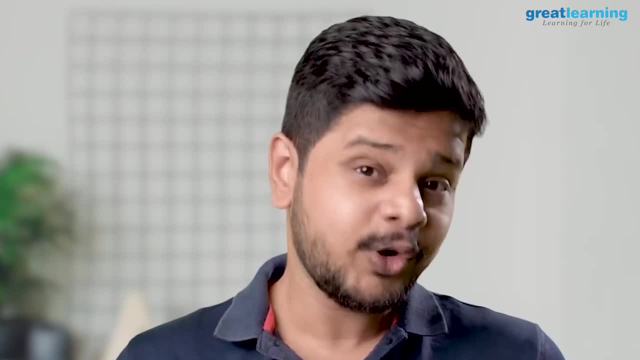 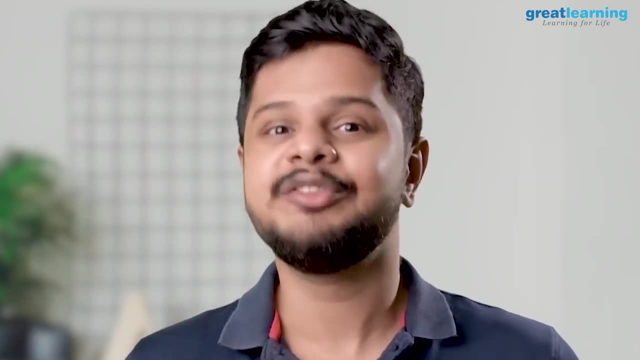 artificial neural networks, So let's get started. networks with the r language. so let's start off in this session. in this video, we will see what is artificial intelligence, what does it mean, how it has evolved over a period of time, and what does it mean to you and me and what does it hold for us in the future. artificial intelligence has been. 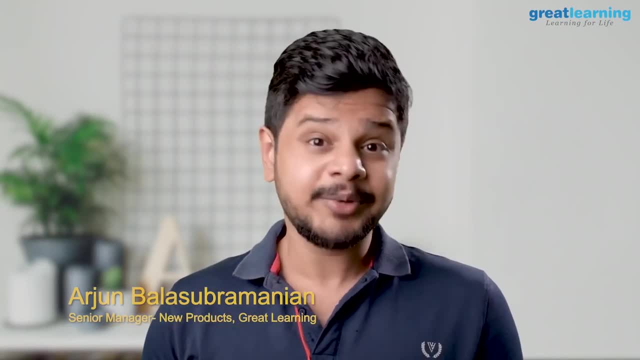 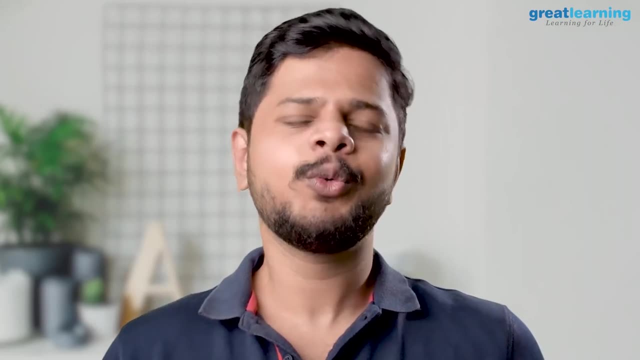 gaining a huge momentum in the recent world and it's making a tremendous impact in our career outcomes. but before we delve into that, let's understand what is artificial intelligence. so what is ai? let me ask you a question. look at the photo above and can you guess who that famous? 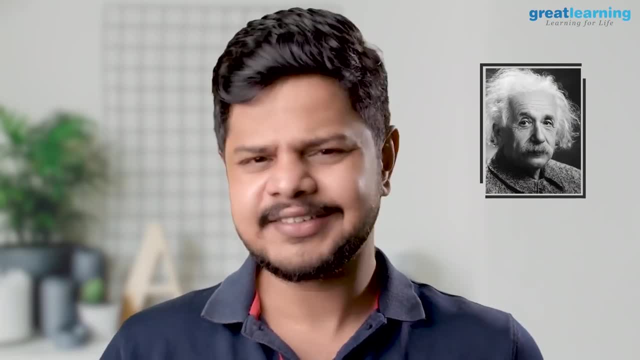 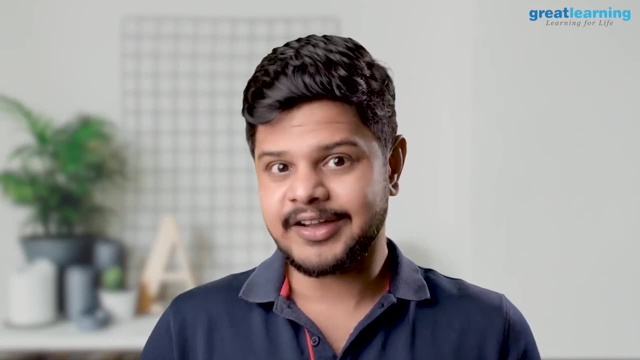 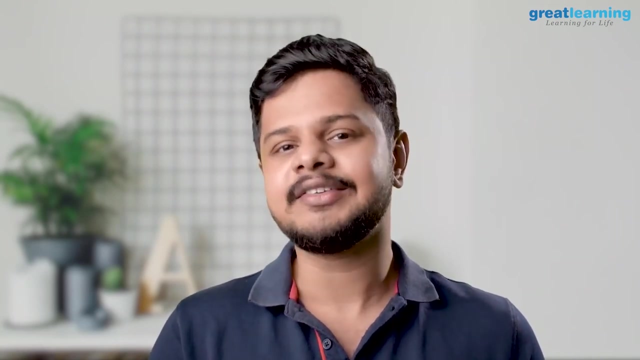 personality is. i think most of you guys would have guessed that it is albert einstein, but it's not an easy problem. think about how your brain processed that information and how did it recognize it. it might have noticed the facial features. it might have noticed the curly hairs. it might have noticed the distance between the eyes. it might have noticed 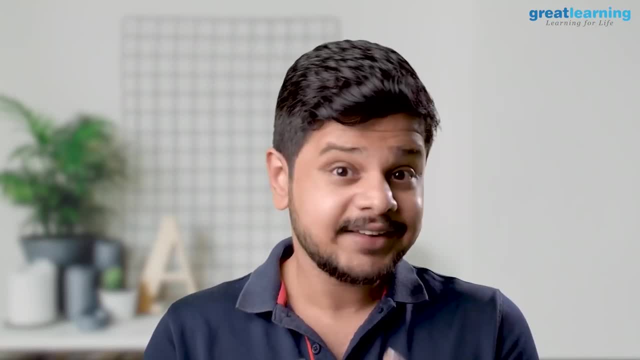 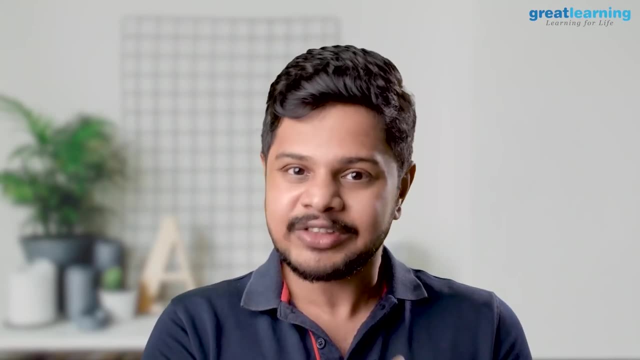 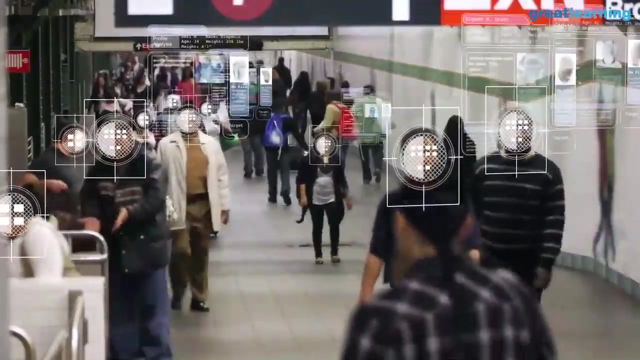 another million features to come to the conclusion that it is albert instant. so can you make a mission to think the same way which you think? that's ai. the process of making a mission to think like how a human does is what is known as ai. however, humans ability to think and 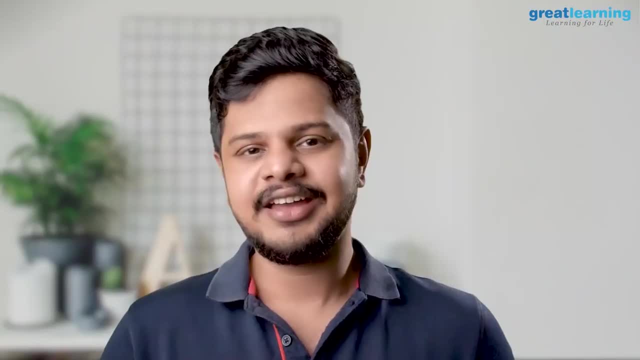 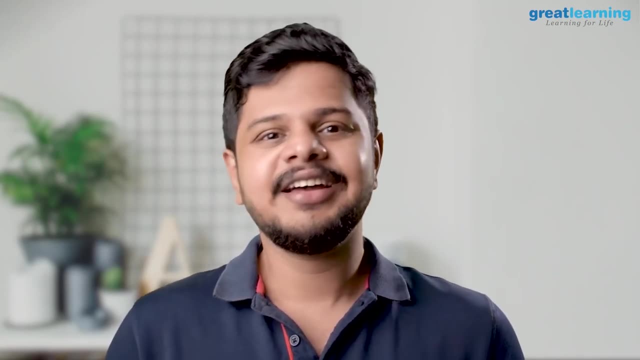 make a rational decision in a critical situation is unparalleled, and even science is not able to crack that. so what does machines have for them? how is it superior and how is it doing good? what do they do in terms of the ability to think? what is the power of a computer and what are the 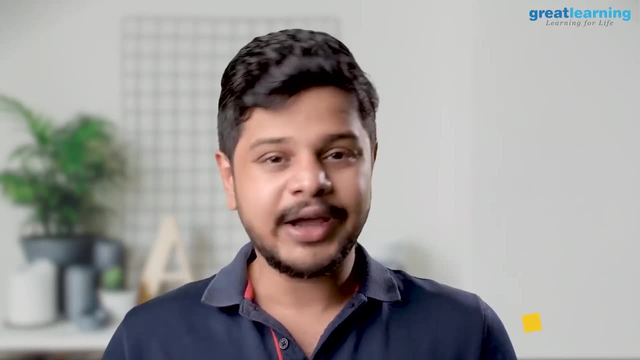 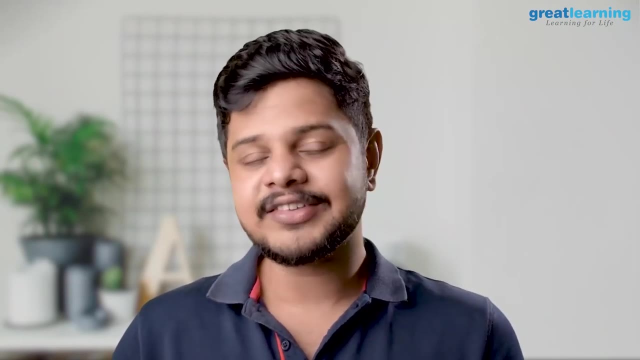 uses of the computer, the way it has been developed and the way it has been played in the world. there is no computational power, and this has gone massively in the recent years. let me ask you: what is the square root of 200? you'll not be able to tell me in a second. but whereas the computers 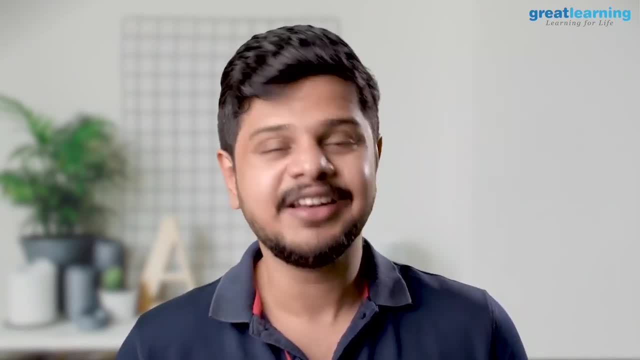 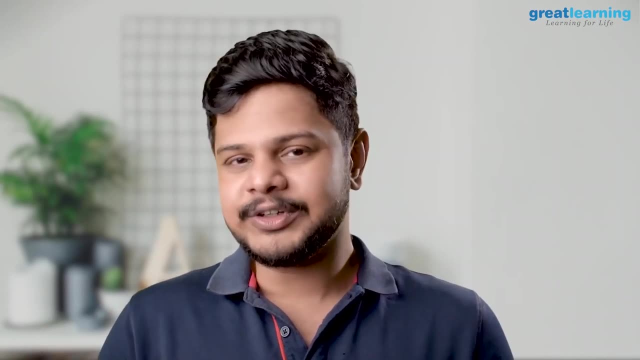 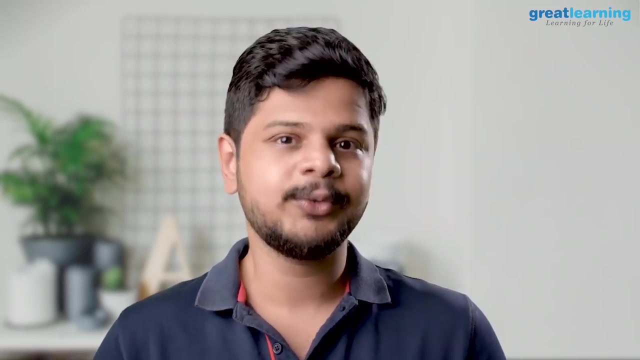 can. but if you were to ask a computer to take a bottle of water from your kitchen, will it be able to? well, the computer needs to know what does a bottle mean, what does water mean, and how to move computer to learn about its surroundings, adapt and then grow. yes, also, yeah, the term artificial. 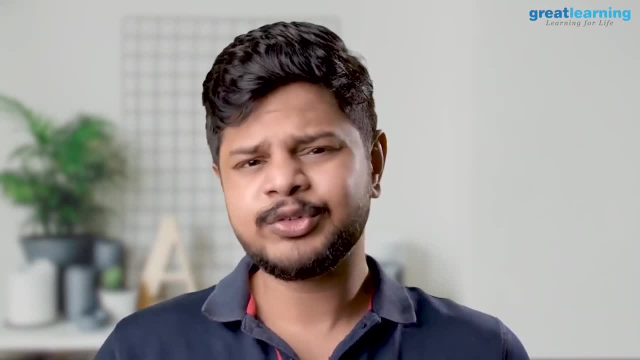 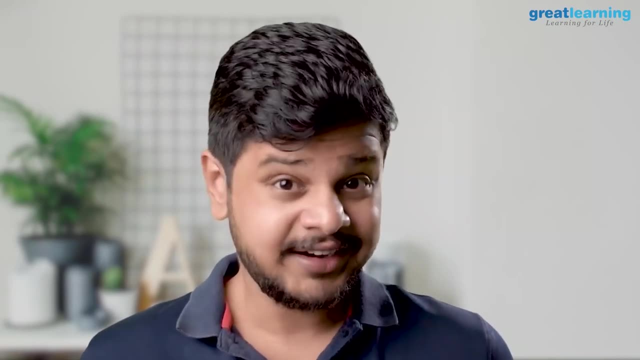 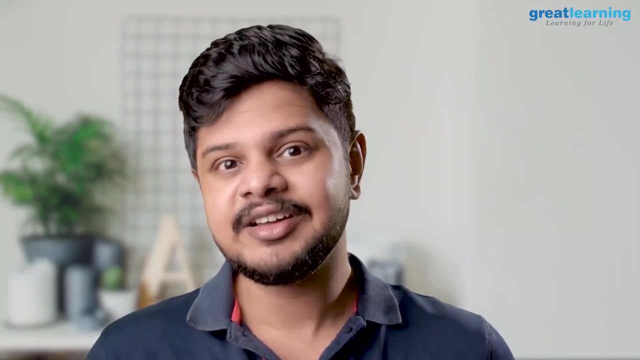 intelligence has been around since a long time. it was first coined in 1956 by mr john mccarthy at the darpa conference. though the conference was a hit and it garnished a lot of attention from a lot of players while creating these machines or creating the smart machines required. 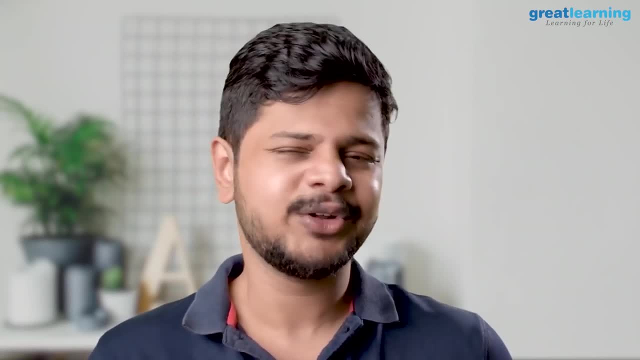 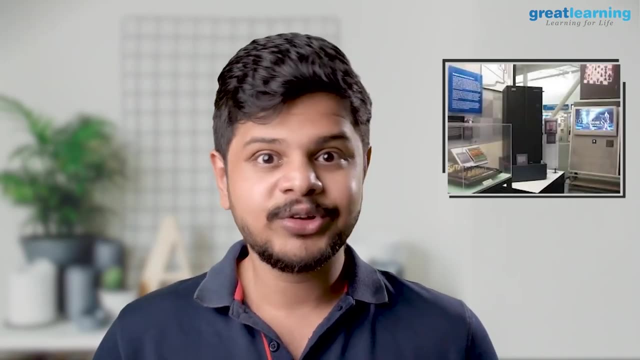 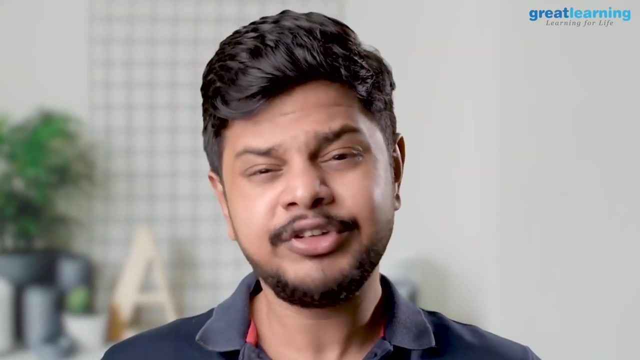 a lot of computational power and hardware, which was apparently not there at that point of time. well, the tipping point came in the late 90s, where ibm's deep blue stunned the entire world by defeating the world champion at a chess tournament, though not a fully functional ai. we 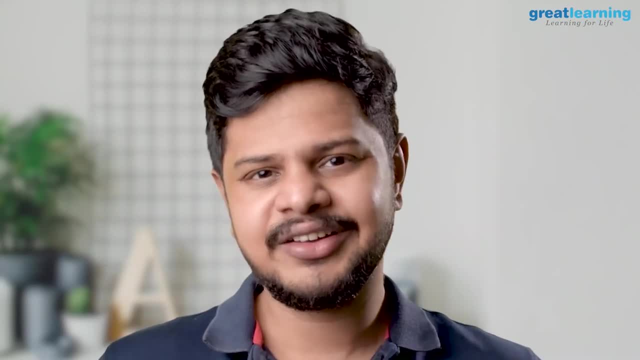 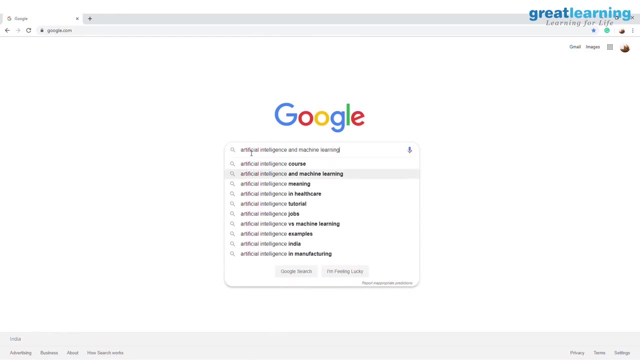 see fragments of ai implementation in our daily, day-to-day life. think of the next time when you type in google to search something, well, how does it come up with the fact? what are you going to type next? well, google has tons of data based upon what have you typed so far, and its ai algorithms are running. 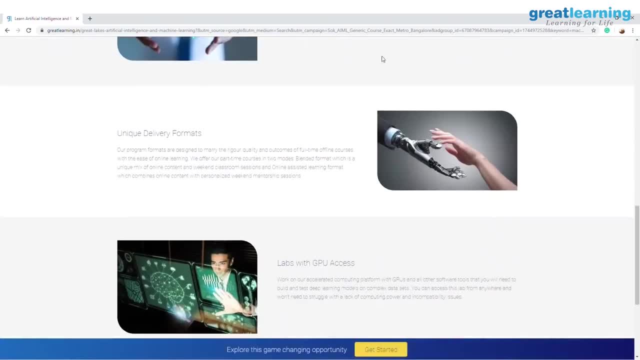 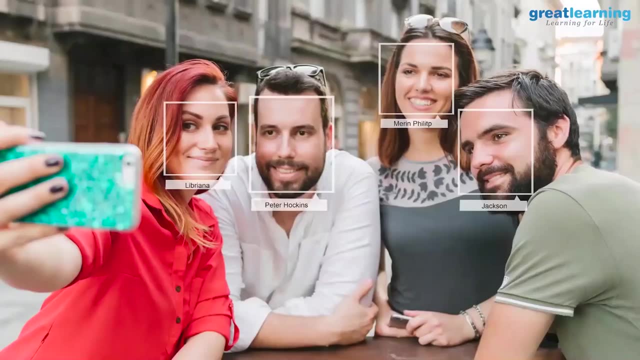 on the back to find out what are you going to type next based upon what have you typed. netflix predicts what movies you want to watch next based upon what movies you have watched in the past, whereas facebook detects all your friends in the same photo which you have taken and uploaded based. 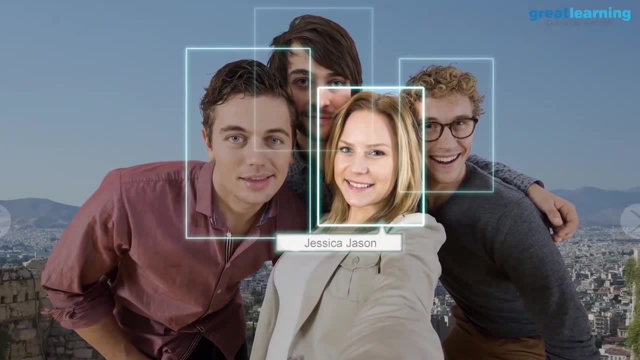 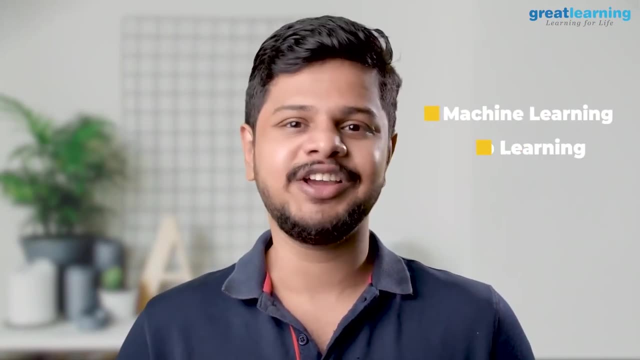 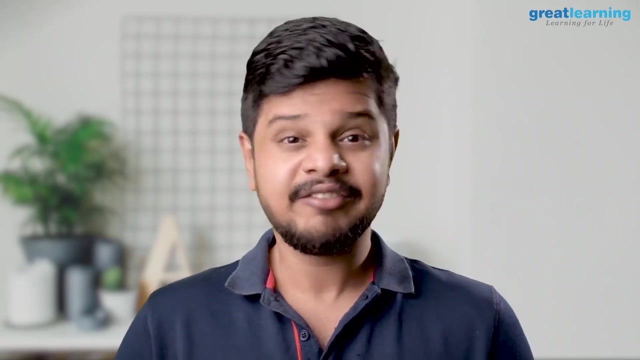 upon the information it has gathered in the past about your friends. in your own profile, ai, is you divided into two broader categories: machine learning and deep learning. machine learning is the use of statistical methods to understand and analyze information from a given data, whereas deep learning a broader area of machine learning or a broader subset of machine learning. 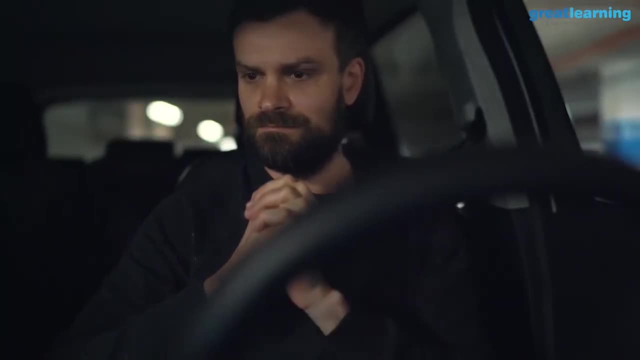 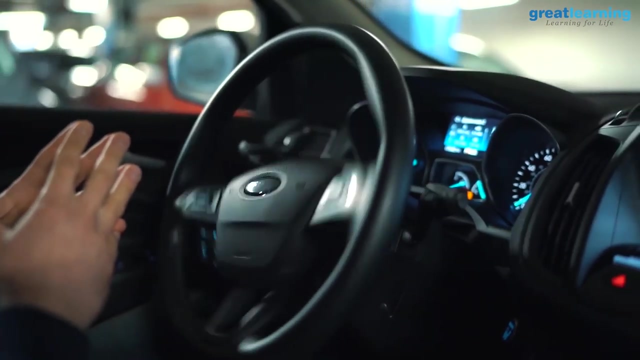 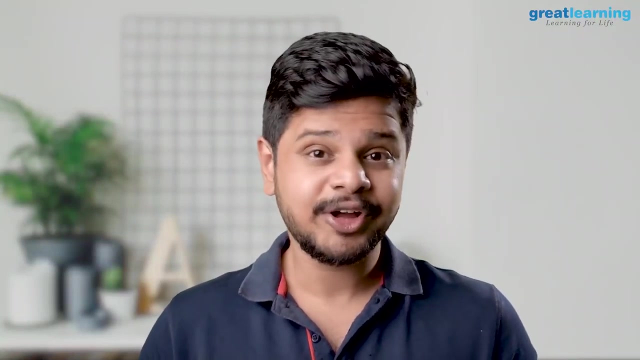 mostly deals with neural networks. with computational power growing exponentially year on year, the scope of ai has become vast and is being used in almost all the domains, in all the verticals and across all the industries, be it it retail, telecom, bfsi, travel, e-commerce. any of these industries, ai and ml, has a future in all. 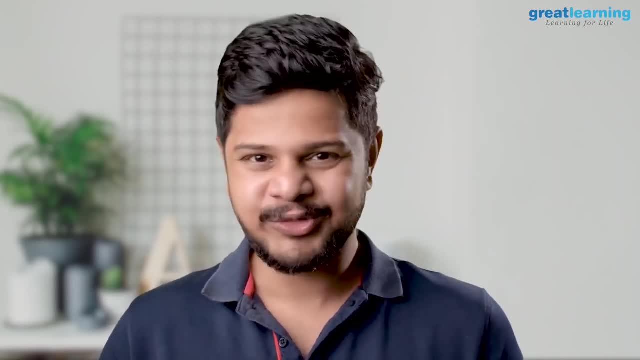 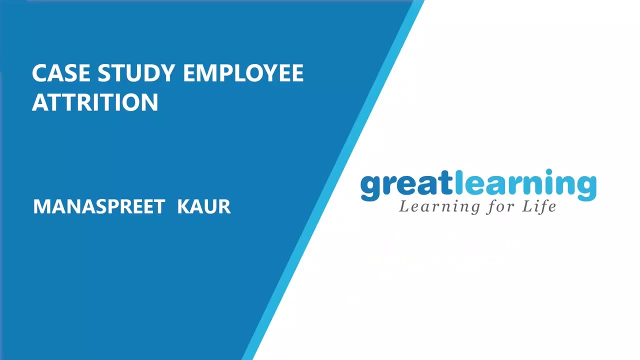 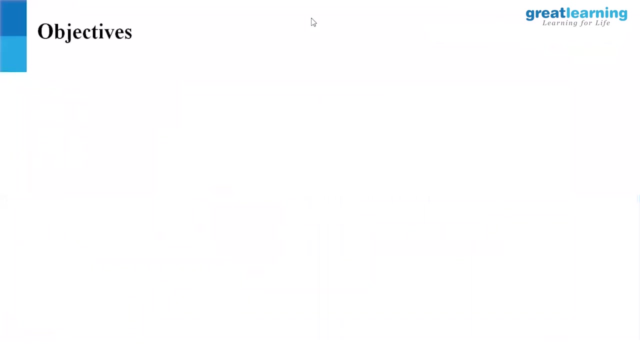 the facets of these industries. hope this video was helpful to you guys. if you like this video, like, share and subscribe to our channel and stay connected with us for future updates. so with neural networks, uh, we'll start off with um, seeing briefly what a biological neural network is. um, we won't go. 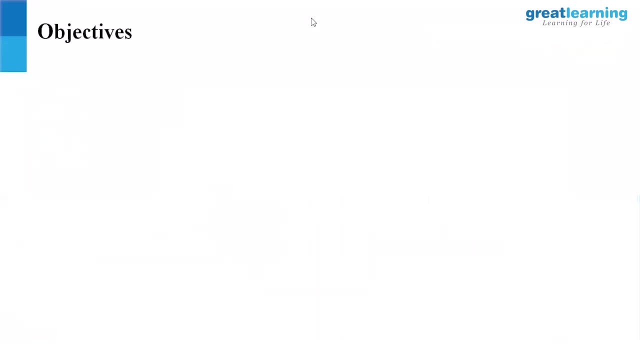 into much of the details. we'll just do an overview, because it helps to understand what an artificial neural network does. um, then we'll see the overview of artificial neural network and a small example- a pretty small example- on what happens and how a neural network learns. we'll see how we implement. 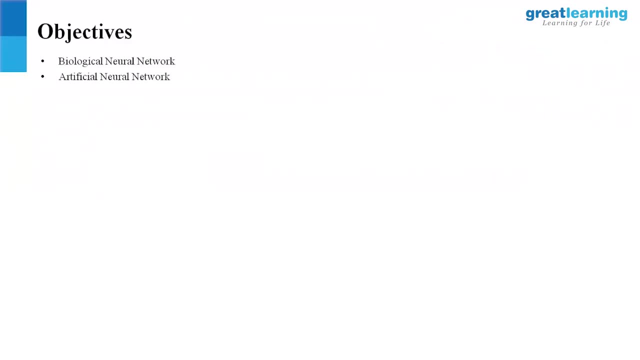 a, an and and um different steps that are a part of implementing artificial neural network, one of them being backpropagation, then the weight subtation and then the error function. Then we'll also see the summary of what the overall learning algorithm that the neural network follows. 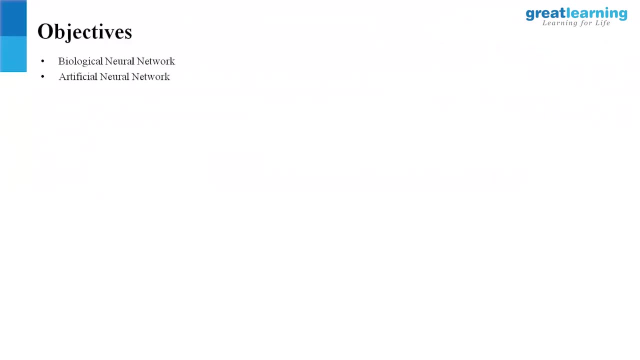 And then we'll see how we implement neural network in R using that same iris data set that we used to do, so that we only know what is the essence of using neural network in R And we're able to compare the outputs of what we did with previous algorithms and what the neural network gives us. 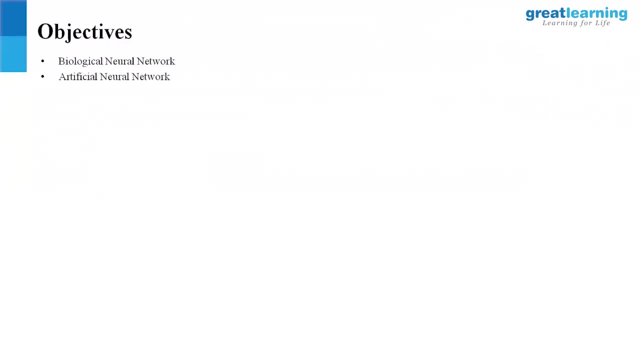 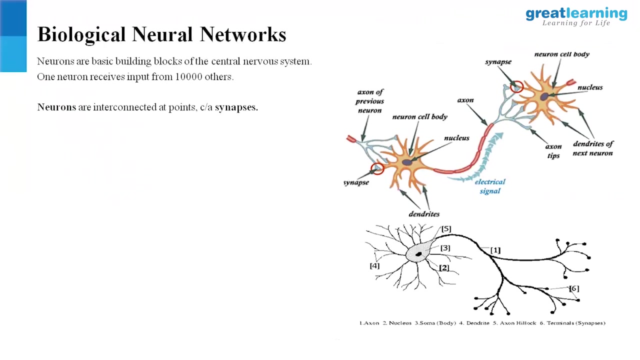 Okay, So with biological neural networks, you would have seen already how they're the basic building blocks of the central nervous system. So these are the diagrams, which may be repetitive for you, but then they help us understand what a biological neural network does. 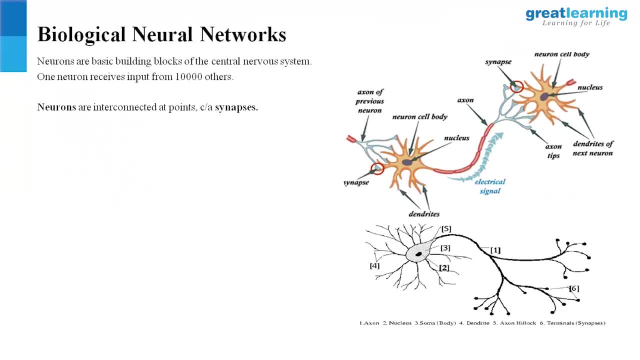 So not Going very deep into biology. So something that you see in yellow is a neuron which is similar to a neuron in the artificial neural network, wherein each contains some data about the input data variables. Okay, So like the neurons are interconnected at the point called synapses. 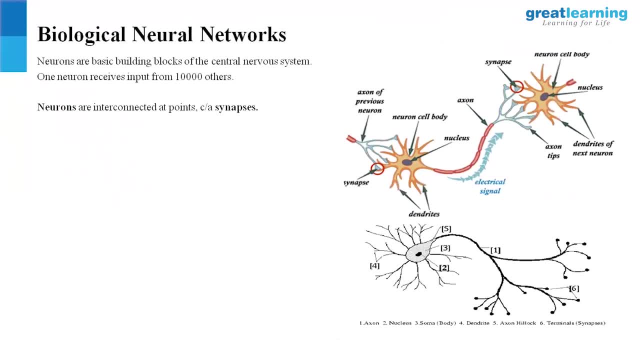 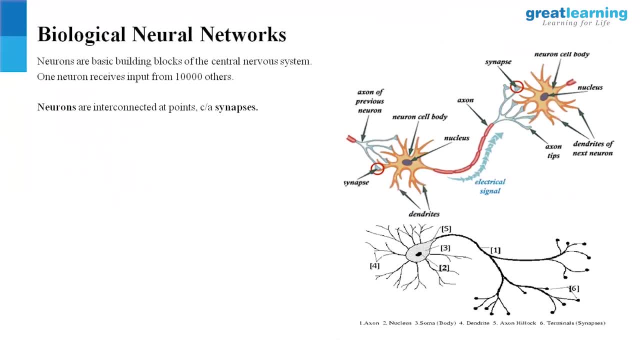 And this is similar to the artificial neural network because the different input variables that you take- that information is passed through the hidden layer. And how that information is passed through the hidden layers is through a point which is similar to the synapse in the biological neural network. 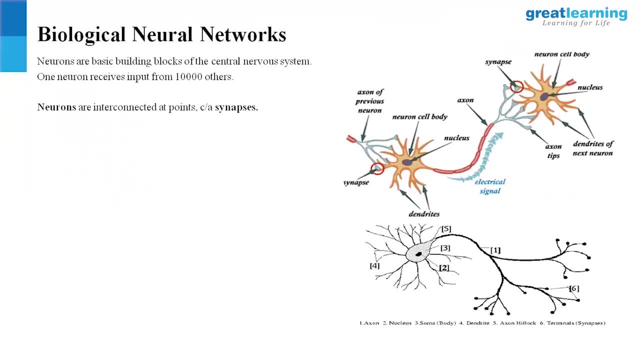 So there are three paths that are typically passes through the synapse, And the biological neural network has three or four paths that we typically choose to use. wed Kalau are typically present in the biological neural network. one is the dendrite, which is the yellow. 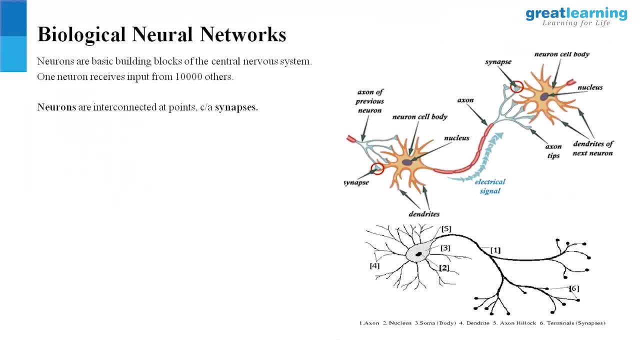 you can say like terminals of a neural network which are responsible to receive signals from the surrounding neurons. then there are accents which are nothing like a path. so comparing it to the artificial neural network like there is a path when you go from the input layer to the hidden. 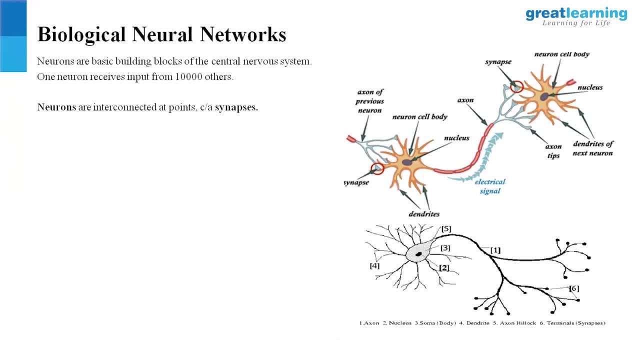 layer. there is a path in between which carries the information, so the action is similar to that. then the synopsis synapses are responsible for receiving the signals and learning from the past activities. how we correlate it to the artificial neural network is because, if you, if you know of the concept of back propagation, even the artificial neural network, 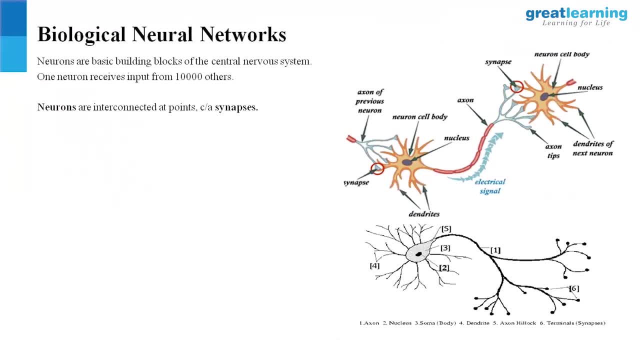 learns from its past activities. hence you're able to relate the biological neural network with the artificial neural network. so each of the neurons here act as a neuron in the artificial neural network. the axons act as a path where the information is traversed from one layer of neural network to the another layer of the neural network. 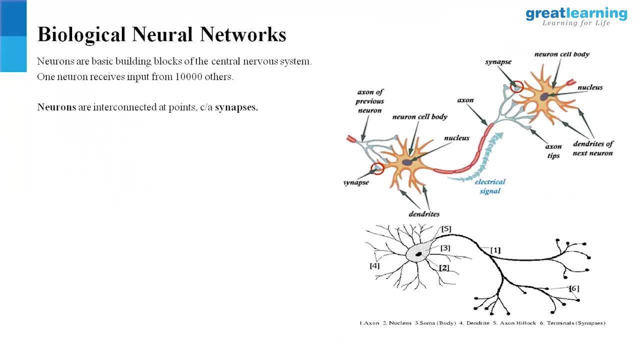 and the dendrite and synapses are used to send and receive information between one neuron to the other, and then they also enable the neural network learn from the past activities, and that's how the algorithm improves itself. okay, so this is essential to understand. only because the artificial neural 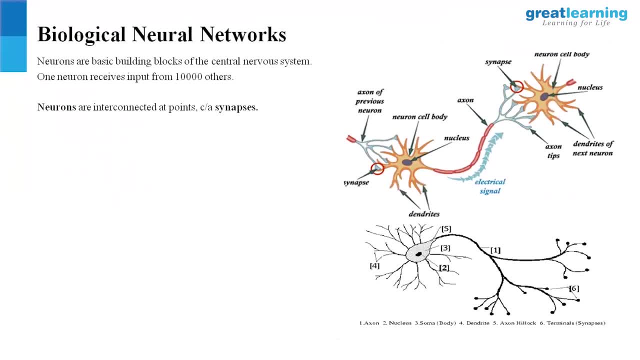 network gets its name from the biological neural network only. okay, so this is again a small diagram to just show you how the information is passed with the biological neural network, and a similar kind of thing happens with the artificial neural network as well. okay, so what happens is whenever a 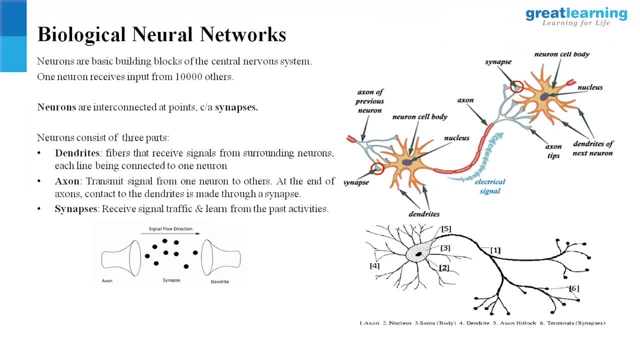 certain information is coming to a neuron when a certain information is present in a neuron. so there's this thing called threshold, which we are also seen with the artificial neural network. so once that threshold is reached, threshold has been achieved. the neural network transmits a signal through the axon and the similar kind. 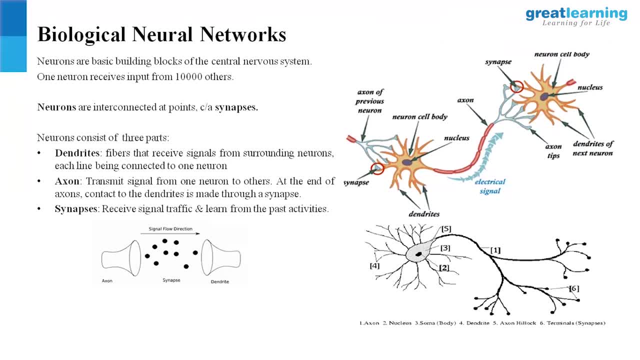 of thing happens with the artificial neural network as well. whenever the threshold is reached, activation function triggers and then an information is passed from the input layer to the output layer. so we'll see how each of these steps in the biological neural network helps us also understand what is present in the artificial neural network. okay, so this is. 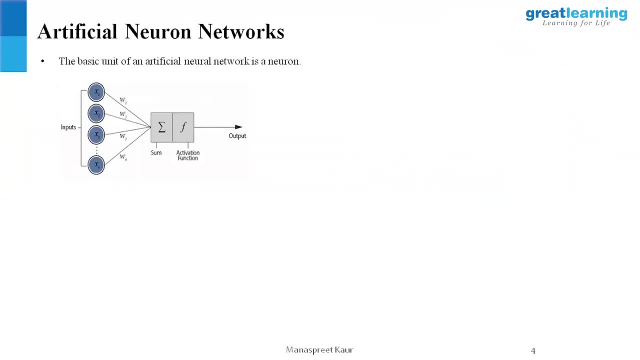 how a basic of how an artificial neural network works. so the inputs that you see here are nothing but the input data variables with the data set they are working with. then there are certain weights which are applied to each of the input variables. so the weights that are applied are: 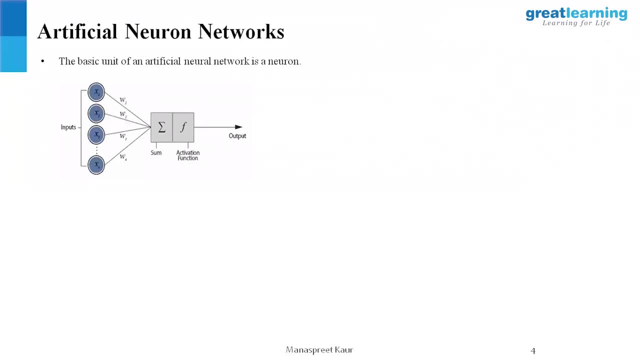 say the num and k. tweeter thefte instánt to escribes kt and the number of 좁. who is the Autobot? the slow movement to the other end of the variable entre Ferrari is called the zoom. while I am showing, you are told at which input I am going to use this verb. 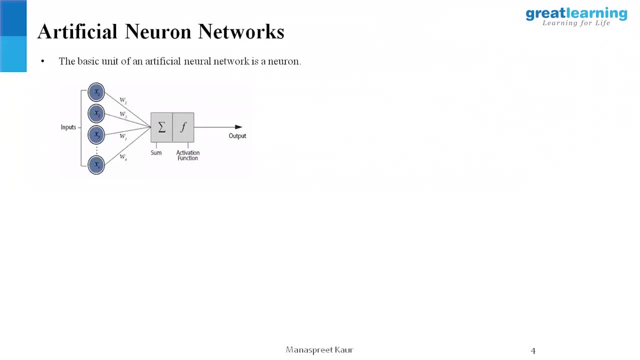 which is still positive, because even though they are using trenches for the�� disappeared- and they are- is through these weights. So whichever variable is given a higher weight is comparatively more important than a variable which has a lesser weight. So this is how the weights are used in. 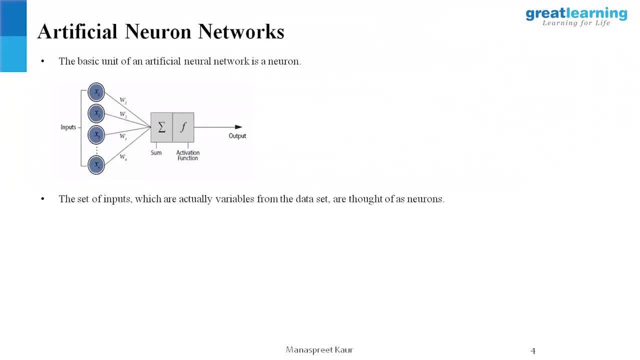 a neural network. So the set of inputs, which are nothing but the variables from the data set, are thought of as neurons. This is how we correlate an artificial neural network with a biological neural network. So then they are weighed according to the weights that are applied. what I just told. 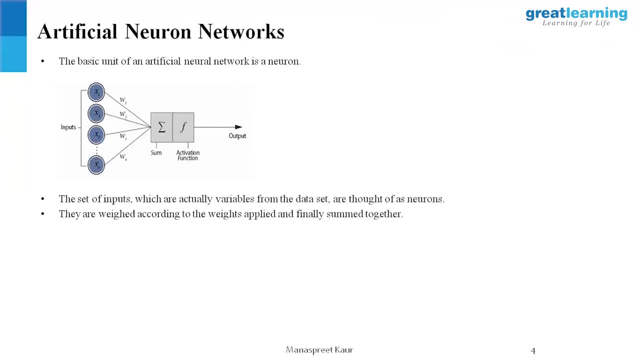 and finally, this is we do kind of a sum product of the input variables with the weights. Subproduct means to say x1 into w1, plus x2 into w2, plus x3 into w3 and so on. Okay, so the function that you 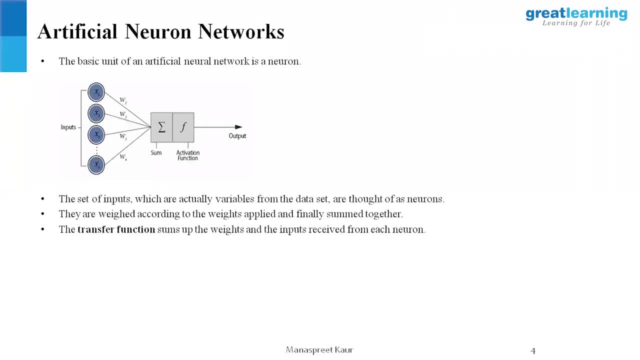 see here the summation function or the sigma function. here this can also be called as a transfer function. So this actually performs the sum product, So it will sum up the weights and the input that it receives from each of the neurons. The next step is to go to the activation function, which will decide. 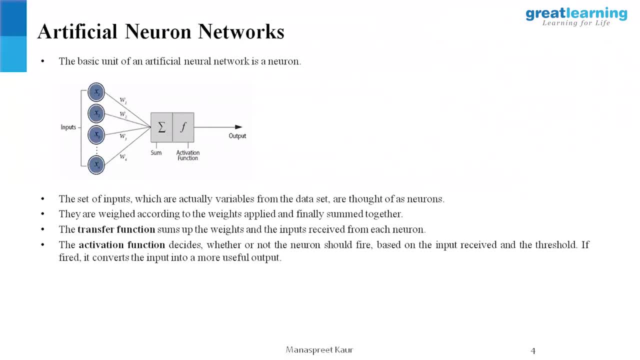 whether or not a neuron will fire. So this is similar to the biological neural network wherein with the threshold we decide whether or not the information should be sent to the next layer. Okay, so if the threshold, so whatever sum you get using the transfer function, you compare it to the 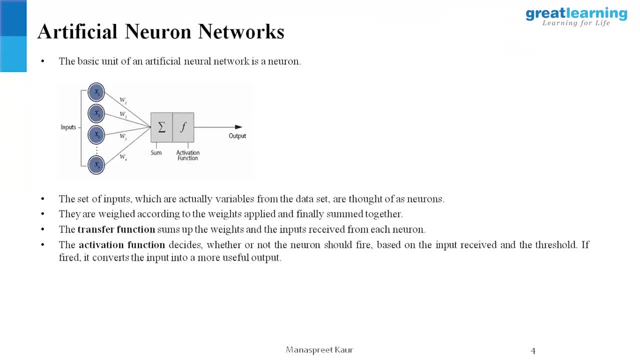 threshold. if it exceeds the threshold, the activation function decides to fire. when it fires, the information is passed from the input layer to the output layer, like similar to what happens in the biological neural network. when the activation function fires, information is passed from one layer to the other. So this is the transformation function. So this is the transformation function. 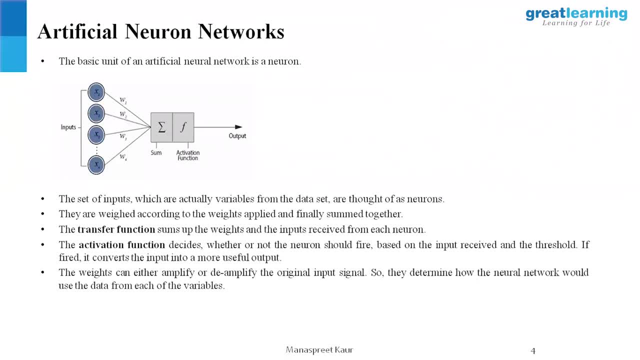 Okay so, like I told earlier also, the weights can be used to amplify or de-amplify the original input signal, meaning to say they are used to determine how each variable will be used. what is the importance that will be given to each of the variables? Okay, so consider a simple example. so, 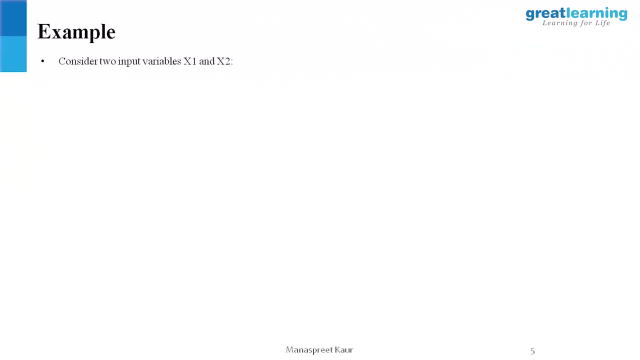 this example has got nothing to do with the neural networks. actually, Consider that you have, just say, two input variables and you have two input variables. So you have two input variables and you have two input variables. This variable is called x1 and x2.. 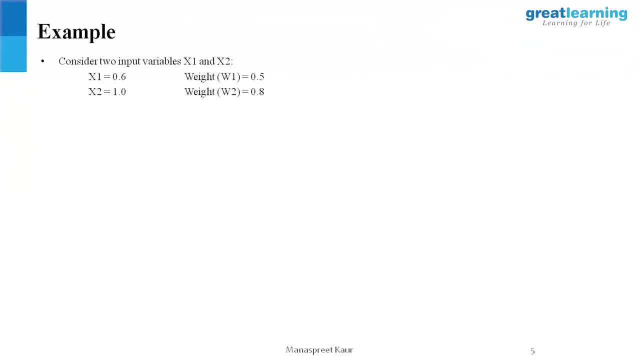 So these are two input variables in a data set, one of them having, a way, a value of 0.6 and one of them having a value of one, and the weights say that are applied to both of these input variables. Al annoyed of value of 1.. And the weights say that are applied to both of these input variables. Al struggled. 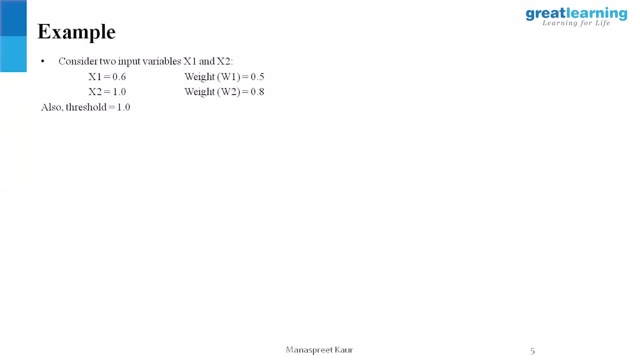 are given a threshold of one. So what happens In simple terms? the neural network is the first term- is given the value of 1.. of a transfer function, what we saw in the previous slide. So nothing but a sum product will happen here. So 0.6 into 0.5 plus 1 into 0.8.. So that gives you a 1.1.. So this is similar. 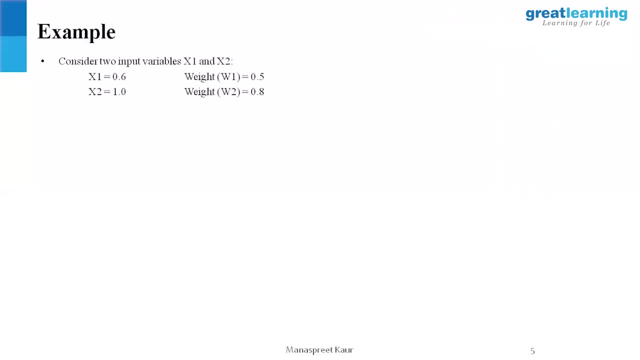 to the summation function that we had seen here. Next, we compare this value that we've got with threshold. So say, our value that we've got is 1.1, but the threshold is 1.0. So we see that our 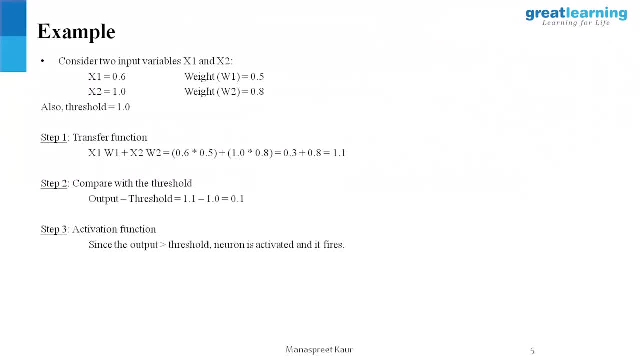 output is more than the threshold that was allowed. So since the output is greater than the threshold, so the neuron is activated and it fires. So this is a very simple example. This is not what actually happens in the neural network, because they're a derivative of the error function and 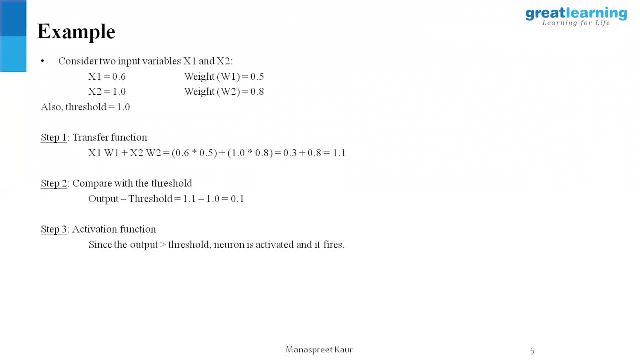 all that is calculated. So error function is nothing but the actual output, a difference between the actual output and the desired output. So therein a derivative of that is calculated and passed back to the neural network. But I put this example only to show you how the threshold works. So when, whenever the output exceeds the threshold, the neural 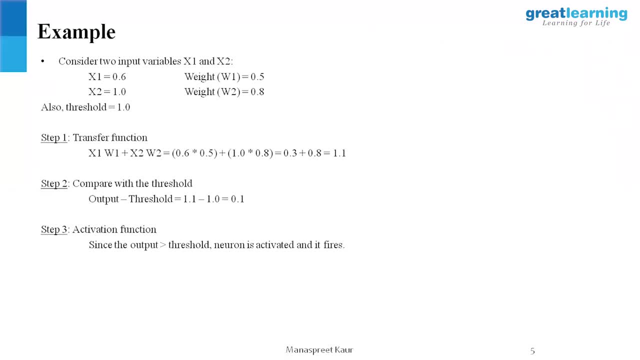 network fails, So the neural network will know that it needs to fire the signal. What is meant by firing a signal is nothing but a back propagation, meaning to say that whenever an output increases the threshold, the algorithm will sorry. whenever the output increases the threshold, a back propagation will occur and a reiteration will occur, a new iteration within the network. 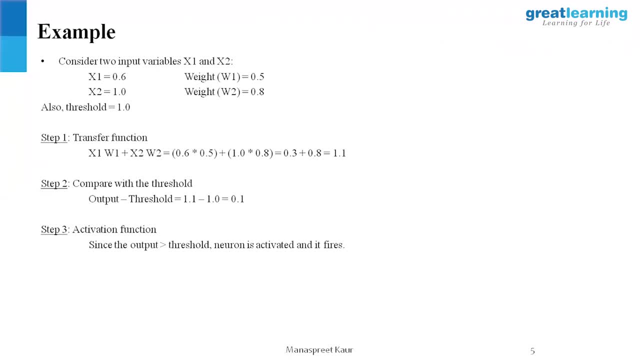 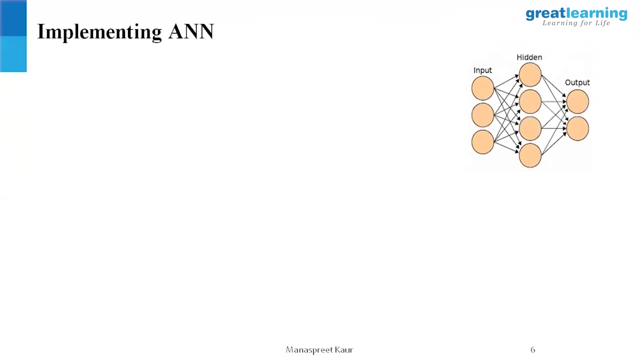 The neural network will occur. and the output? the algorithm will try to improve the output. Okay, Now we'll see how we implement the artificial neural network. So this is a simple diagram to show how a neural network works. So there are, for example, three input variables and two output variables here. 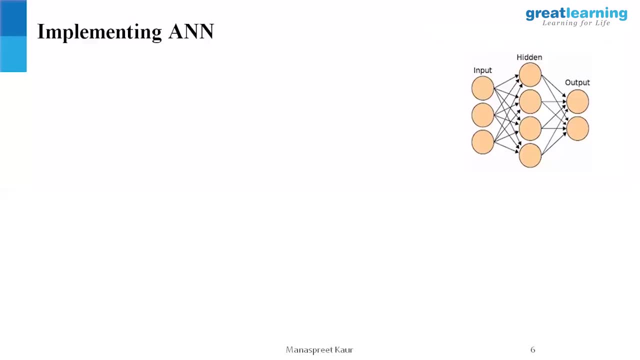 So they can be any number of hidden layers that are present. So there are, for example, three input variables and two output variables here, So they can be any number of hidden layers that are present. So there are, for example, three input variables and two output variables that are present. 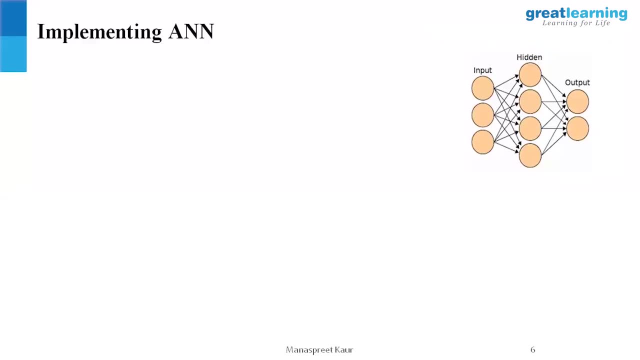 In the neural network and the hidden layers actually perform. whatever The algorithm needs to be applied is done by the hidden layers only. There are different ways on how we decide how many hidden layers are to be present, And we'll see that when we work with R. 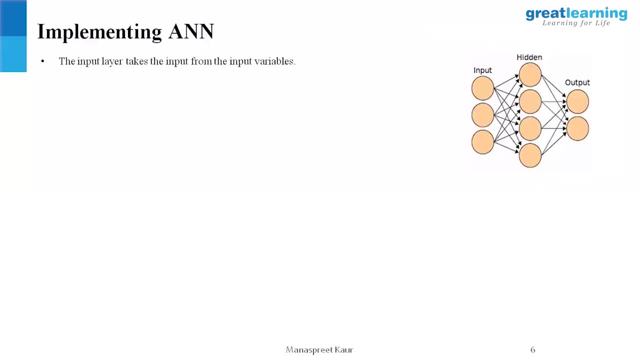 So what happens here is that the input layer will take the input from the input layer, the input from the input variables. so say you have three variables here, so each input, each of the neuron that you see in the input layer, will have data from one variable each. the input layer will take input from the input variables. 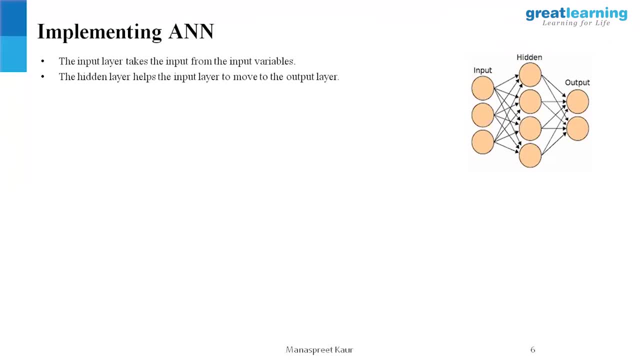 the in hidden layer will help the input layer to move to the output layer. okay, so the input layer will pass the information to the hidden layer with the weights present and then the hidden layer will move that data to the output layer. but the hidden layer is essentially a big black box layer like I. 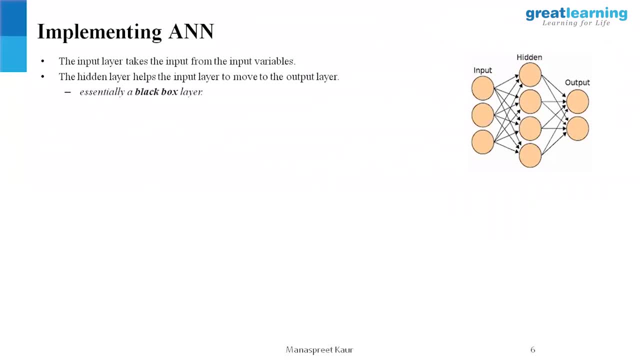 told you earlier, you will never be able to understand what is happening with the hidden layer, and the output layer will throw you the final output. so this is another the way to a more detailed diagram of the above diagram. so what I'm trying to show here is that 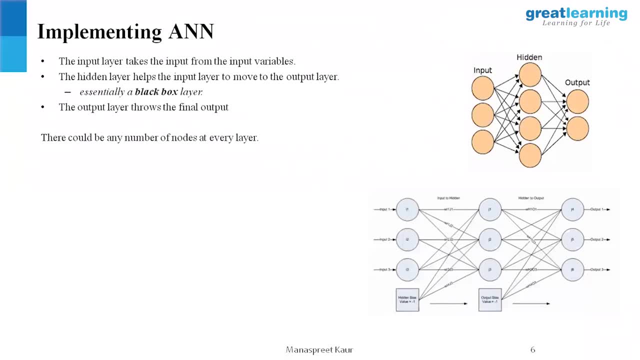 there could be any number of nodes that one can be present at every layer. and then there are weights that are applied to the inputs. excuse me, okay. so then there are weights that are applied to the inputs that take them to the hidden layer. so if you see in the diagram below there are three. 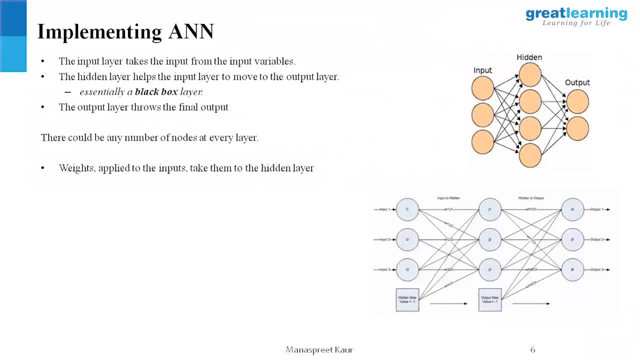 inputs- one, two, three- and then there are some weights which are applied to the each of the inputs when it is being taken to the hidden layer. so each input variable with some weight applied will go to each neuron in the hidden layer. so if there are three input variables and there are, 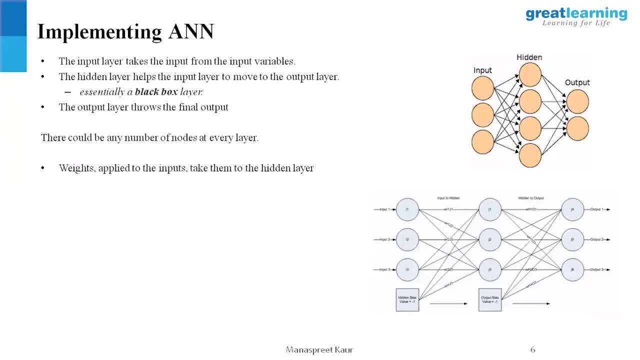 three hidden layers. so each of the inputs, like the input i1, will go to each of the the neuron in the hidden layer and a different weight will be applied when it goes through each of the neuron in the hidden layer. and there is another category of weight, so one is the weights. 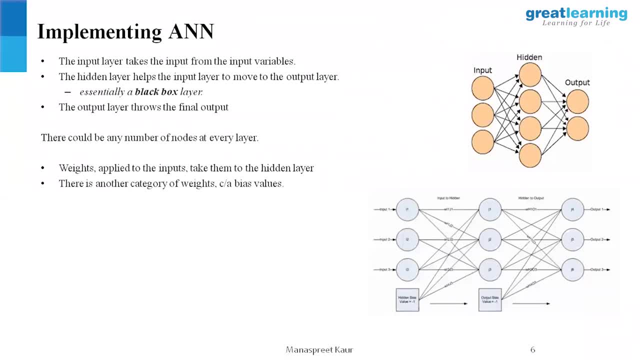 that are applied to the input variables. there is another category of weight, which we call as the bias values. so bias values are again used to train the neural network. so this, this can be compared to, if you remember, with regression also, we used to have a similar thing, wherein we'll have some 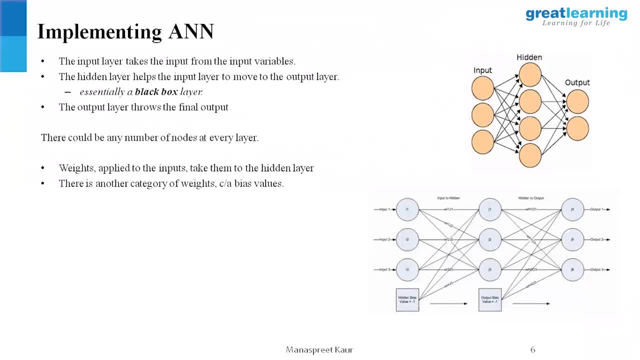 weights that are assigned to each of the variables. so that were the coefficients back in regression when you used to get an equation something like: y equals to a plus b1, x1 plus b2, x2 plus b3, x3 and so on. so when there were coefficients in regression are the weights which are in the neural network. 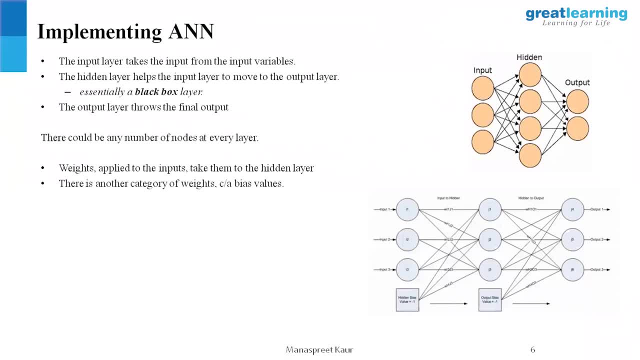 but they were. so there was also an intercept, which was the unexplained variance or unexplained output that the intercept used to capture. so similar happens here with the hidden bias. so there is some information that the input layer, input variables, along with the weights, cannot capture. that is. 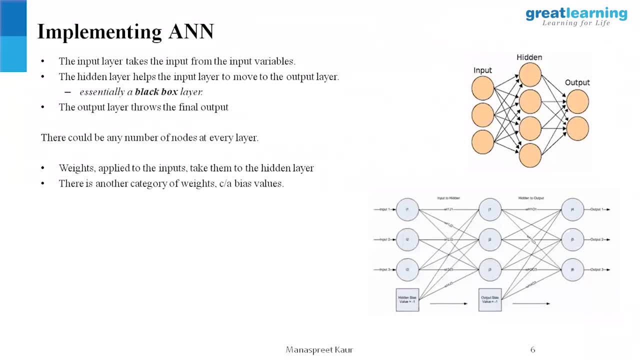 captured by the hidden bias. so with each of the layer that you have, apart from the input layer, there will be a bias added, like if you see in the diagram here, with the second layer, that is, the hidden layer present in the between, there's a hidden bias that is added, and with each hidden layer that you 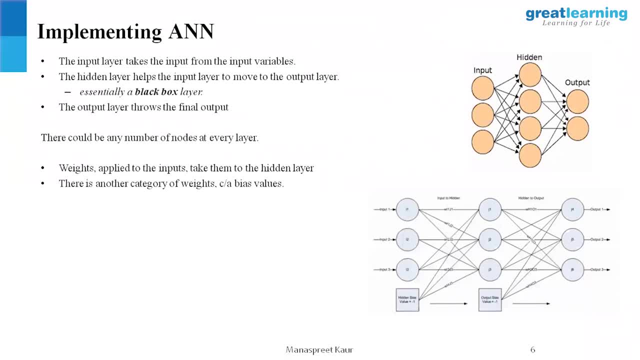 have like here. we have just hidden layer, but with each hidden layer that is present, there will be a hidden bias for each of the layers and finally they're all. there will also be an output bias, which is present for the output layer, nothing but the intercept, what we call the intercept layer. so 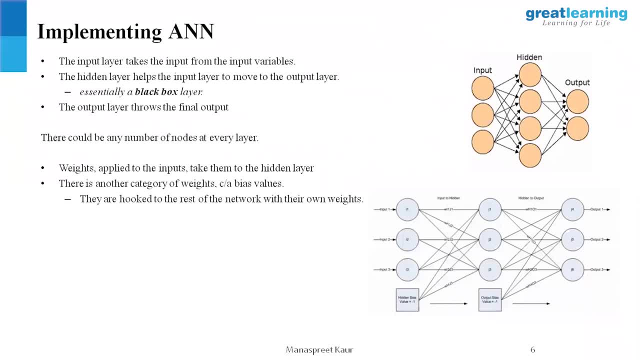 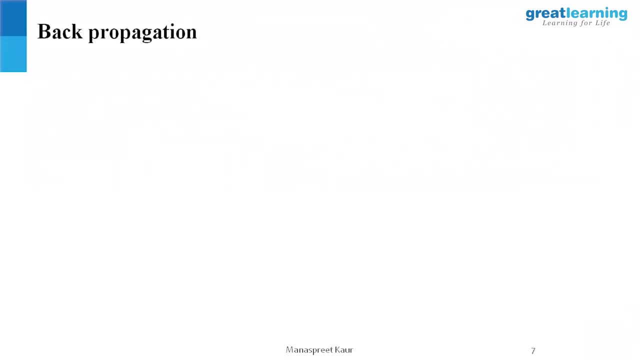 what we used to have with the regression equation. okay, that was the basic of what an artificial neural network does. we'll go to bragg propagation now to see how the neural network learns. okay, so the basis of a neural network is a powerful learning mechanism, although it is a powerful learning mechanism, but you will never be able to understand. 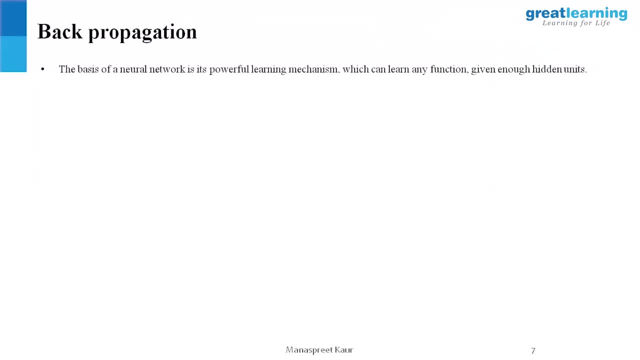 what that learning mechanism is. but, that being said, the neural network has a powerful learning mechanism and it can learn any function, given it has enough hidden units. so each of the hidden units that are present enable it to learn to the input data set, and how it learns is by the mechanism that we call. 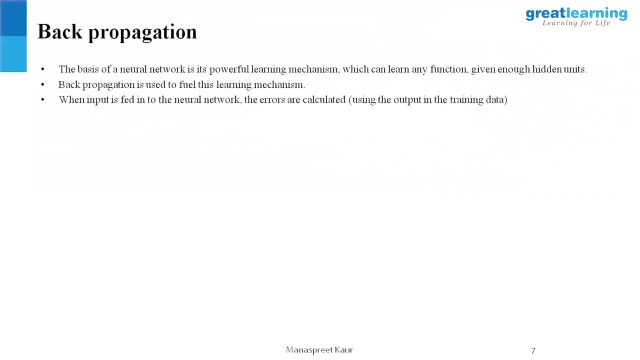 as back propagation. okay, so, like i told you earlier, also, when an input is fed to the neural network, that is, when the input variables are fed into the neural network, the input will, some weights will be applied to the input that is coming, some bias will be applied to the in addition to the input that is coming. and finally, 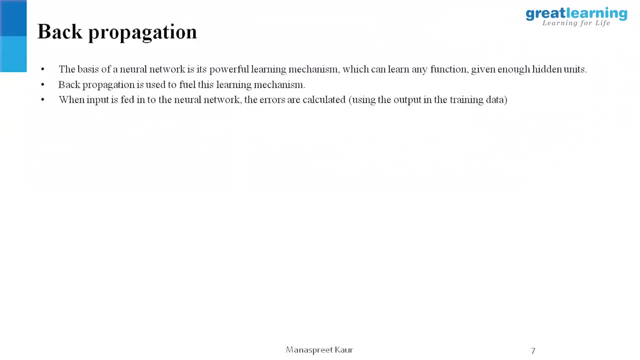 that data will go to the hidden layer. the same process will be repeated and the data will move to the output layer. when you get the data at the output layer, the difference between what the actual output or the desired output was and the output that you are getting- some error- will be. 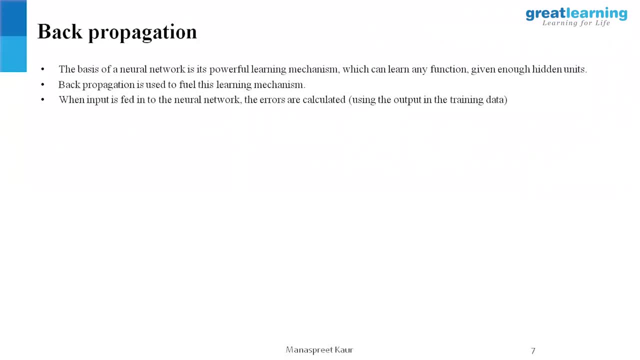 calculated based on the difference. whatever is, the error will be fed back to the first layer and the whole process repeats again. okay, so these errors are fed back to the neural network and then these weights to the question that you were asking. the weights are then changed in order to 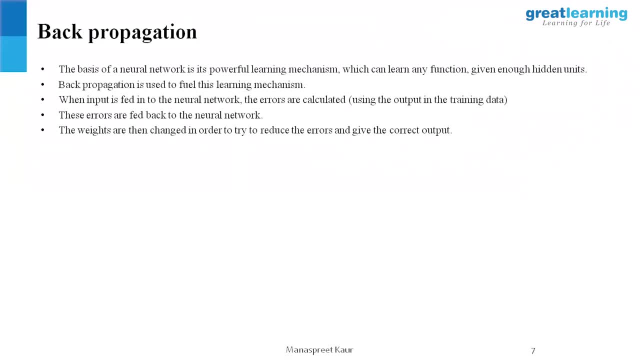 try to reduce the errors and give the correct output. so the first iteration, random weights will be assigned, but with each iteration that happens the weights are changed using the errors that we have got in the previous layer. so this is the diagram that explains back propagation. so there, 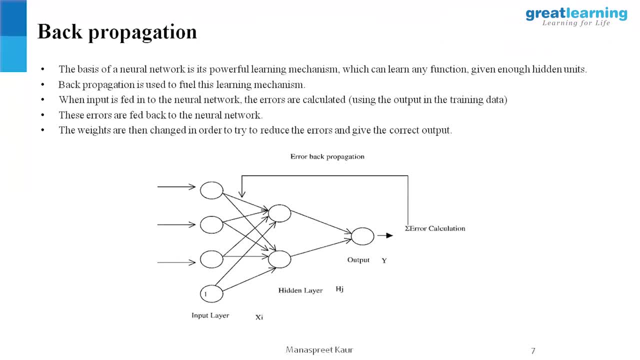 are some input variables, then there is a hidden layer- друзья, this is theад never transcendence attack variables. then there is a hidden layer. so say there are three input variables here. then there are two hidden neurons with the hidden layer. so each of the input variables is being fed to the 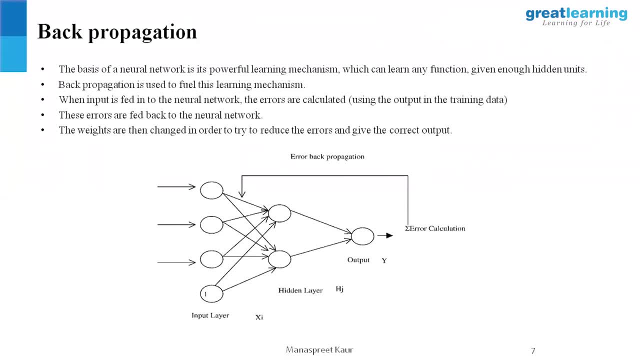 hidden layer, and then there's also a bias which is being applied, and then from the hidden layer we're going to the output layer. and the output layer, the error calculation happens, which is nothing but the difference between the actual value and the calculated value. whatever is the 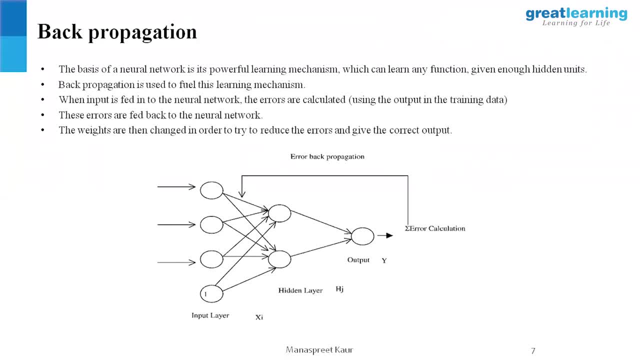 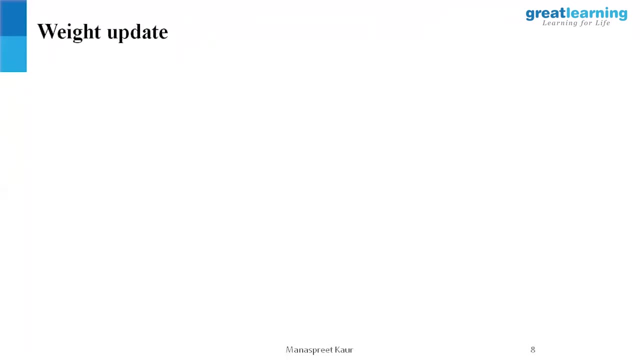 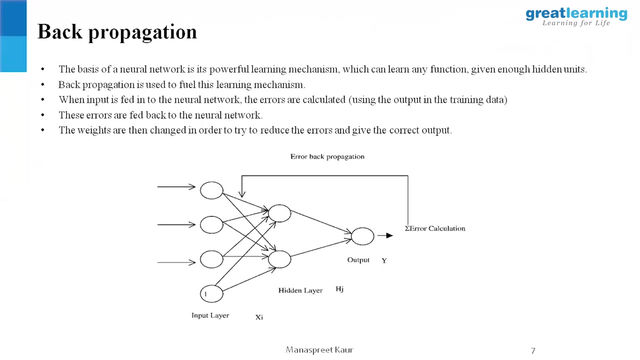 error calculation is back propagated and then the weights are modified. this happens each time the algorithm runs, and that's how the weights are improved, and that's how the algorithm learns, okay, okay, so then, once you're done with back propagation. so all you did with back propagation was to get the error calculation back propagated. so that's how the algorithm. 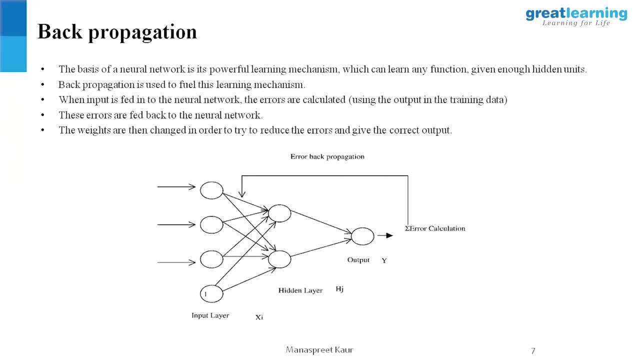 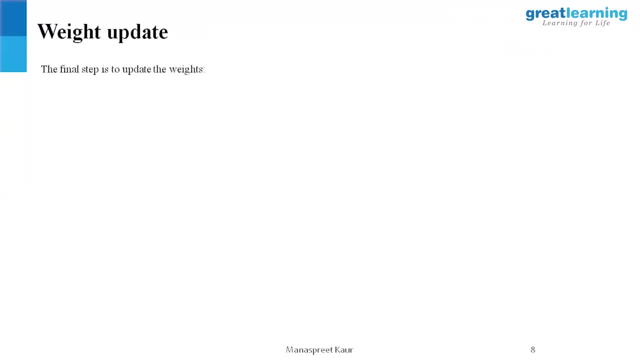 the error and pass it back to the input layer so that the weights are modified. now how the weights are modified is after you've done the back propagation. you need to update the weights now. if you remember with the previous slide that we've seen here, there are weights applied to the 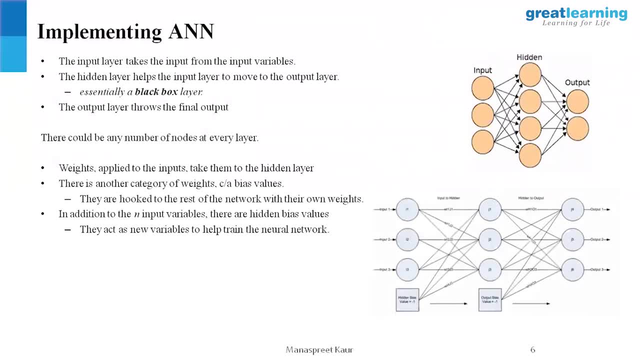 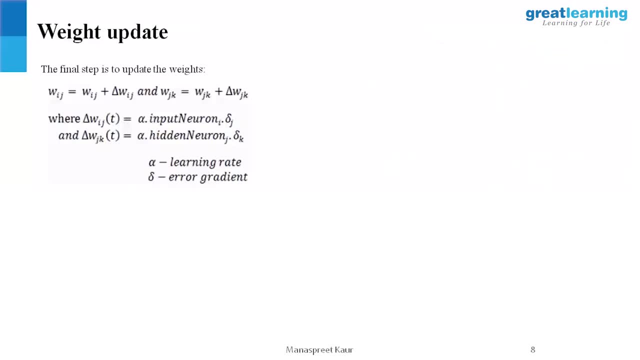 hidden layer, and then there are weights applied to the output layer as well, so both of these weights are applied to the input layer. okay, so don't get too confused with what the equation here is, but this is just meant to show that there are two different weights that are applied to both of 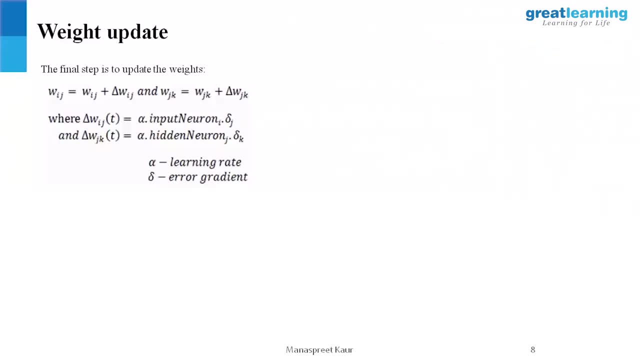 the layers. so w i j that you see here is the weight that is passed to the variables from the input layer, and w j, k is the weights that are applied to the neurons from the input layer. so both of these are the weights that are applied to the neurons from the hidden layer. okay, so both of 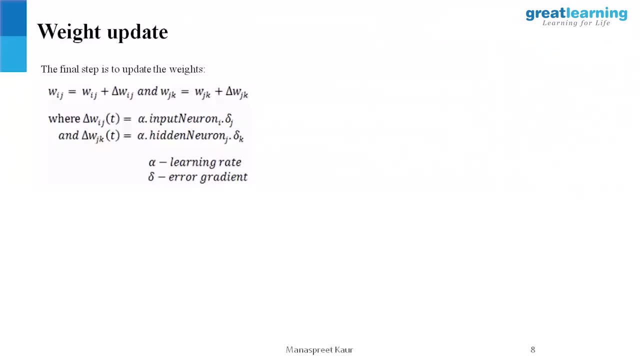 them will learn from the errors that they are doing, and both of the weights will be updated. now don't go very deep into what the mathematical terms here are, but this is just meant to tell you that both of the weights will be modified based on the error that we are seeing from the previous 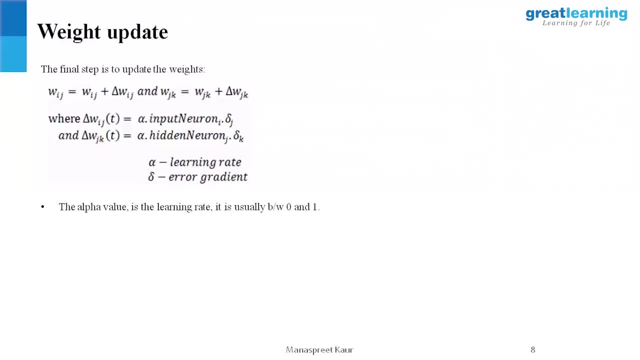 iteration of the algorithm. there's another thing which you would be see, uh, which you're seeing here, which is the alpha value. so alpha value is nothing but the learning rate. learning rate means to say at what rate do you want the neural network to learn? so this is nothing but the learning speed. 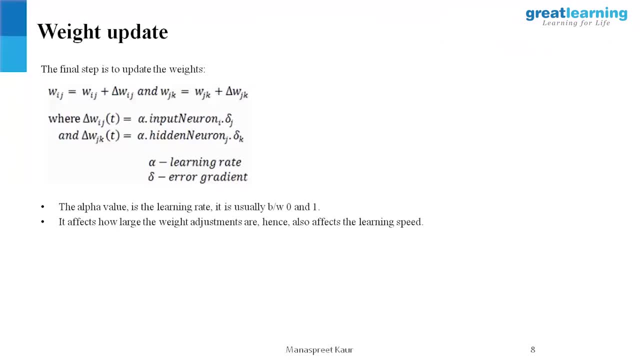 okay, if you make the learning speed too quickly or you make the alpha value, you don't really specify these values. this is what happens in the background. but if the learning speed is very quickly, the sorry. the learning speed is very fast at an alpha value is closer to one. 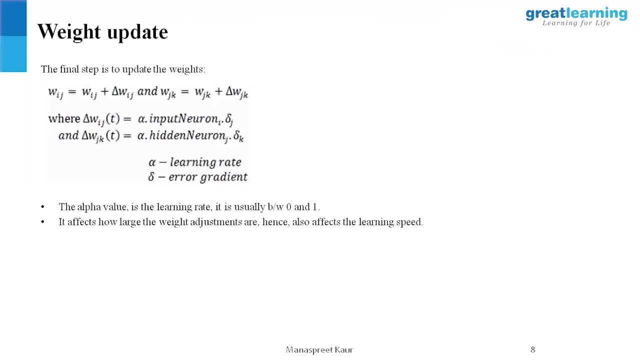 the algorithm would not be able to learn properly. this is nothing like nothing, but trying to say that you're trying to learn something very quickly, so you just run over it. you don't understand the essence of what was there in the data. and if, if you make the learning, 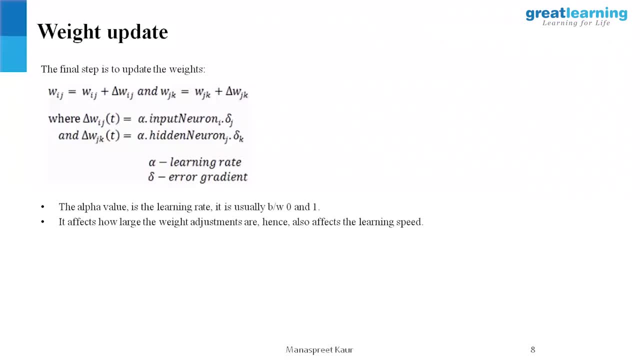 rate very small. you don't allow the algorithm to grow, you don't allow the algorithm to learn. only so an optimal learning rate is chosen. but you don't choose it. choose it, the algorithm chooses itself, but an optimal learning rate is chosen for each iteration that happens with the neural. 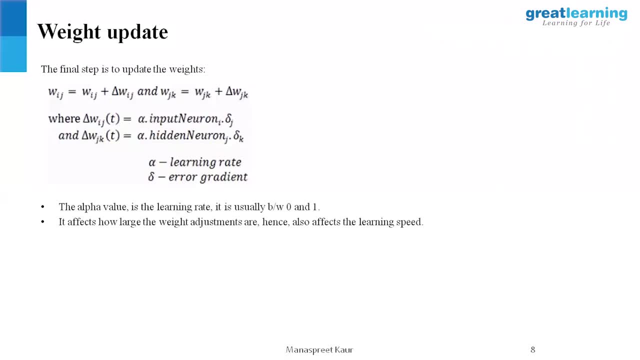 network. so when back propagation will occur, some errors would have occurred and then a back propagation will occur. that error will be passed back to the algorithm. the weights that are being passed, that are being applied to the input data variables, will be modified. the weights that are being applied to the hidden layer will. 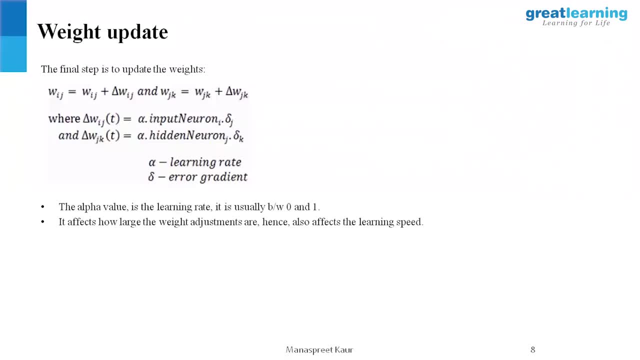 also be modified and, finally, a new output will be produced. and this process repeats across multiple iterations, and each time the weights will be updated. okay, then we come to the error function. error function is nothing but again the difference between the error function and the error function and the error function. 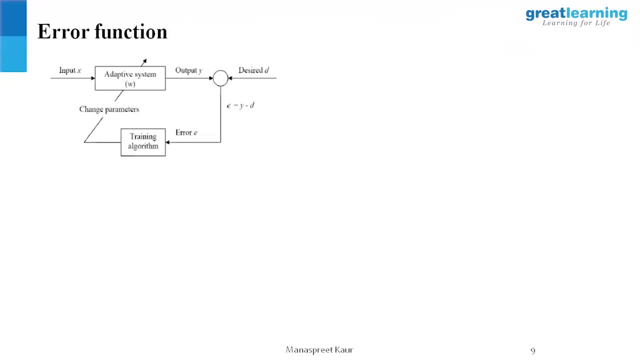 will be the difference between the actual value and the desired value here. so although this is repetition, but the input variable will be passed through a system. so adaptive system here is nothing but the hidden layer. and then you get a output y you compare that output to the desired. 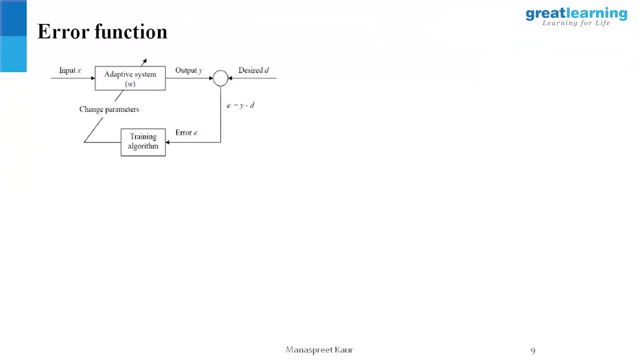 output. whatever is the error is passed back to the adaptive system- nothing but the hidden layer. then the weights are modified. so one thing to keep in mind is that the error should satisfy some particular properties. this was- this was present in the videos as well that we saw, the first thing being that the error 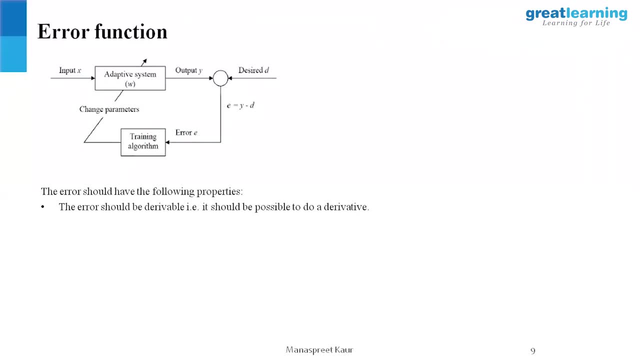 should be derivable, meaning to say that it should be possible to do a derivative. derivative is nothing but d by dx, what we used to do back in 11, 12 mathematics. so it should be possible to do a derivative y. to answer to one of the questions earlier, the threshold that we calculate the 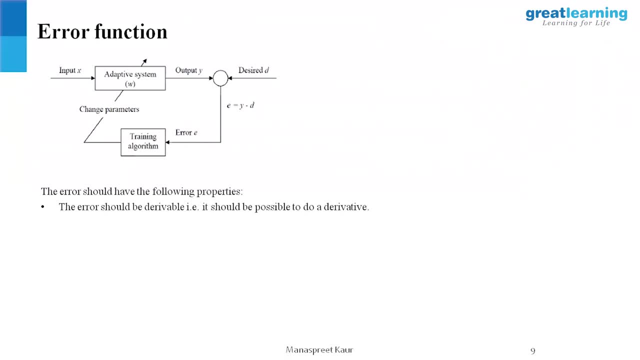 threshold that we specify is a derivative of the error. okay, so if, if it is not derivable, so the threshold thing will not work. the threshold that we are specifying, that we are telling the algorithm is nothing but derivative of the error that we are getting in each layer. okay, 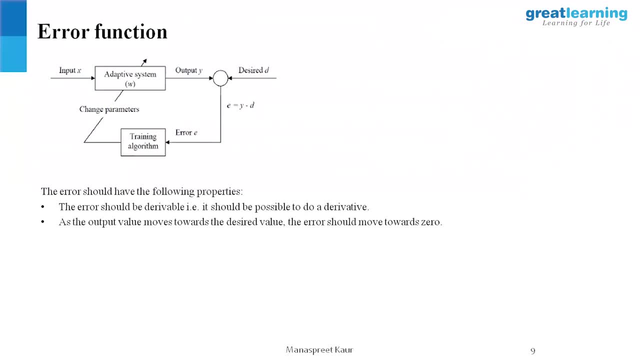 as. so this is very obvious, although. but as the output moves towards the desired value, the error should obviously move to zero. error should be negative again, for the reason that we should be able to do a derivative of it, and then we need to choose the error, the error value. sorry, we're. 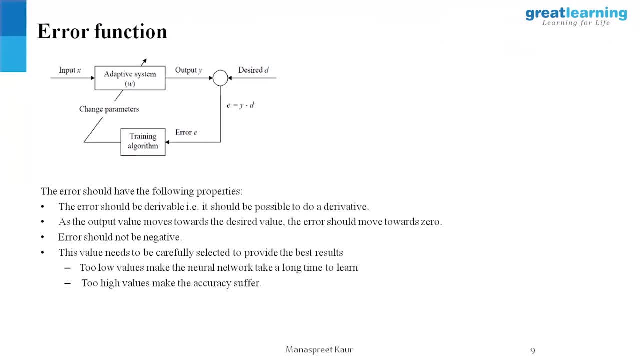 not choosing the error value actually, but then when there is a value for the error or there are too high values for the error, that actually impact how the neural network works. if the error value is too high, the accuracy of the neural network will be bad and then it will take a lot of iterations to be able to learn. and if the error value is too small, 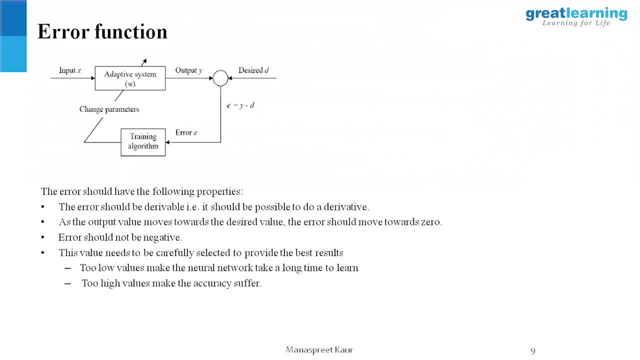 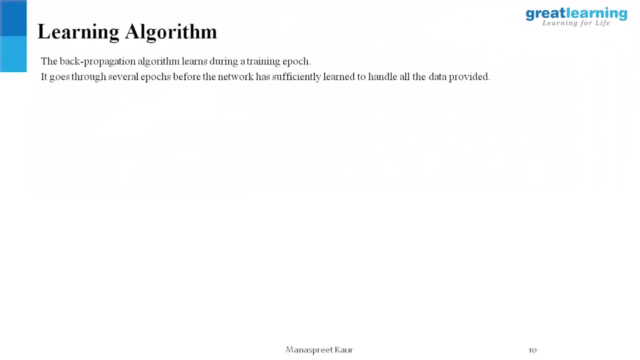 sorry that I've put it opposite. so if the error value is high, then the neural network will take a long time to learn. I'll just change it after the session. okay, so we'll finally see an overview of what happens with the learning algorithms in the learning algorithm overall. so the back. 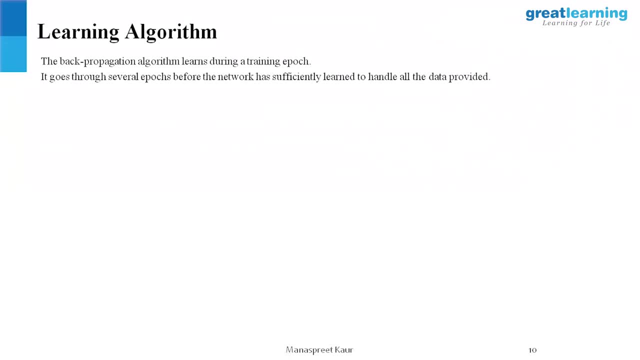 propagation actually allows the neural network to get trained, similar to how we train all the machine learning, all the data mining models. similar way, the back propagation allows the neural network to learn. this happens in multiple iterations, what I've been calling so far these iterations, in terms of 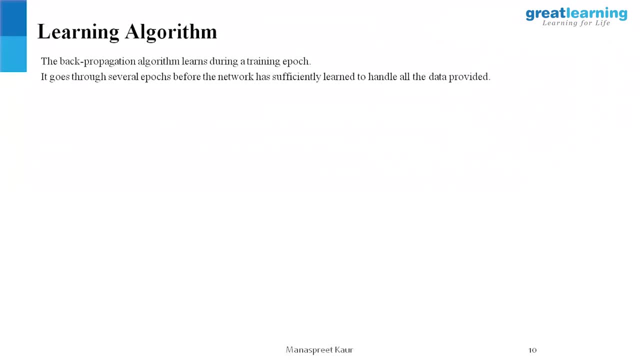 neural network are also called as epochs, so it goes through several epochs before the network has sufficiently learned to handle all the data that is provided. this is again a different diagram, shown in a different way, to show how back propagation works. but if that will happen, this is that will happen for each of the iteration. 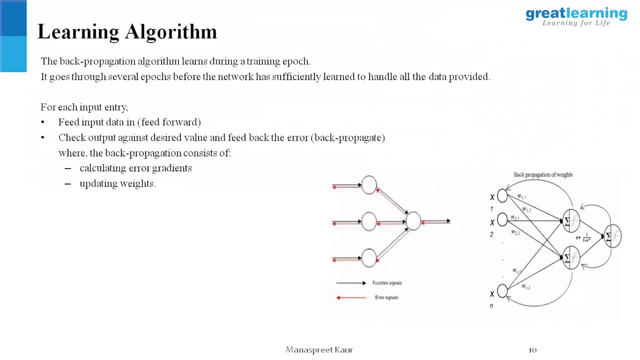 and each of the epochs. the input data will be fed, the output data will be compared against the desired value and then it will be. whatever the error will be will be back propagated using the error to update the weights. now, when will this stop meaning to say that each time when a particular error is calculated based on what was? 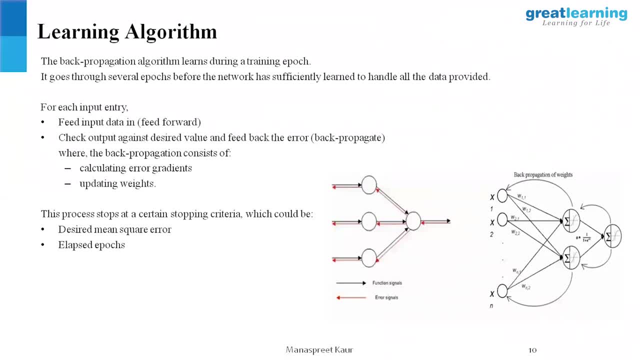 the output versus what was the desired output, and then a back propagation occurs. so this process keeps on repeating. so like we used to have a pruning step or a stopping criteria for the decision trees that we saw last week, similarly there should be a stopping criteria here as well. 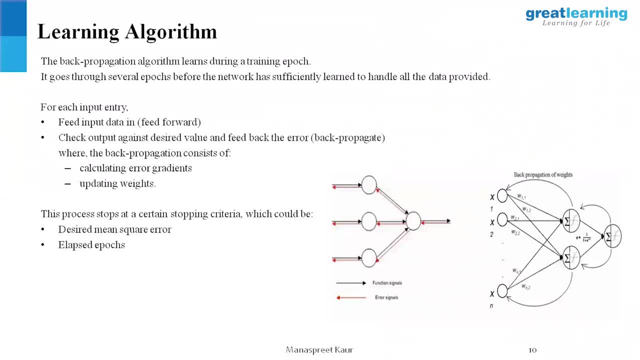 so multiple stopping criterias can be used for neural networks, one of them being a desired mean square error and one of them being elapsed epochs. desired mean square error tells what is the error that we can allow the data to have, what is the flexibility that we're giving the data to. 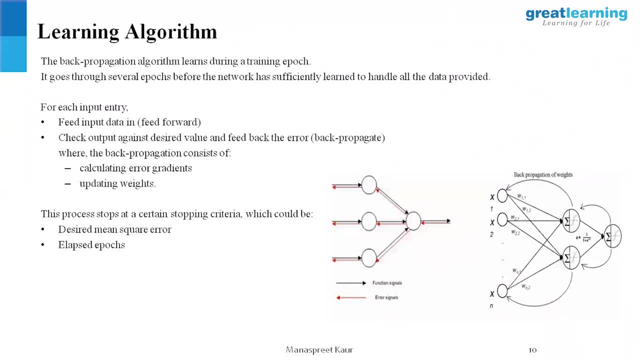 have and elapsed epochs is nothing. but what is the number of iterations that we want? so a neural network cannot run indefinitely through 10000 or 1 lakh iterations. this varies with the data that you have, so so it cannot run indefinitely. so we need to specify the number of iterations for which a neural 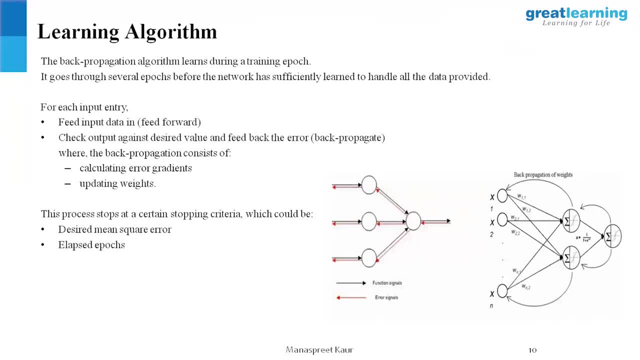 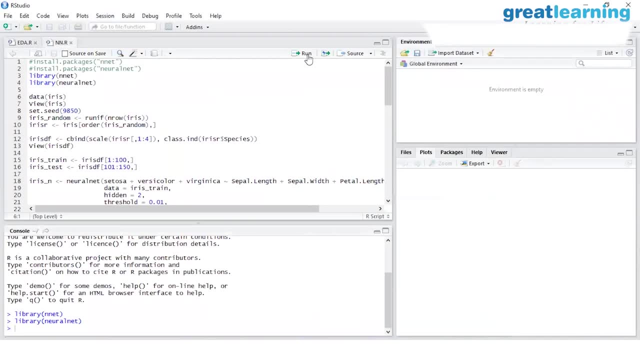 network should run. so both of these are used as stopping criterias for the neural network. okay, so again i'm using the iris data set that we had seen with the previous algorithms as well, to give you a quick revision of what the iris data set was. so this data set has 150. 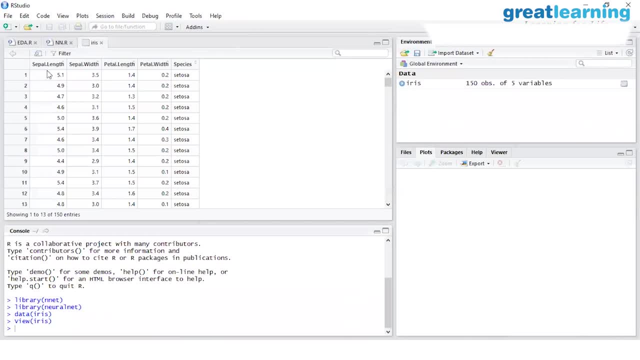 entries and which there are four input variables, which are sepal length, width, and petal length and width, and, finally, there are three species, 50 of each species, and the aim of this algorithm is to try to predict what the particular, what is the species of a particular flower given its attributes? 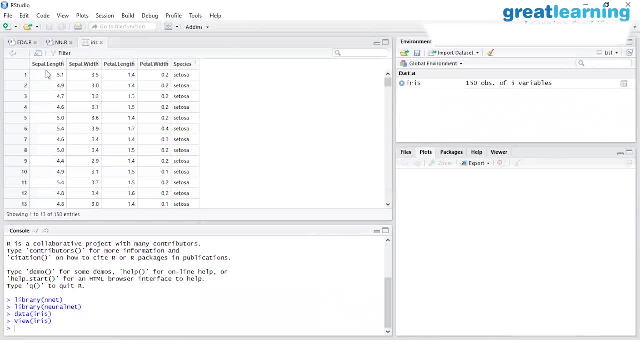 of sepal and petal length. so with the last session we try to predict the species using cart, using random forest. we also saw the same example with clustering as well, when we were trying to use the sepal length, width and petal length and width to try to cluster these flowers together. so we'll use 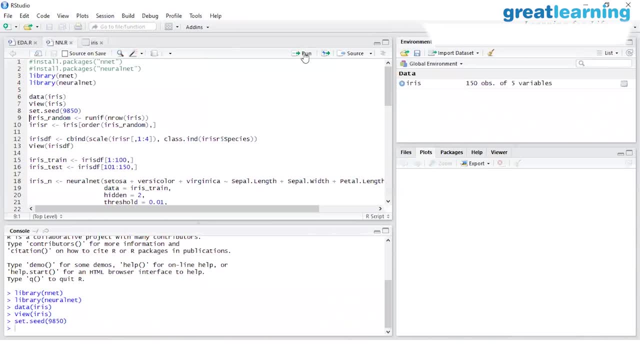 that same data set. i'm repeating the steps, what we did earlier, of generating a random number, shuffling the data. so this again is an idea of using a random number data. so this again is an idea of using a random optional step, but i normally do it so that there's no biasness which is present in the data. 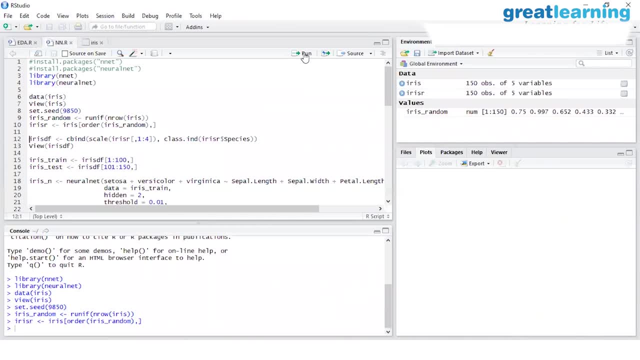 one important step uh, which you can note down here, is the line number 12, um that i have uh with the r code. so, if you remember, with um neural network, uh, this was being done in the example that we did and this will also be useful in the example that you do with. 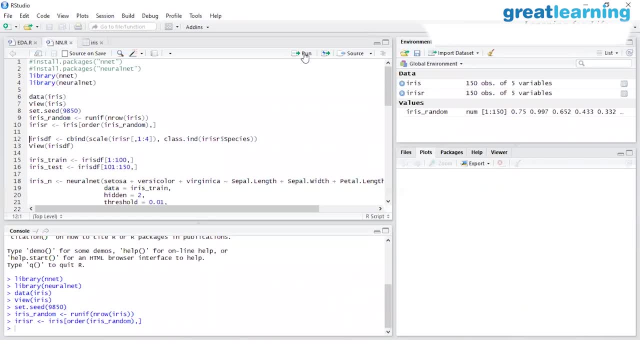 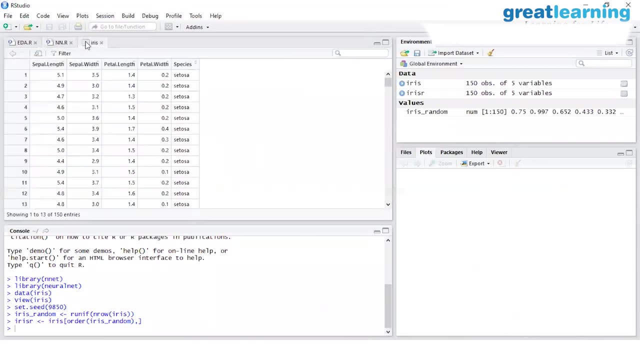 uh, your mini project. so if there is any variable which is a categorical variable, something like um, the species that you have here when it- where is this? where it is sedosa, uh, versicolor and virginica, when you have three species, you cannot have the data in this format when you work with. 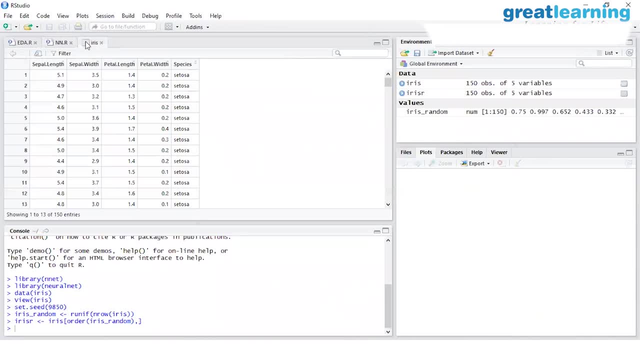 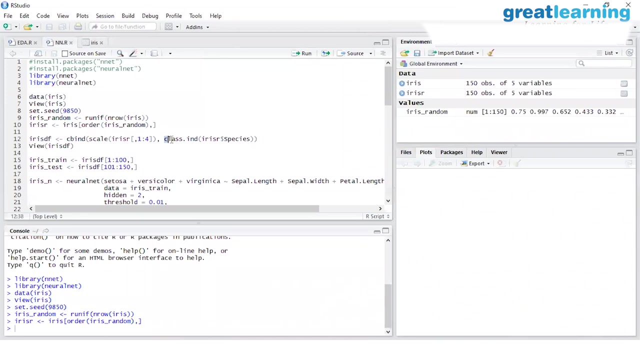 neural networks. so you need to have um three columns which are in forms of uh, one and zero. so, um, either you can do that with multiple commands, either you can create um three new input variables and then pass one or and zero here. but a simple step, a simple command is the class dot. 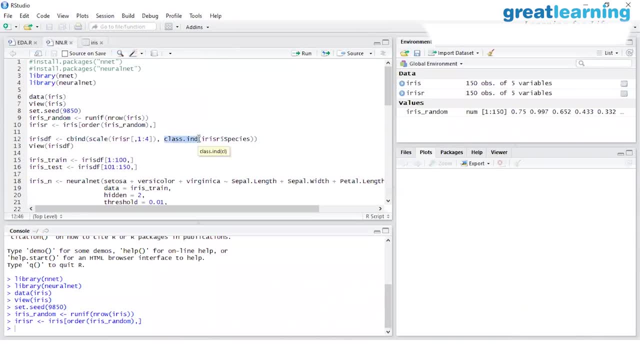 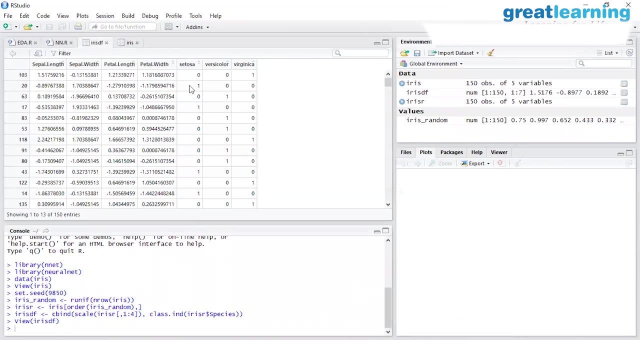 uh int command which you can use in one go to create all the three variables. let me show that to you how it happens. so if you see, here with a single command i am able to segregate the initial species that i had, if you see, the species i had here was: 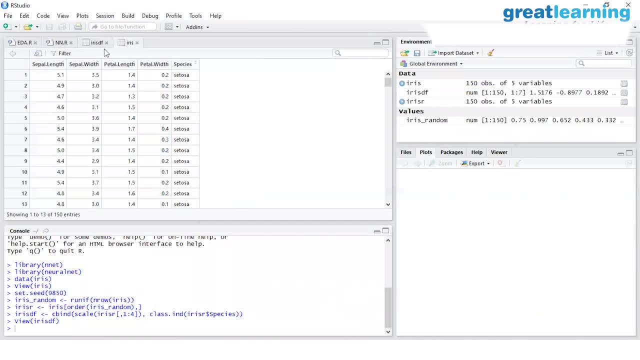 um, in the form of setosa, virginica and versicolor, and then i've split that data in form of zero and one, with one single step. okay, so, um, what was done earlier was we used to create? we used to do that, uh, for each of the variables one by one, but using this command, you can now. 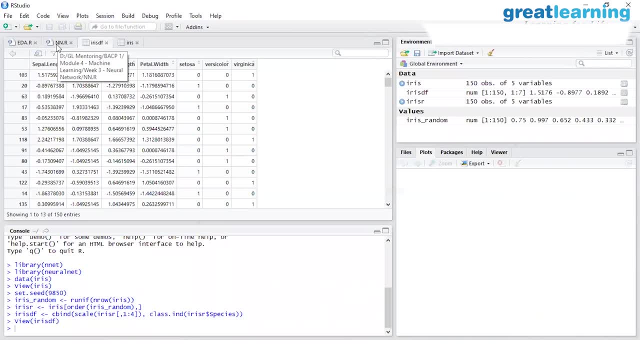 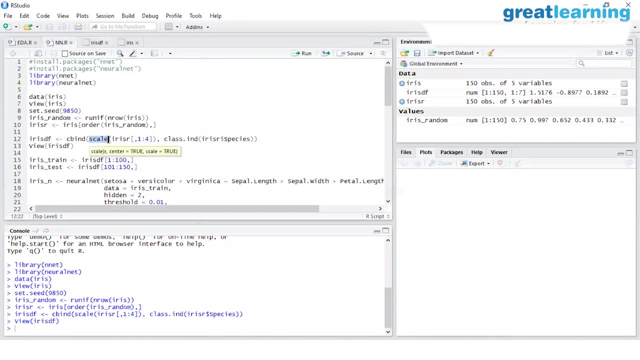 very simply split the data in the required format. okay, and as a shortcut, what i've also done is i've done the scaling in the same command here. so what i essentially did was, from the initial irisan data set that i had, i scaled the first four variables, so the first four variables of separate length. 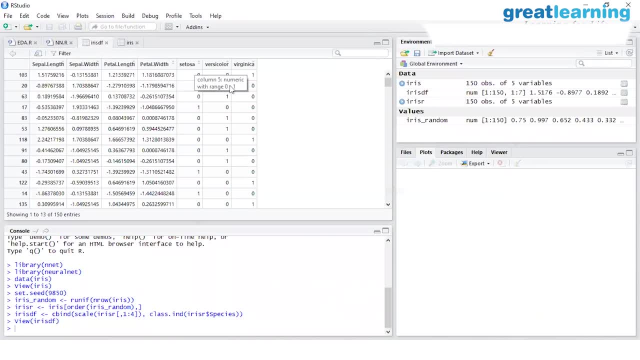 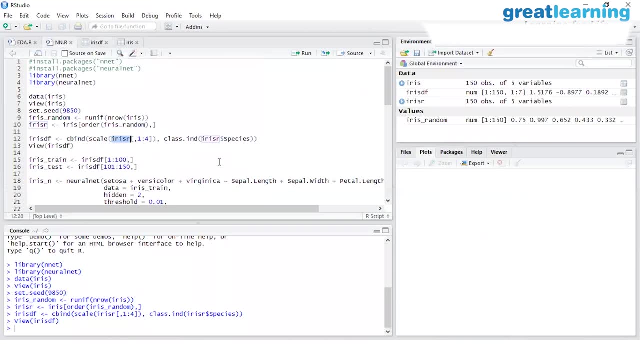 width, pet length and width was scaled, and then this, with uh, the output variable, which was one split in the form of zero, one, one to be able to fit the neural network. so then i am um, simply dividing my data set into training and testing data set. uh, so roughly a 70, 30, but not exactly. 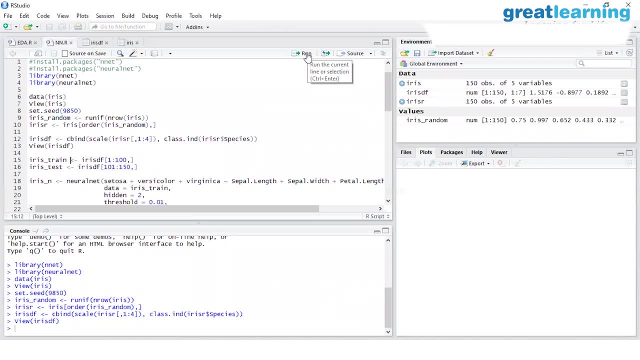 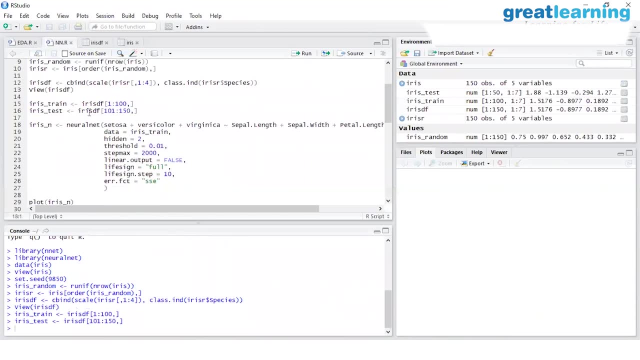 so, first hundred, i'm passing to my first hundred rows and passing to my training data set and next 50 to my testing data set and finally, i'm creating a neural network. so we'll see here what is going to happen when i'm creating a neural network. um, so the first thing is the formula that we need. 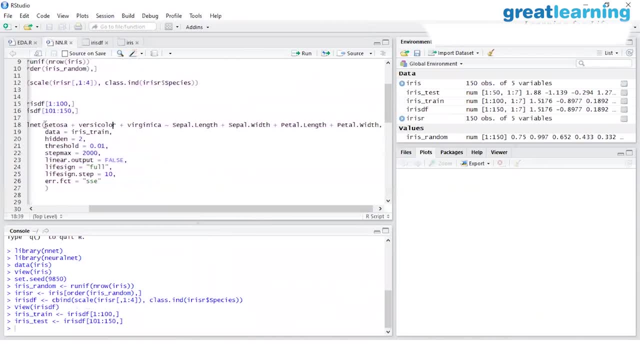 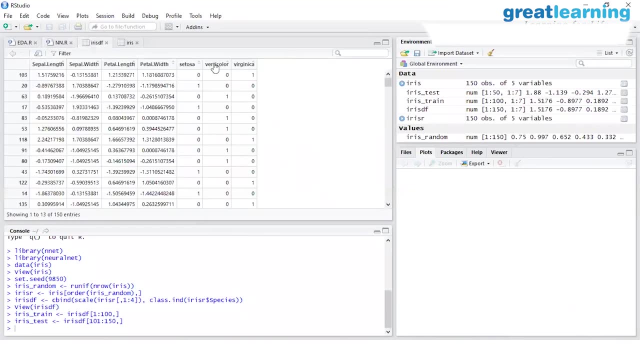 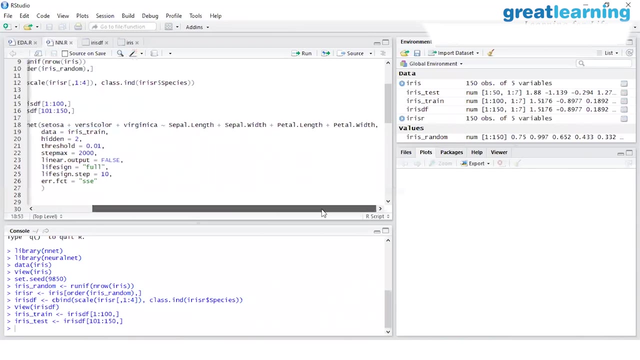 to give here. so the formula here tells me that these three, which now become my um output variables, um c, cytosa, versicolor and virginica, which now become my output variables, are a function of four independent or the input variables. so this is the formula that i've specified. 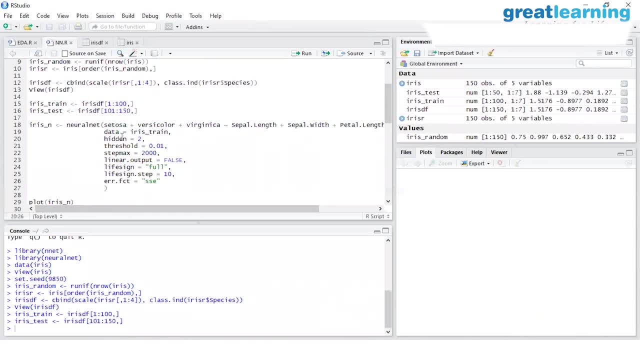 data is the training data set hidden specifies the number of hidden layers that you want, um. so a thumb rule to choose the hidden layers is uh under root of the number of uh input variables that you have. so if you have, i had four input variables here, so i chose two. 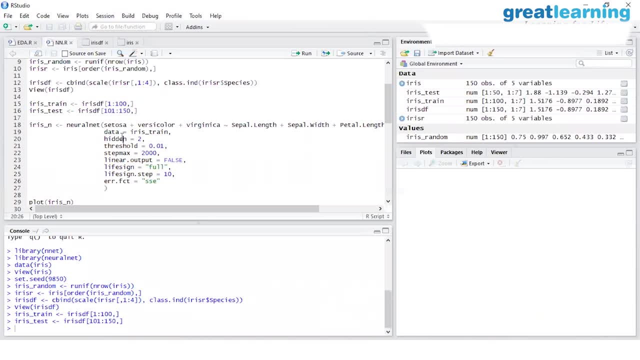 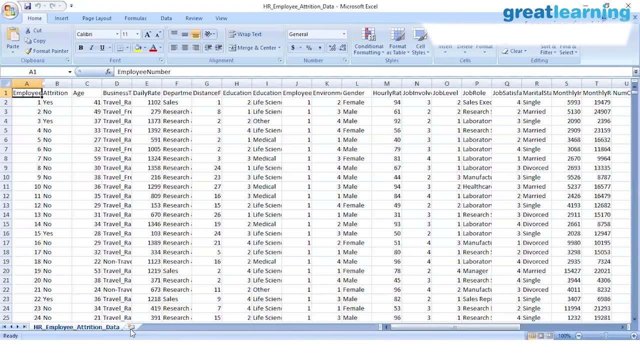 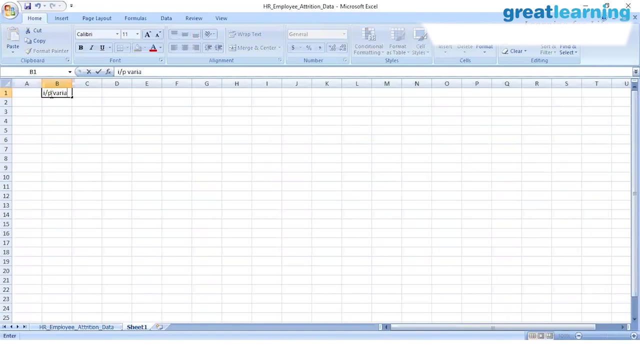 okay, and um, since you saw you can have multiple hidden layers here, um, so say, if you have, um, uh, maybe, like here, i had one second input variables and hidden layers. so, since i had four input variables, i did a square root of this to choose that i'll have two hidden. 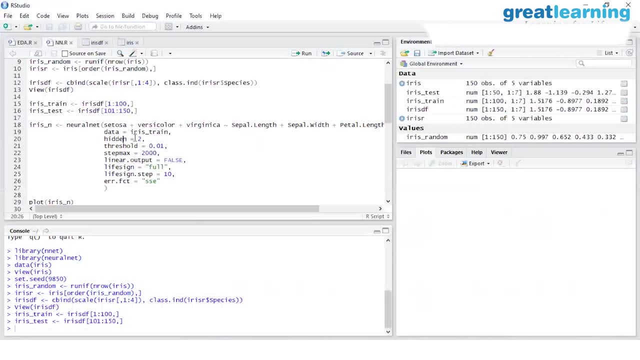 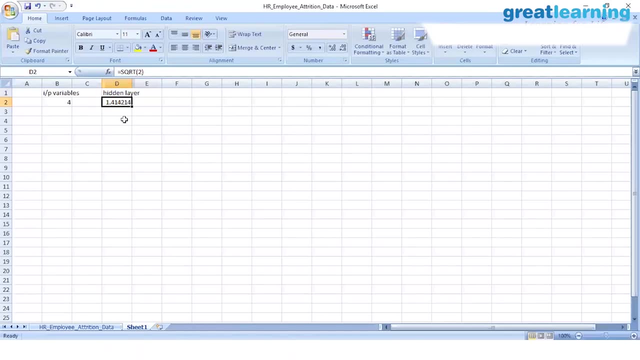 hidden equals two. two here give me a second, okay, and um, sorry, uh. so terra means i'm rounding it off to get a two. so that will mean that i have one hidden layer with two neurons. say you have, um, maybe 20 input variables of in place of four, so you do a square. 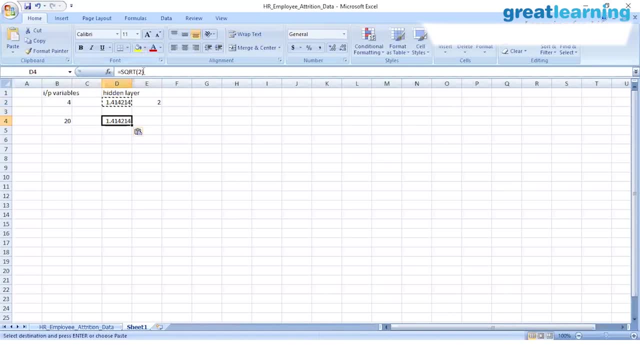 root of 20, which will be 4.47. now new round it off to 5. then you do a square root of 5 and that will be 2.23, so you can round it off to probably 2 or 3. so what I'm trying to tell you is that when there are 4 input variables, I'll have 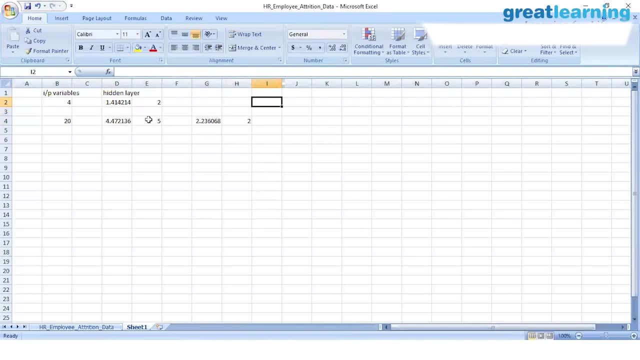 just one hidden layer which will have two nodes. when you have, say, 20 input variables, you'll have two hidden layers, the first of which will have five hidden neurons, the second of which will have two neurons. okay, making sense, like if I have hundred input variables, I'll have a first hidden layer which will have 10. 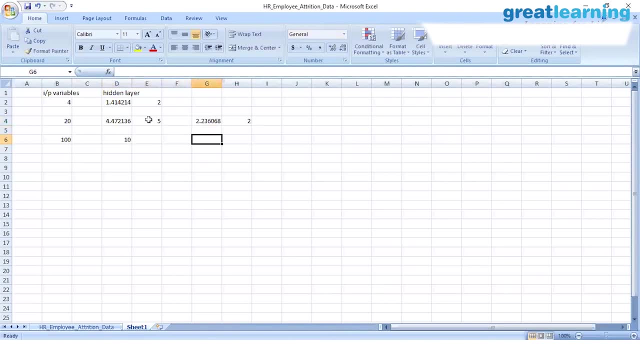 neurons, then I'll have second hidden layer which will have three neurons. then, uh, yeah, so that will be here. um say, i have 500 input data variables, so i have first hidden layer which will have um, say, 22 hidden. sorry, i'll have first hidden layer which will have 22 neurons, then i'll have um second. 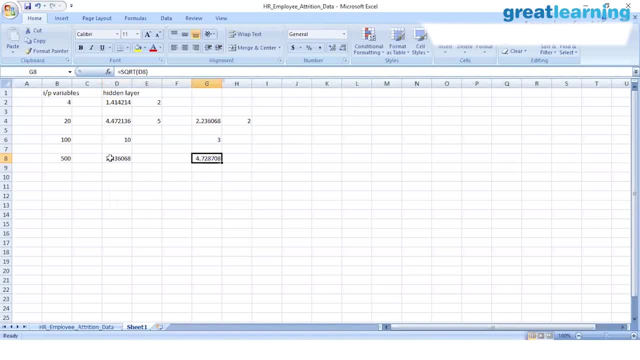 hidden layer, which will have 4.7, or you can round it up to five neurons. then again i'll have third hidden layer, which will have two neurons. so this is how you decide the number of hidden layers that you have, with the data and number of neurons that will be present in each hidden layer. 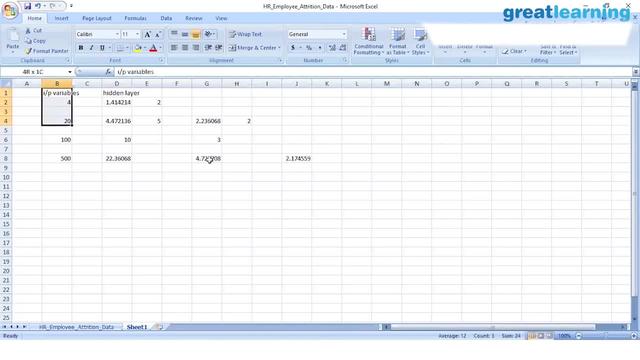 let me. let me kind of erase this and do this again. okay, so input variable and then the hidden layers. so when i had four input variables, i do a square root of four. that will be two. so i have one input layer which has, so this will be the first. 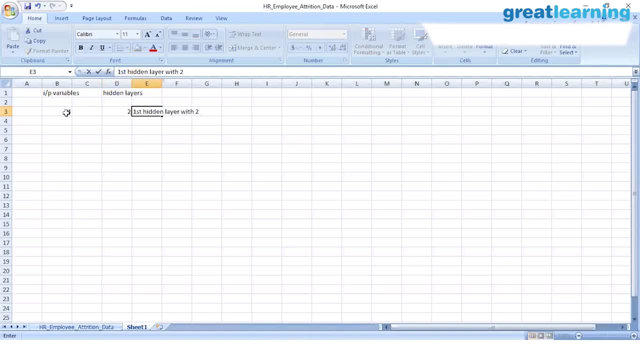 hidden layer with two neurons. okay, i'll kind of keep doing the square root multiple times. so i'm doing a square root here the first time. second time, when i do a square root of two, i come to approximately one. so then i stop. okay, meaning to say, when i have four input variables, i get a two. so that will be first. 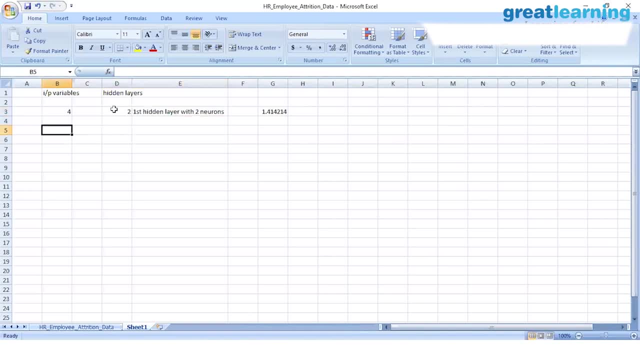 hidden layer with two neurons. say, if i have ten input variables, i'll do a square root which is approximately equals to 3.. So I'll have a first hidden layer with 3 neurons and then I'll do a square root of 3 which is 1.7, and you can round it off to: 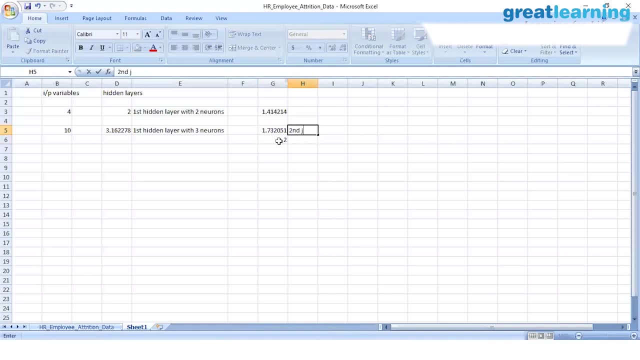 2. So I'll have a second hidden layer with 2 neurons. Now, if you do a square root, you keep on doing the square root iteratively. So now, if you do a square root, you'll get something like 1.4 or something. So there you stop. So with 10 input variables you'll 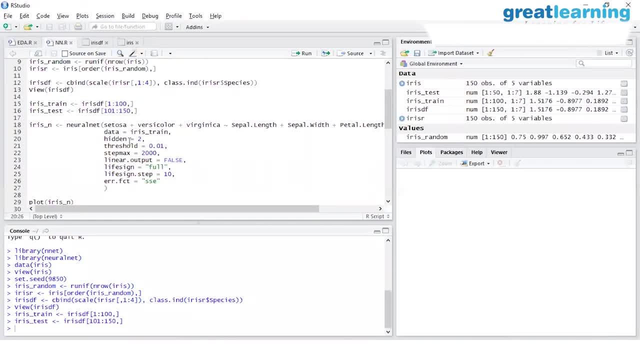 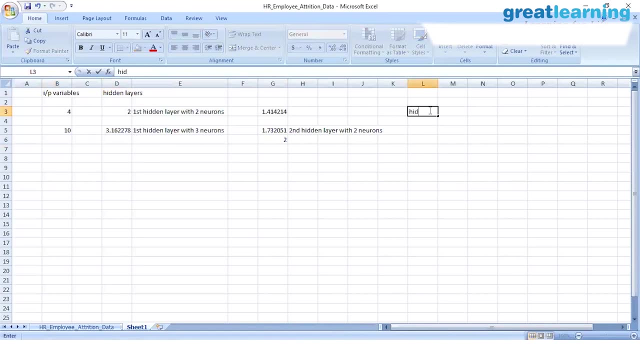 have 2 hidden layers. So with the hidden layer parameter that you're specifying here I did a 2 here Because I had just one hidden layer. So you need to give hidden equals to 2 here. With the 10 input variables you need to give hidden equals to C of 3, comma 2.. 3 means first with 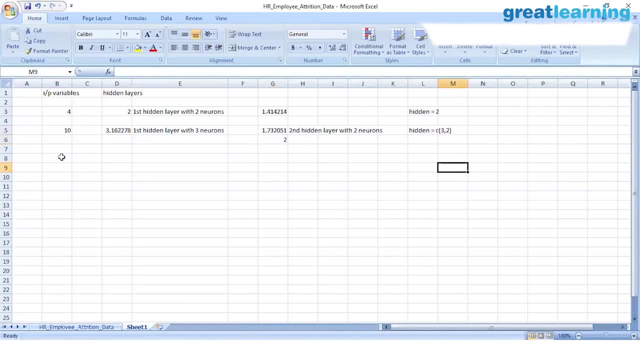 3 neurons, second with 2 neurons. Okay, like a bigger example, if we take, I have 500 input variables, So I do a square root of 500. That will be say 22.36. And I'm rounding it off to 22.. So I'll have first hidden layer with 22 neurons, then I'm 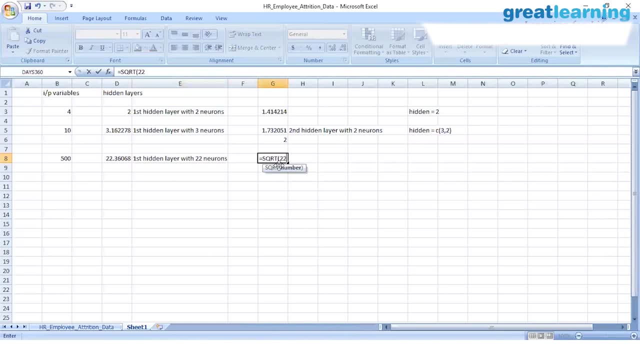 doing a square root of 22.. That gives me 4.69.. And if I round it off to five, so I'll have a second hidden layer with five neurons, then I do a square root of five. square root of five. Okay. 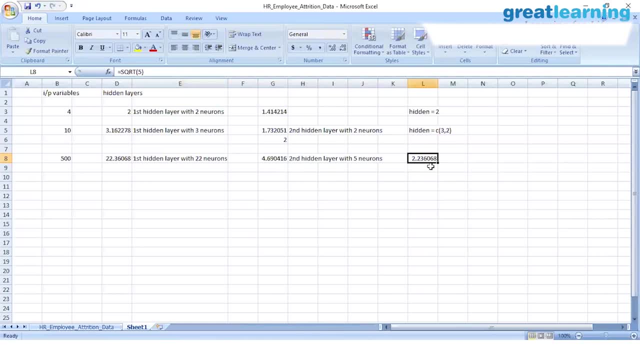 Okay, So I'll have 5.5, which gives me 2.23.. So I round it off to two, for example. So then I'll get a third hidden layer with two neurons, And then, when I'm doing this with R, I'll. 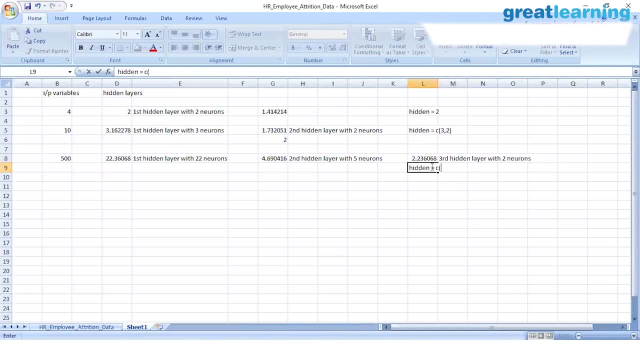 give hidden equals to 22 comma 5 comma 2.. So this means three layers, first having 22 neurons, second having 5.5.. So I'll have a third hidden layer with two neurons and then I'll have a third hidden. 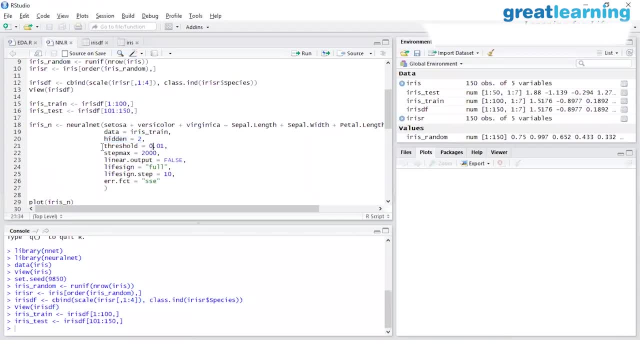 layer with two neurons. So I'll have a third hidden layer with two neurons and then I'll give hidden equals to 22 comma 5, comma 2.. Okay, So next is the threshold. So threshold is nothing but a derivative of the error that. 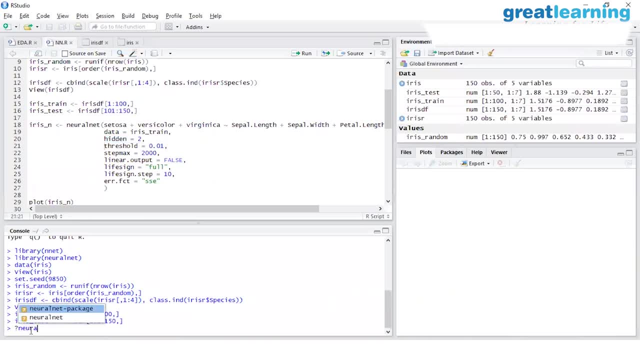 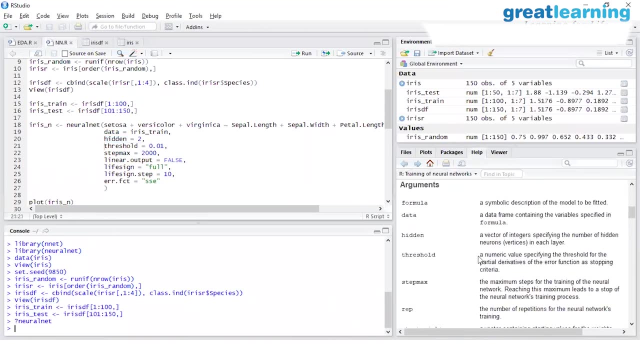 will be calculated at each step. So we can also see that from the help in R, See the threshold. So threshold is numerical value specifying the threshold And then the threshold will be calculated, for the partial derivative of the error function as a stopping criteria. 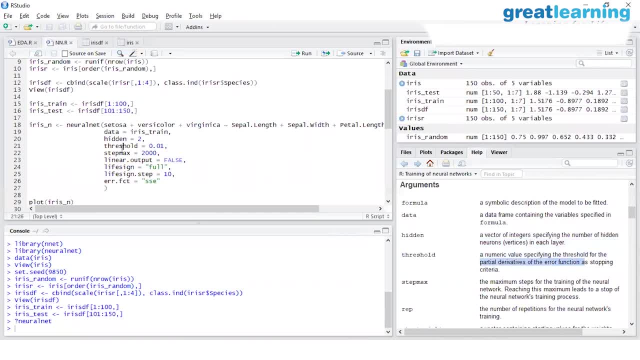 So at each step some error will be calculated as a difference of the actual value and the desired value, and then you calculate a derivative of it. So say, the error in the first step is 2, for example. So you calculate a derivative of it, then backpropagation will occur. then 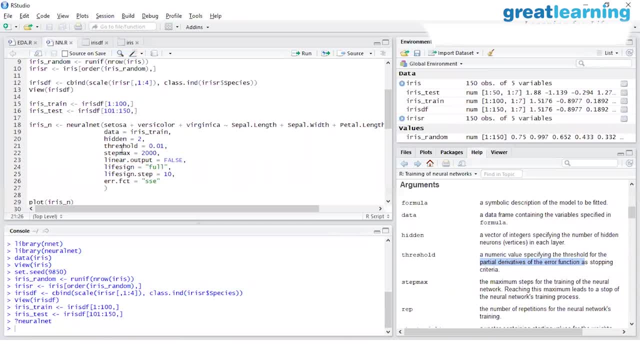 a reiteration will occur, will occur and this process keeps repeating. so this threshold equals to 0.01 says that keep repeating until you receive a derivative of the error function, which is 0.01. okay, so in the first, the first iteration may be a derivative of the error function will be, say, for example, 1: 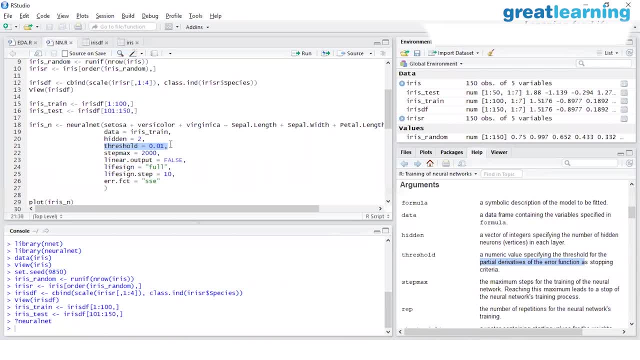 then you back propagate, reiteration occurs, then the derivative of the error function maybe comes down to 0.9. then you repeat, the back propagation occurs, then maybe the derivative of the error function comes down to be 0.6, then 0.2, 0.1 and till it comes down to 0.1. you need to keep. 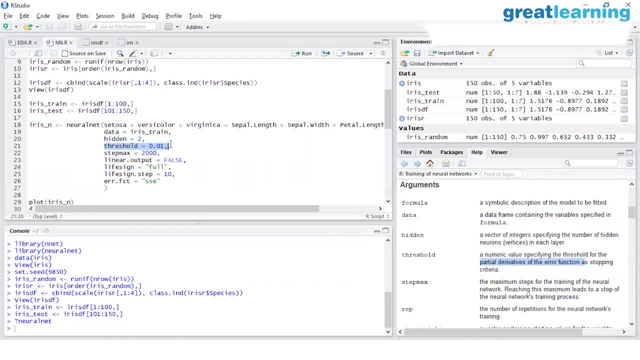 repeating the algorithm. okay, um, the next step is: so you- this is um one stopping criteria. threshold is one stopping criteria. step max tells you what is the number of iterations you want. it is possible that, um, even with 10 000 iterations or 10 000 cycles, the threshold 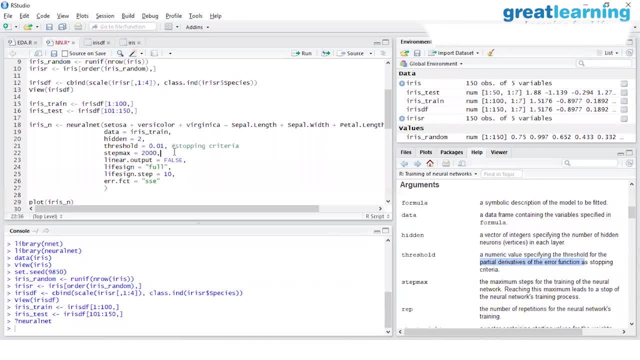 doesn't reach 0.01 doesn't mean that you'll keep running this algorithm infinite times. step max is another stopping criteria, which tells us what is the number of iterations you want. it is possible that, um, even with 10 000 iterations, it is the number of iterations that we can allow our neural network to have. so step max equals to. 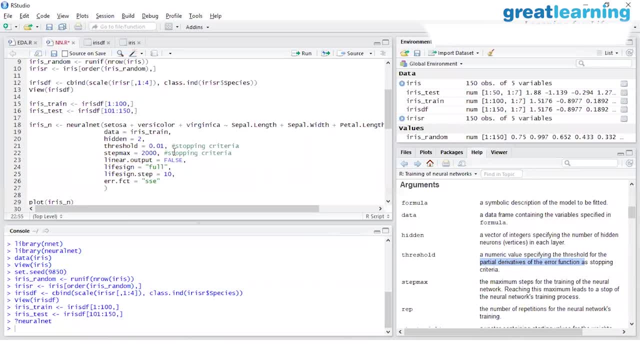 20 2000 tells us that we need to. um, we can run this algorithm a maximum of 2000 times. okay, so linear output equals to falls. is nothing but um, telling whether or not you want the activation function to work. so, uh, to revisit activation function was nothing but allowing a neural network to fire a trigger. 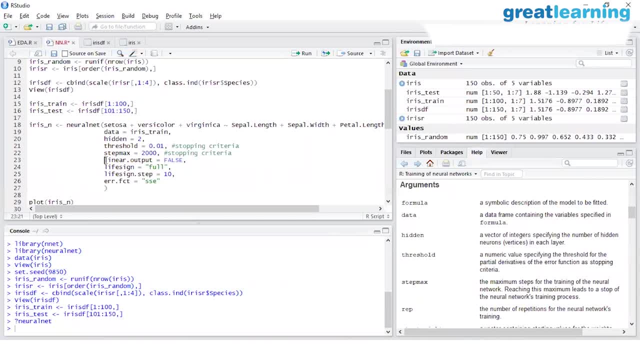 firing a trigger means allowing the neural network to backfire, so sorry, backpropagate. so when when you specify linear output equals to false, that means that you're allowing the activation function. okay, so with with the lectures there were different activation functions that were also given, but there is not much difference practically speaking with the different activation. 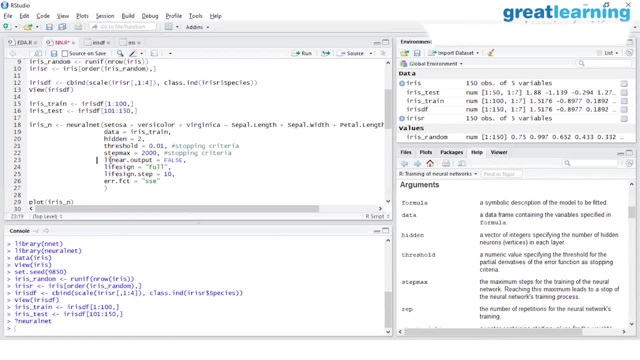 functions, and even if you don't specify it explicitly with your commands, you're you're not missing out anything. just specify that linear output is equals to false. this is enough to tell that you want the activation function to work. okay, then life sign equals to full and life. 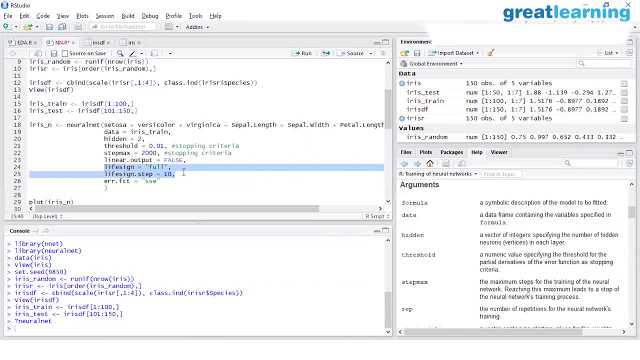 sign dot step equals to tenor, again optional. okay, so if you want to specify it explicitly with the commands, you're not missing out anything. steps um: these are only to tell r that say, i am telling here that i want 2000 iterations, so these two steps are only to tell r that i want to see the output after every 10th iteration. 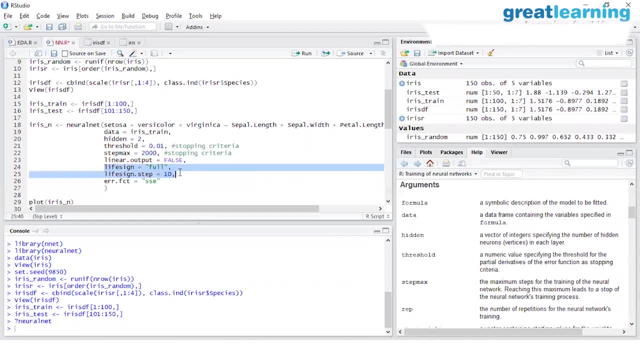 if you, if you step, if you skip this step, even then the algorithm will run, but it will not show you what is happening with uh each step. so when i'm telling r that i want the life sign step to be 10, so after each 10 iterations, like after 10 iterations, after 20, after 30, after 40, so on till. 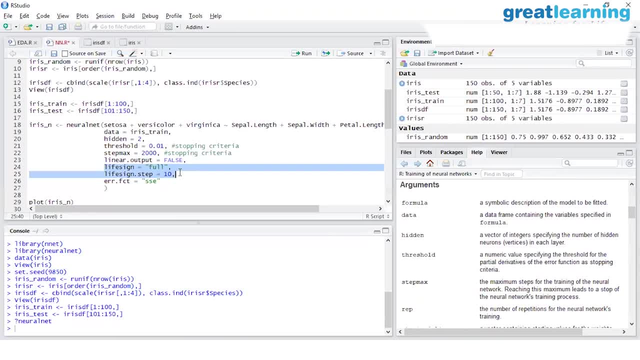 2000 r will show me what is happening with the neural network. if you skip this, it will directly give you an output. okay, then uh, errorfct is nothing but uh, telling you how do you calculate the error function. okay, um, so error is error, function is nothing but. 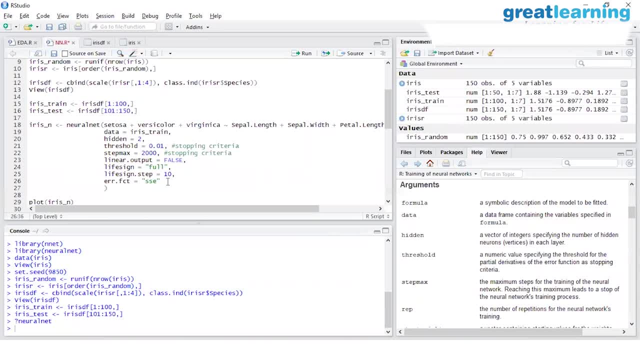 difference of the actual value and the desired value. but how do you calculate it? ssc is sum of squares, error, and this is the best you can do with neural networks, because with neural networks, you want your error to be positive, uh, so that you are able to do a derivative of it. um, so, the best. 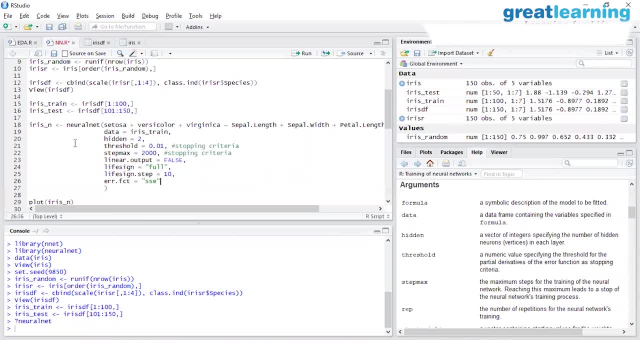 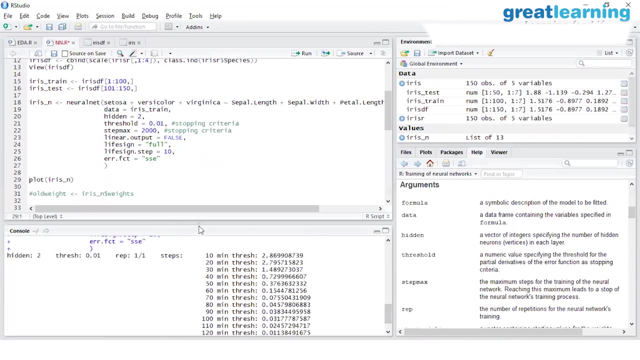 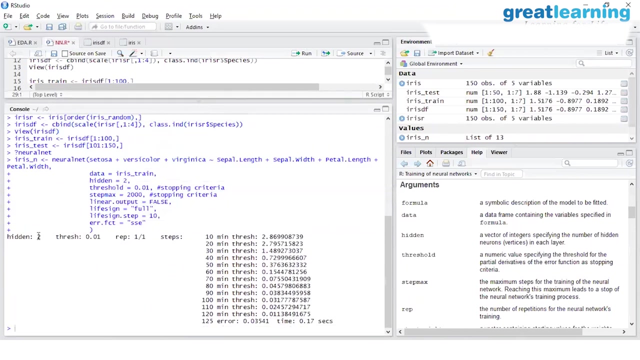 thing to use is an ssc, which is sum of squares. error. so supplying all these parameters when i run this command. sorry, okay, so i ran this command. see, there are two hidden neurons. that was what i had specified, uh, with each iteration. so i told that i can do a maximum of 2000 steps, uh, but my algorithm stopped with 125 steps. uh, so when 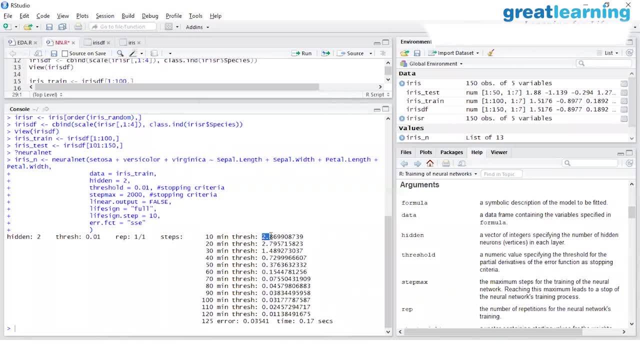 there were 10 steps. when 10 iterations had occurred, my error was 2.869. after 20, it reduced to 2.795. after 30 it reduced to 1.487 and finally, after 125 iterations, my error reduced to 0.03541. 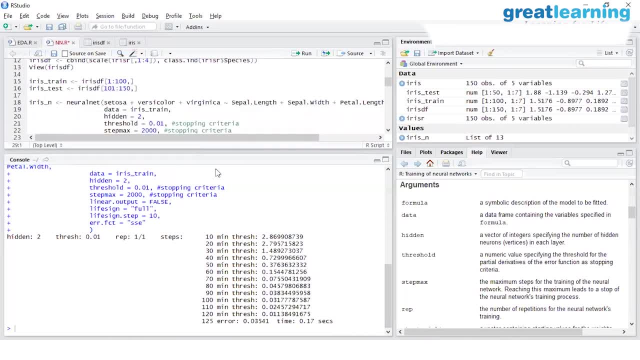 um, so the stopping criteria which worked here was this threshold, so a derivative of 0.0351 would have been lesser than 0.01 and hence it stopped here. okay, so once the error of 0.03541 was achieved, this was achieved with 125 steps, so i did not have to do 2.000 steps. so because there's no empowered choose interval: zero, zero, zero point zero, point zero 25, the test was not done until i managed to achieve this freakin litter, Swiss k, that means um. so the error eventually has to be global, even though the test isn't always perfect. so then, for the average, also work. 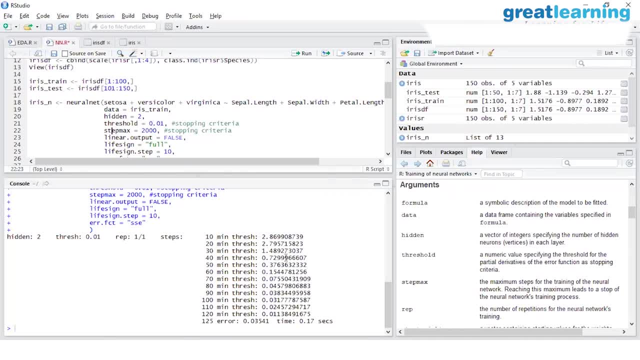 thousand steps. i got the output with each 10 iterations. you see, you can, you could have done a life sign, step of one, to see what happened with each iteration, but then becomes too detailed. so with each 10 iterations, you see the error was reducing and finally it came down to 0.0351. 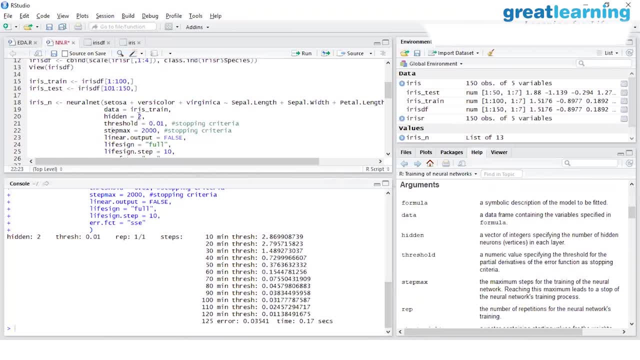 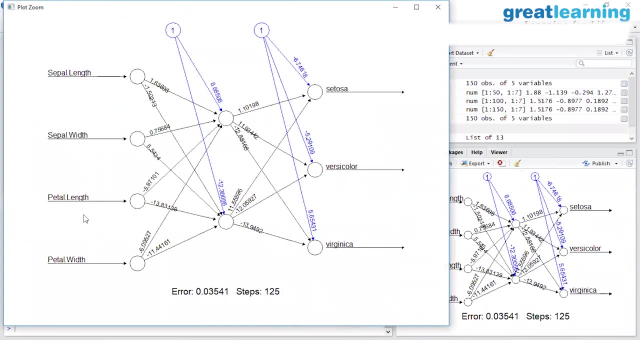 and this occurred in 17 seconds only. okay, now, if i kind of try to plot the neural network, this is what i get. so see, there are four input variables: sepal length, width, petal length and width. i have just one hidden layer that has two neurons. 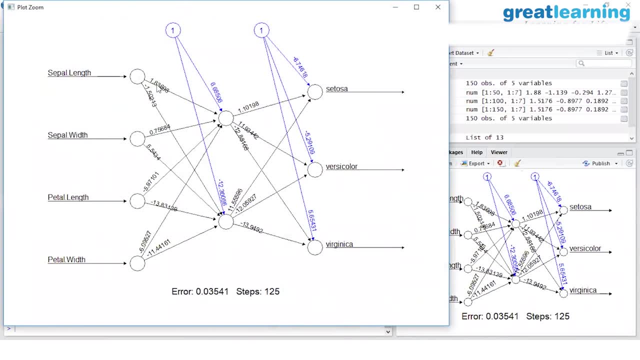 these are the weights, the ones that you see: 1.83 on the top second. yeah, so this one point three that you see- 1.83 that you see here- is the weight. these are all the weights that you're seeing, then the zero, the 6.6 that you see here, the minus 12 that you see here. 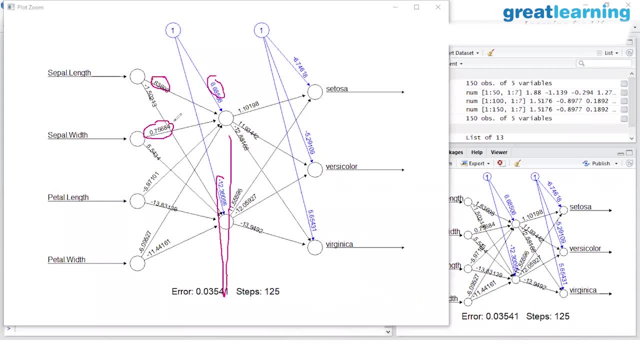 sorry, these are the biass. so 1.83, 0.76- the one that you see on the black lines are the weights that are being applied to the input variables. the ones that you see is the weight of each iteration in blue: 6.6 and 1.2. these are the biases which are being applied, so there's just one hidden layer. 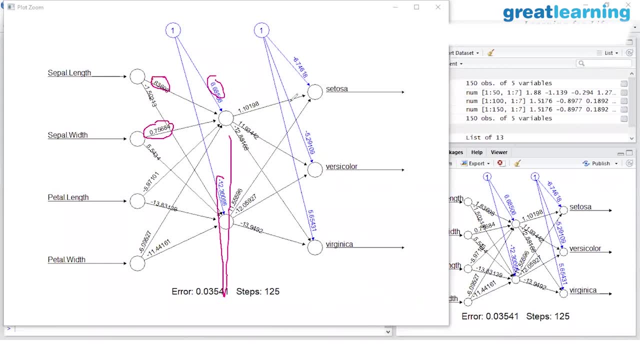 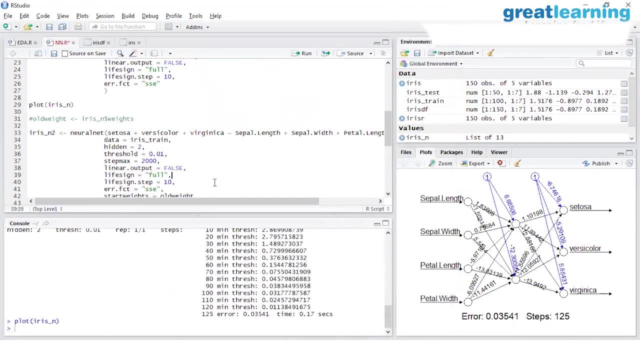 with two neurons. the biases are being applied at both the layers: the base, the hidden, the weights are being applied to both the layers and, finally, an output is being thrown out. okay, one thing to note here is that if I run the same command again, the weights will be different. okay, so if you run, 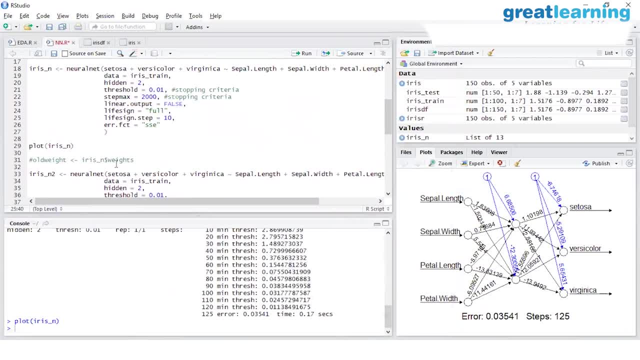 the same command at the same time with me. even then, this will be different. so far, what is happening is iris underscore n is a neural network model which is being created. it's just showing you that these were the four input variables, these were the three output variables, and something is happening. 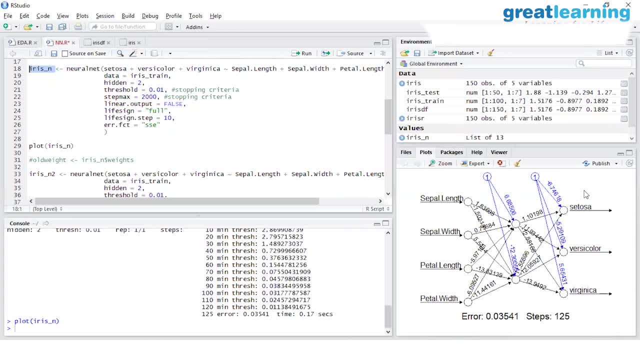 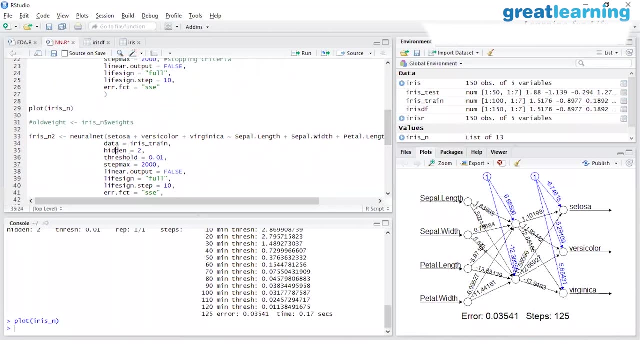 and this neural network is getting trained. okay, one additional step which can be done here is not with the small data set that I'm using, but if you have larger data sets. one another parameter that you can pass with the neural network command is this step, this parameter called start weights. okay, so what this is doing is that, even though 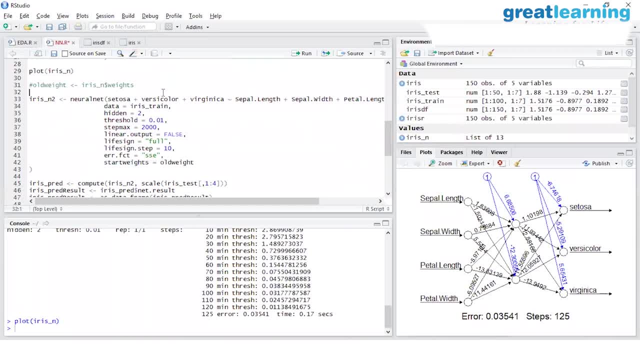 with back propagation. the errors are being passed and then the weights are being modified. but additionally, you can also pass the weights of the first step to the second step, meaning to say, whatever were the weights that were being applied in my first step, I can also pass them as a parameter when I'm 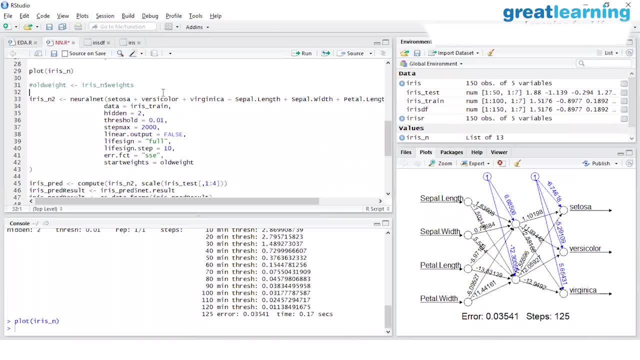 back, propagating to the second step, so that the same weights are not being used. so this becomes my second step- comes an additional learning for the neural network. so this is not applicable in the small data set that i'm using. it it won't do any benefit but for the larger data sets that are present, the 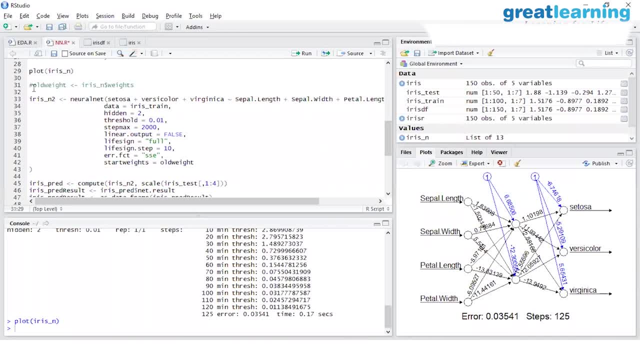 steps become helpful, then i'll show you how you do that. so you create another variable, old weight, or you can name it anything, and in the iris underscore n was the name of the model that i've created that has some weights. so i'm passing those weights to a new variable and then i can. 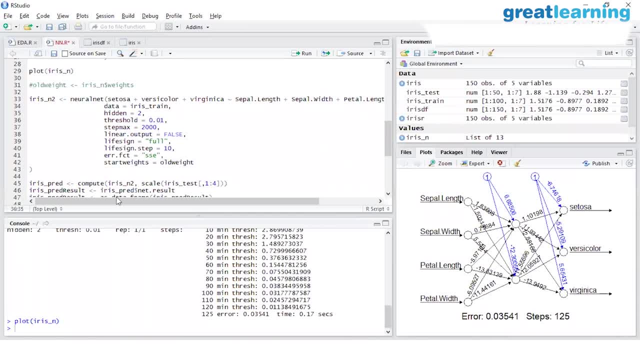 create another neural network which has the same parameters. additionally, i'm adding a parameter called a start weight, in which i am passing the old weights, that is, the weights that i received in the first iteration. so this is an additional step you can do to improve the performance of. 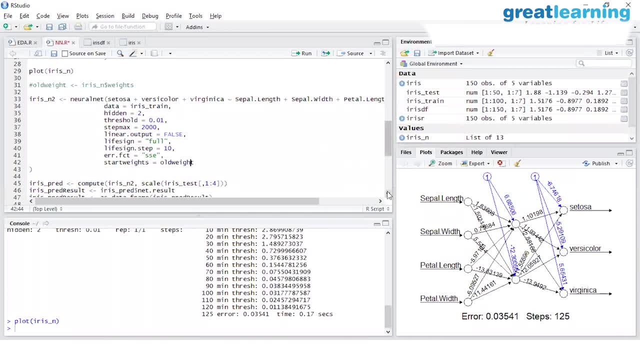 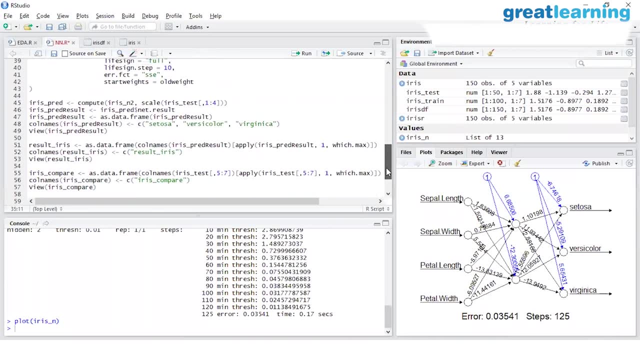 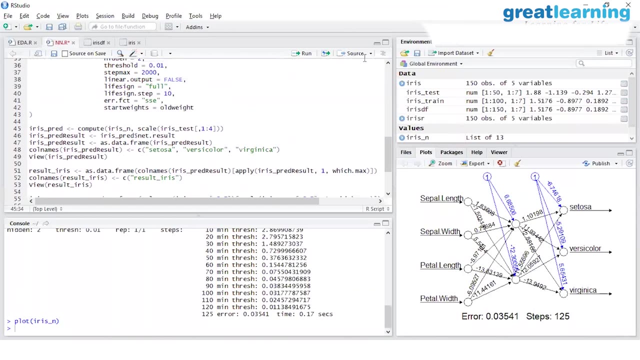 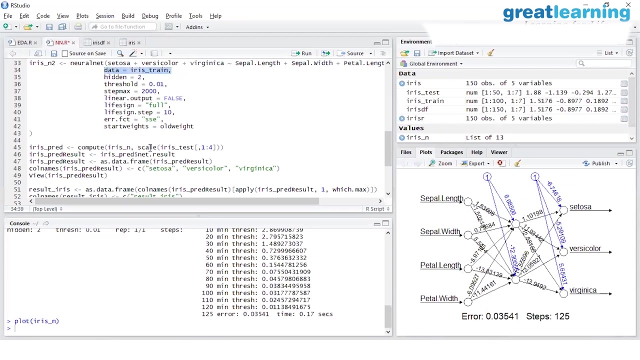 your neural network. okay, so so far, with iris, underscore n, i've just created a model. now we'll see how does our model work. okay, so what i'll do with uh? what i'll do here is uh with the data set. here i had used the training data set to create a model. next i'll be using the test data set to see how my model 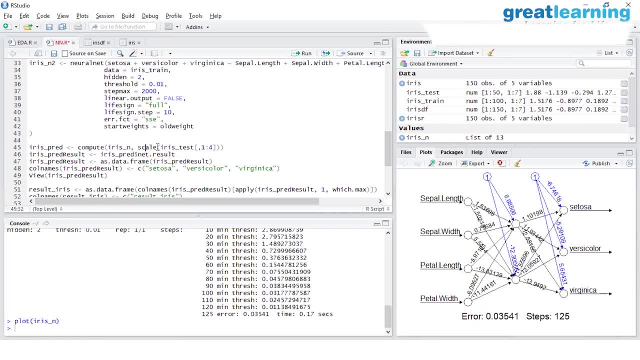 performs. so, uh, because i had scaled my training data set, so i'll also be scaling my testing data set and try to predict the outputs of the testing data set. so i'm using a compute function to predict the values of the output. uh, sorry, the testing data set, iris, underscore n, is the model. 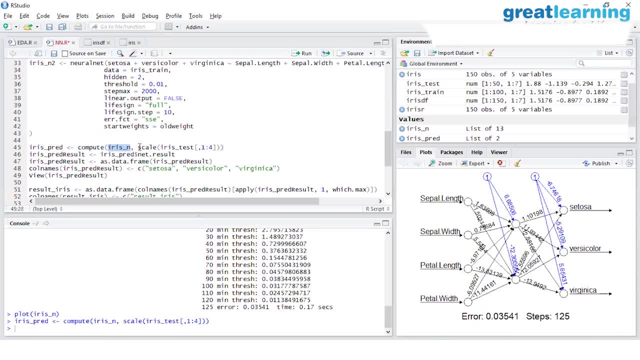 that i had created neural network model that i'd created and the data that i'm passing is the test data set. so i'm going to use the test data set and i'm going to use the test data set and i'm going to use the test data set and i'm going to give it the first four columns, which are nothing but the. 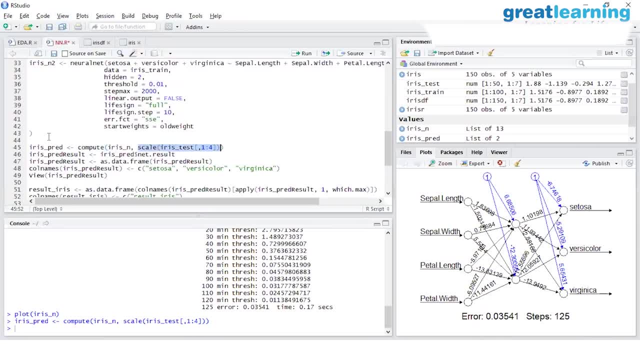 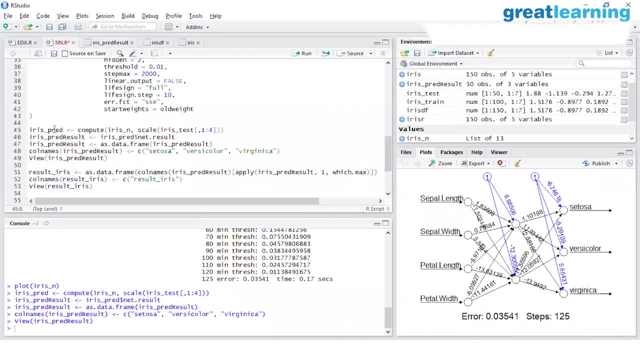 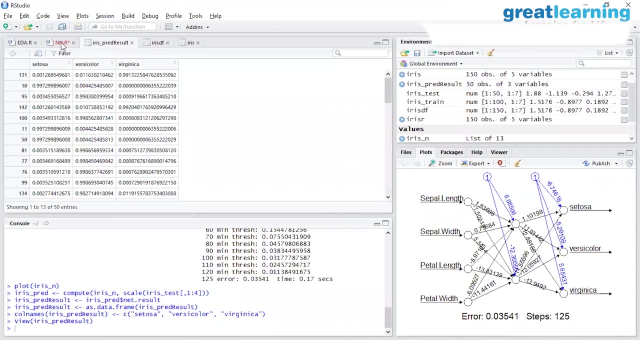 separate length, width better than that width. okay. so, finally, when i predict, when i try to predict the values of my test data set, this is what happens. um, now, since this is a scaled data set, so the numbers are achieved in this way, but you can again, uh, use these numbers as well to 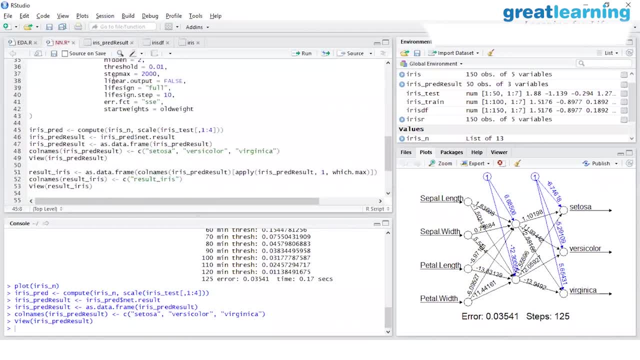 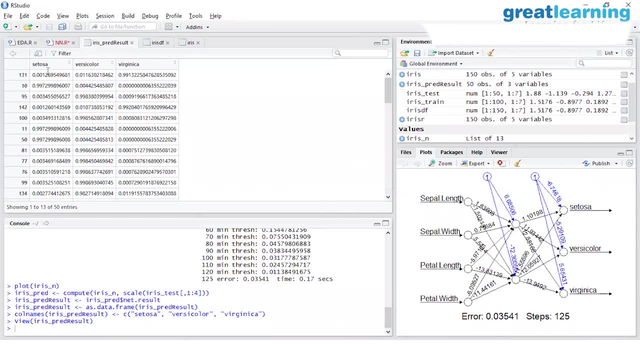 do a prediction. let's see how do we do that. so you see, we had three species which were possible and in the results that i got, i get these are 50 entries, which was in the test data set, and i get some scores for each of the species, like for this particular flower. 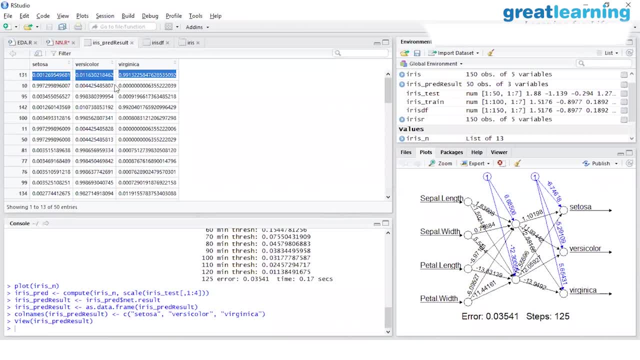 i get three values for each of the species. so the score- the probability that it is a setosa- is 0.001, the probability that it is versicolor is 0.01, whereas the probability that it is virginica is 99- 0.99, which is 99. so this flower, which is in the row number 131, will be a virginica. 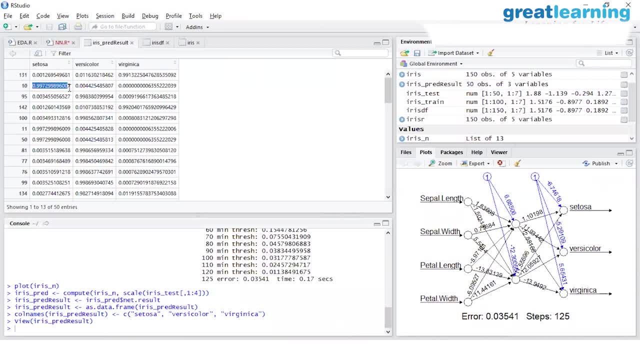 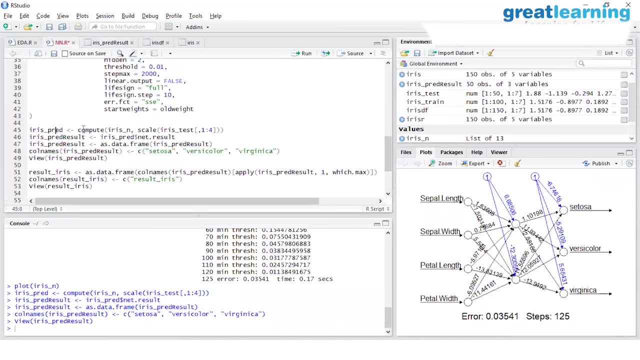 similarly, the flower which is in this row 10th will be a setosa. the flower which is in row 95 will be a versicolor. the flower which is in 142 will be a canna virginica. this one will be a versicolor. so what i'm essentially doing here is: 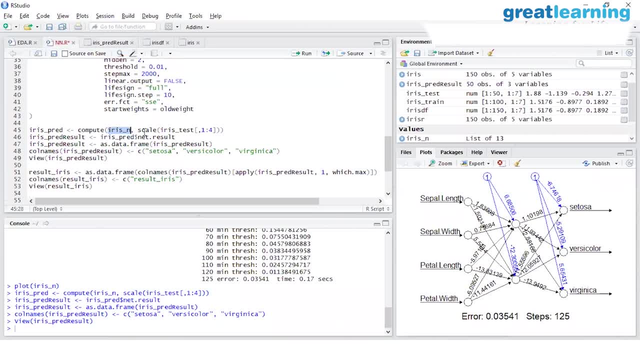 i'm trying to use the neural network model to predict what will be the class of my flowers in my testing data set. okay, so pass the testing data set. i pass the neural network model, which contains the learnings that it has from the training data set, and i'm use this to do. using this. 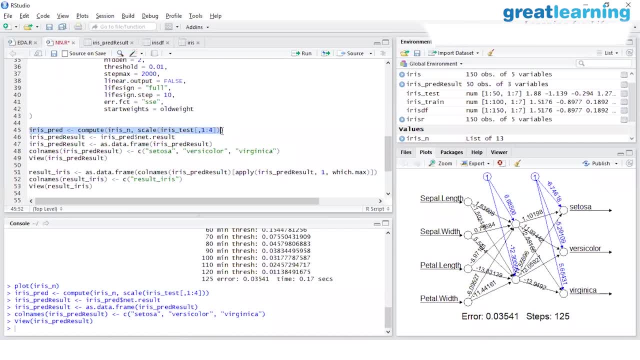 to predict. so this, this is the main step. do not get confused with the other steps, because i'm just doing kind of formatting to give you a nice looking output there. but with this step i'm trying to predict the values in the testing data set using the learnings i have from the 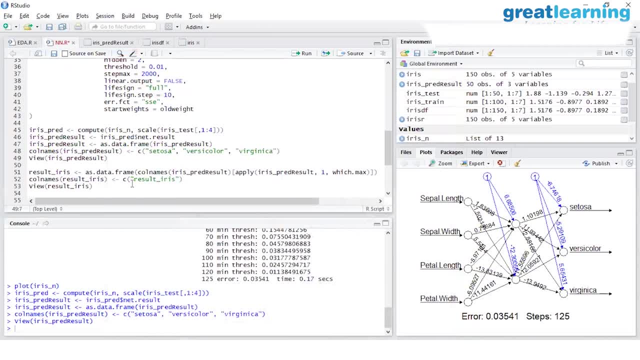 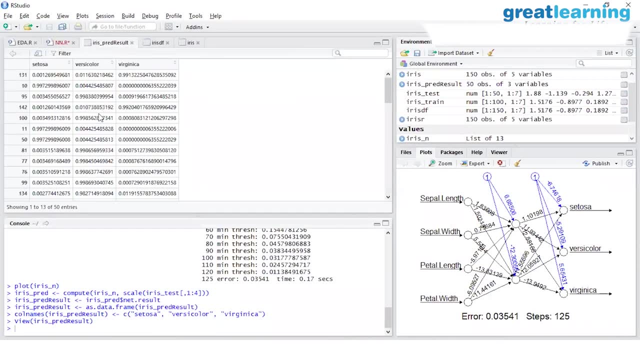 neural network model. okay, so with the results that i got here, i'll kind of try to compare it. so these are the predictions that my neural network model is making. these are the. these are the predictions that i'm trying to make for my testing data set using the neural network. but 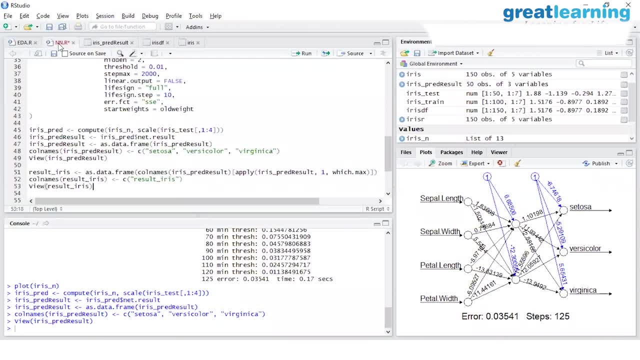 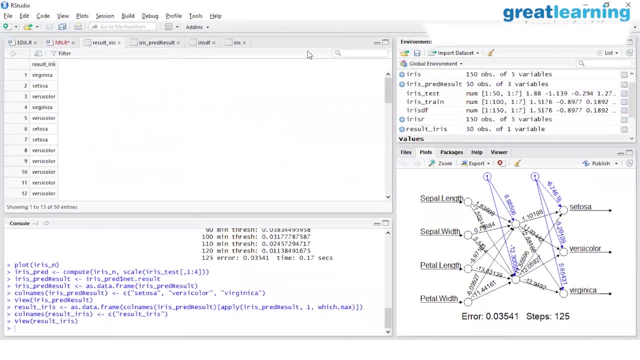 i should also be able to compare it to the actual values to see how good my neural network is doing. so, okay, what i did with this step was nothing, but, like i was telling you theoretically here on how this would be a virginica and this would be a. 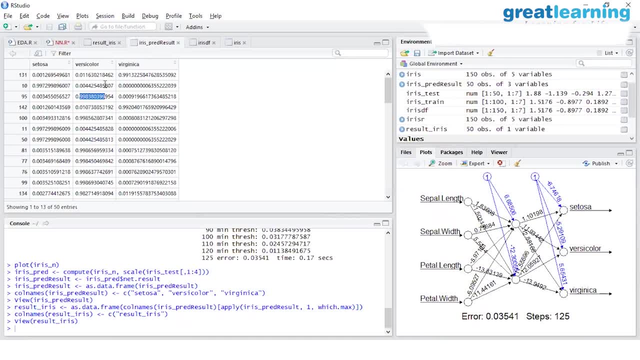 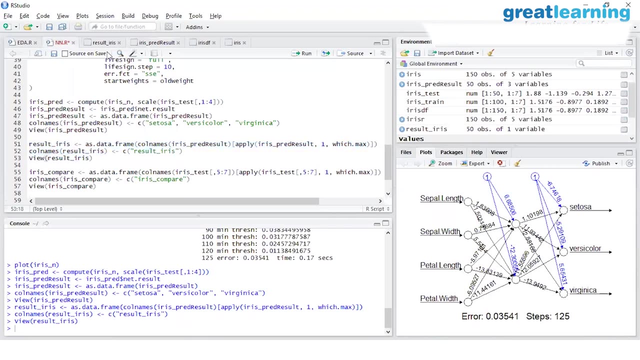 setosa, and this again will be a versicolor, so i kind of tried to put that in words so that we don't have to read through the numbers. so these three commands that i'm doing here are doing nothing but producing this result from this result. so 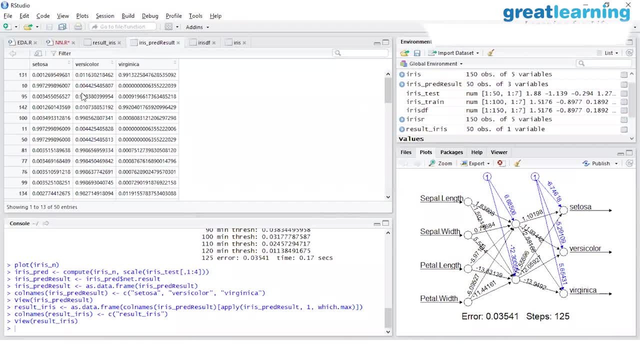 the first one should be a virginica, the second should be a setosa, the third should be a versicolor. this is what i'm doing here, telling r that whichever is maximum out of the three columns, i want that column name to come in my result. so this is: 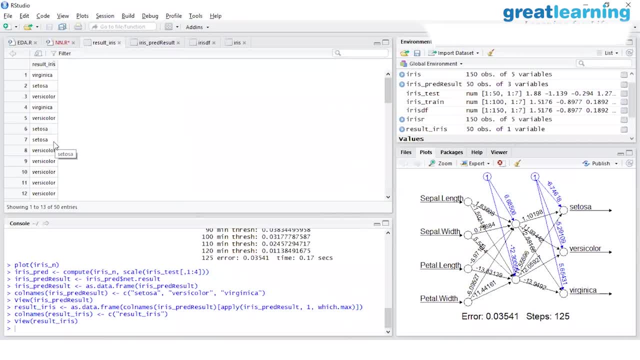 the result that i get as a result of prediction after my neural network for the 50 entries that i had in my test data set. these are the predicted species of the flowers using my neural network model. now i'll be using these 50 predicted values against the initial. 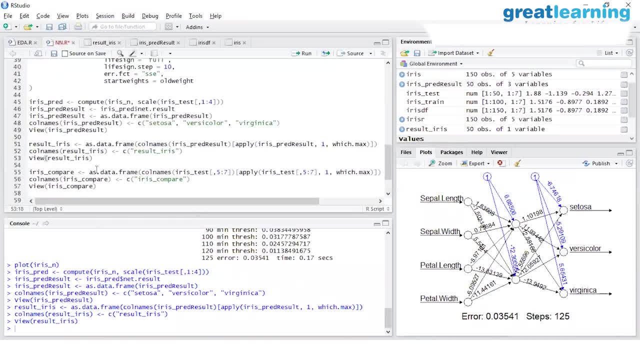 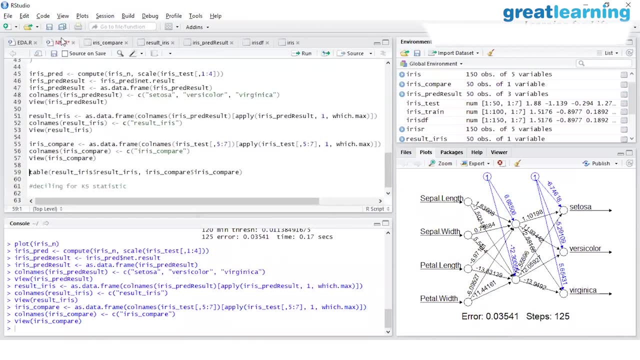 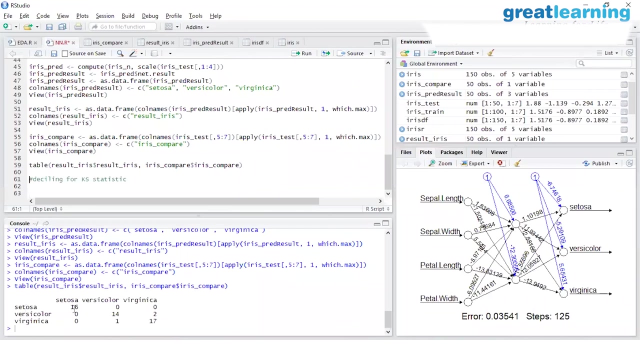 against the actual values to see how good my neural network is. okay, so these are the original values which were present and these are the values that i've got and we'll finally compare them in the table. so you see, we have out of 50 um. so this, this matrix, if you don't know it already, we call it. 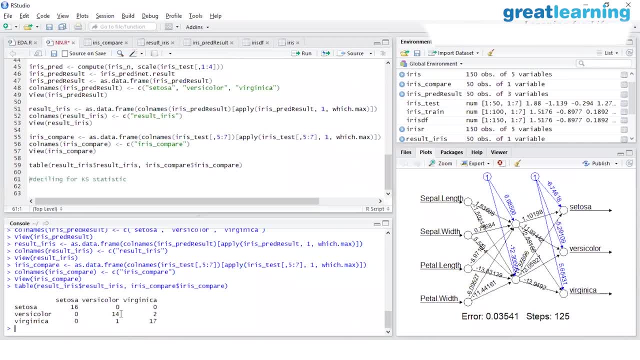 as a confusion matrix. uh, to see how good, how good our models do. so we see there is an error of three here out of 50. there is an error of three, so 47 values are being calculated fine, and hence the accuracy of this model is 94 percent. 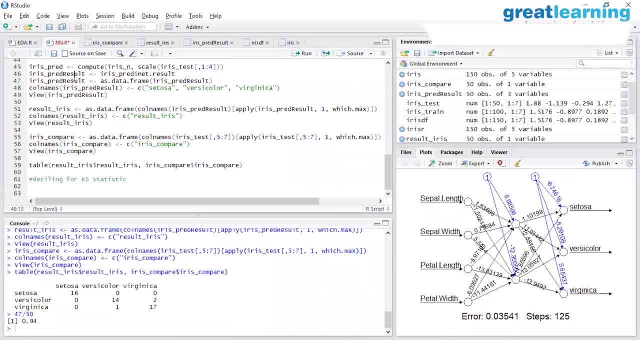 to tell you uh quickly again what i did here. i uh used my neural network model to predict what species each of my uh flower belongs to in the testing data set. then i compared it with um the actual species which were present, and finally i get this table which tells me that i have an 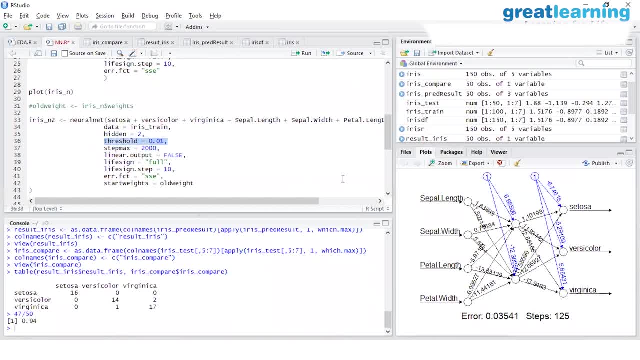 accuracy of 94 percent. okay, so weights will change according to the error. uh, whatever the error is, the end aim is to get a threshold of 0.01 passing whatever weights possible. so it is entirely possible that when you run this algorithm the second time- um, if you remember, here we had done. 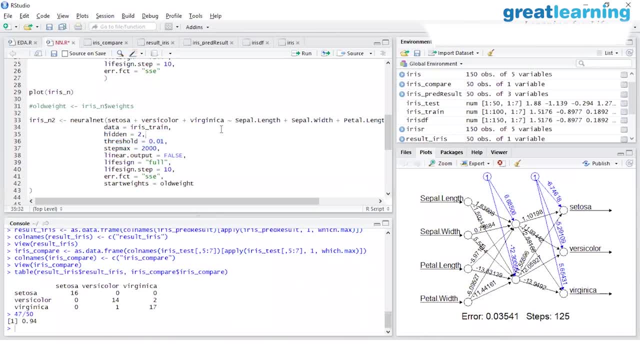 this with 125 steps. okay, when you run this the second time, it may take lesser steps, it may take more steps, but towards the end your result will be the same. okay, because the algorithm will stop when it achieves a threshold of 0.01. uh, just to tell you. i'm running this algorithm fourth time since yesterday. uh, once it has run. 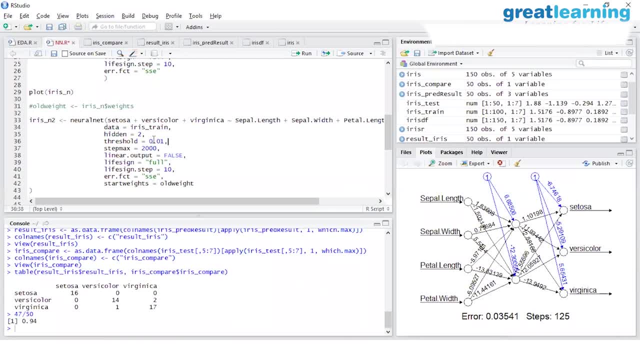 with 300 steps, once it ran with some 95, 96 steps and once it is running with 125 steps now, but your end accuracy will be: uh the same, the same, um, um, this thing, the same confusion matrix you'll get, no matter how many times you run the same algorithm, because it will use the threshold to stop and 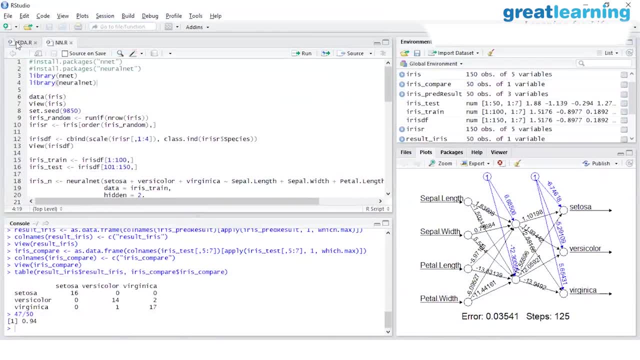 the weights can be anything, okay. so, uh, for today's session i'll just be doing an um exploratory data analysis that will help you just see which variable should be used and which should not be used. what's the next session? we'll try to actually solve it to see which uh. 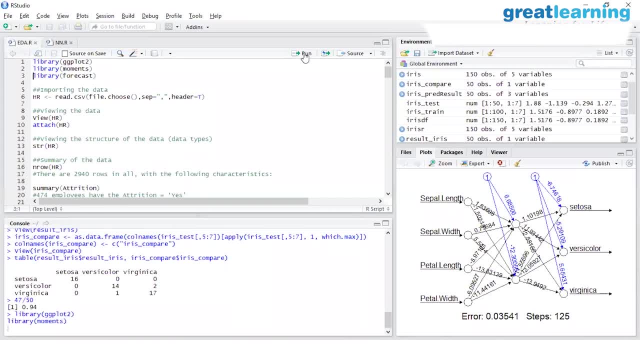 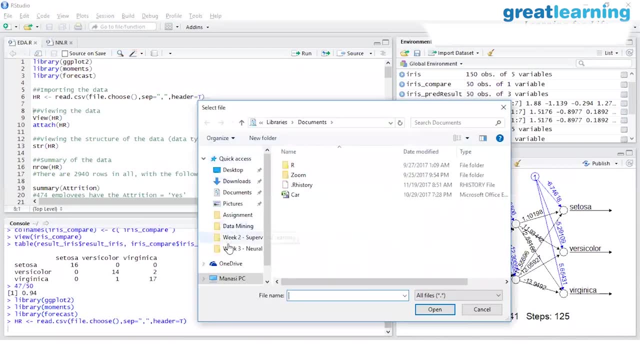 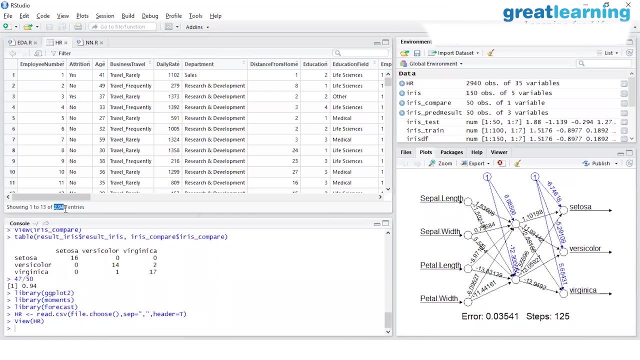 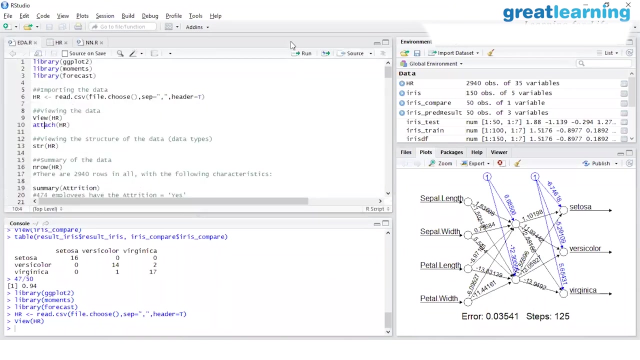 what is the output that each of the algorithm throws? okay, i'm importing the data set. okay, so when i'm viewing this data set, it contains approximately 3000- uh, or like 2940 rows, and it has 35 columns. um structure is just an additional step to see what the structure is. 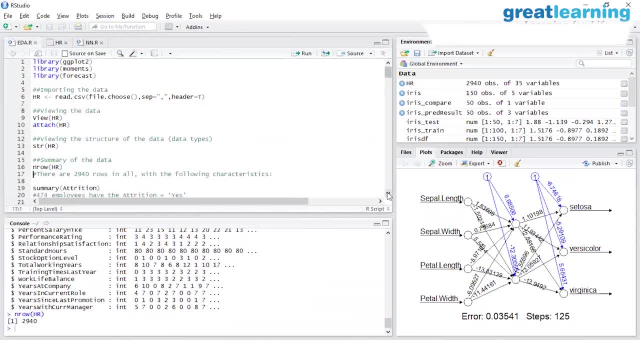 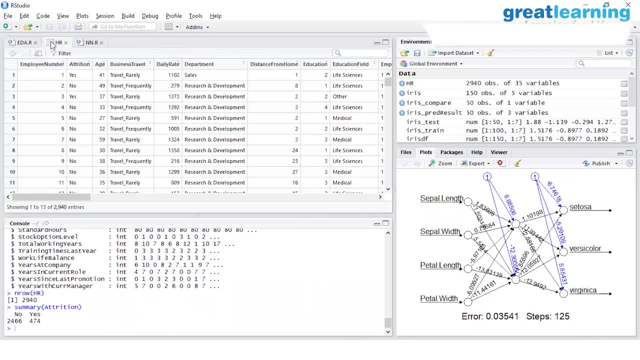 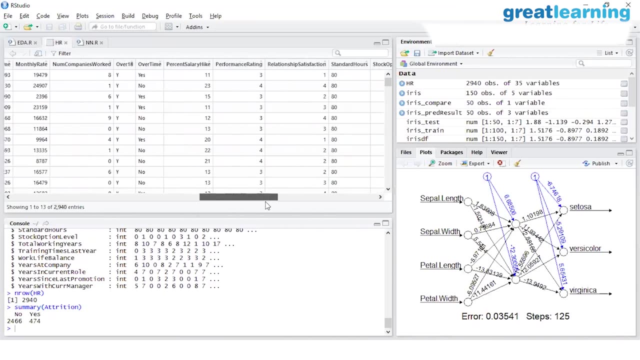 so we have a total of 2940 rows, and then we'll now go to each of the variables individually. so when i start off with the address and variable, one thing to note here is that these variables have been arranged in an alphabetical order. so you need to if for 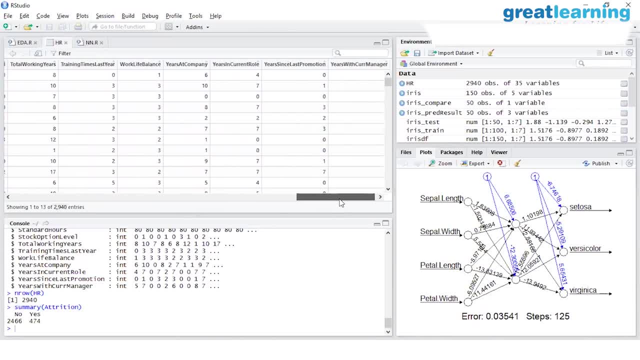 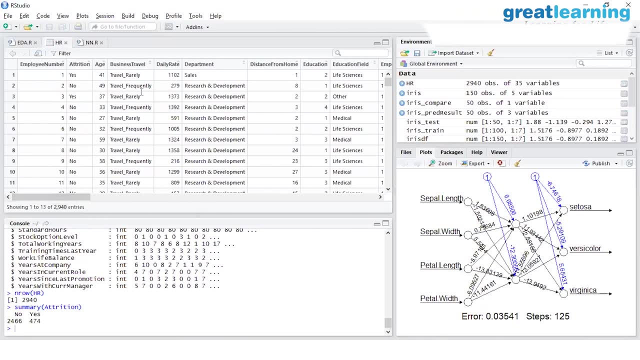 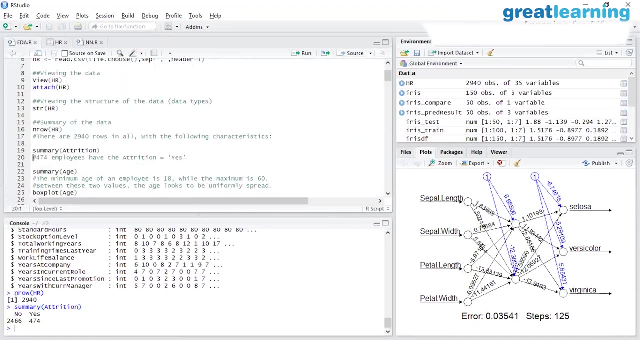 better understanding, you might want to rearrange these columns so that similar columns are together. I haven't done that, but maybe you can do that, arranging the similar columns next to each other so that it becomes easier for understanding. so we see here when we start off with that attrition, so there. 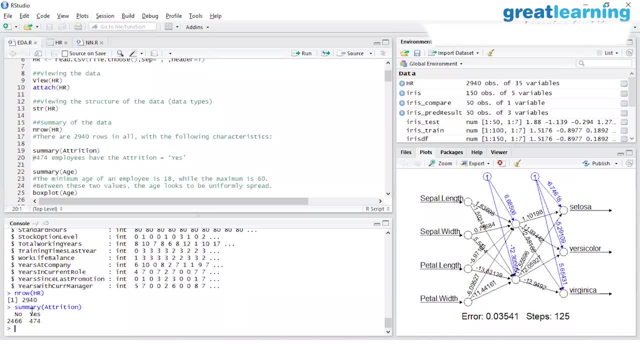 are total of two 9 4, 0 employees, out of which 474 had an attrition, so that becomes 474 upon 255. so approximately 16 percent of people had an attrition and we'll see what impacts the attrition of these 16% of the. 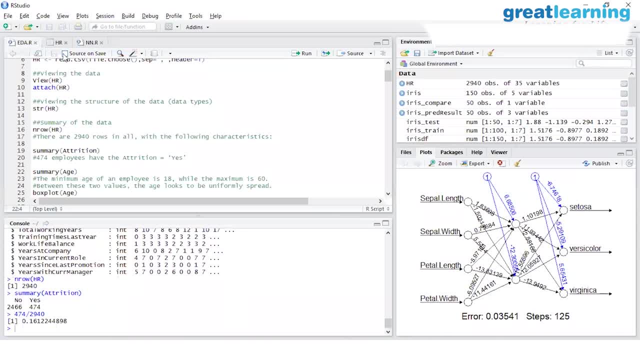 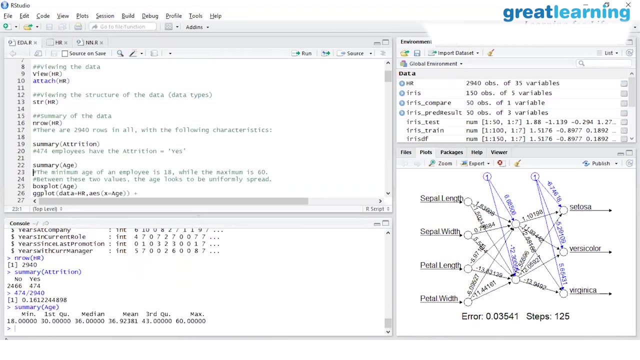 employees. okay, so we'll start off with each of the variables one by one and see whether or not that variable should be included here. so I am starting off with the age, which is the first variable here. so you see, the minimum age is 18, the maximum is. 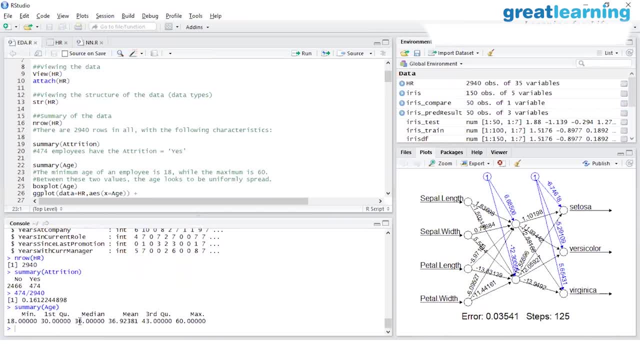 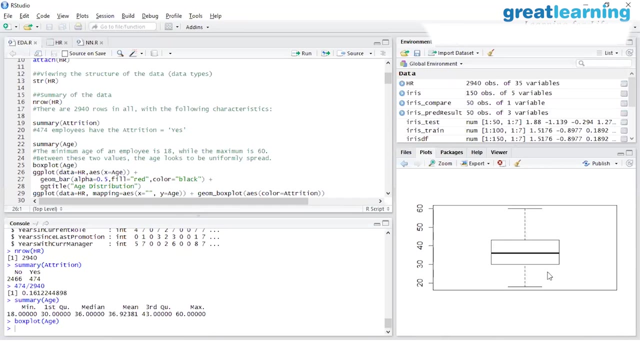 60 and the median- excuse me, the median- is 36, which is somewhere in the mid. so the data looks like not being very skewed. we do a box plot of it and we see that it looks like a normal curve. the age: so there are people from the ages 18. 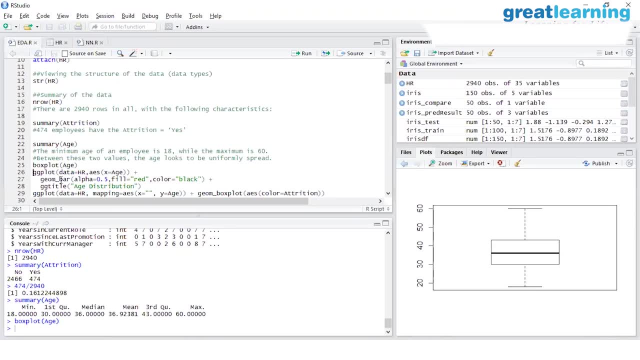 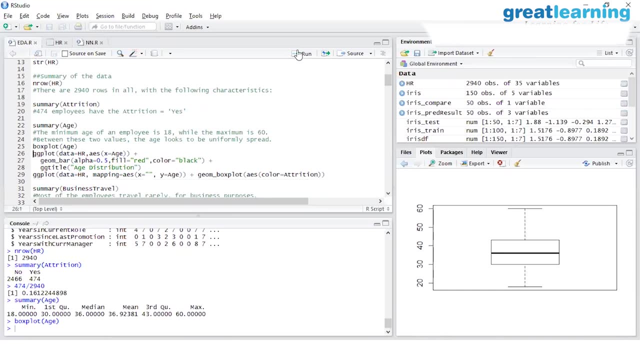 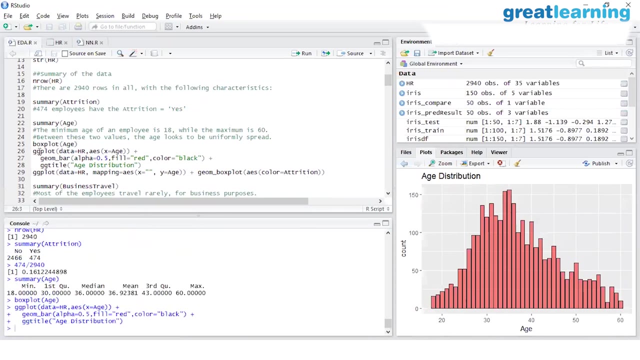 to 60 and the data is normally distributed. now I'm trying to see. so this is another way I did a box plot and this is another way to do a clearer histogram. we could have done it using the haste function as well, but you can also use ggplot to do a histogram, which gives you a more precise. 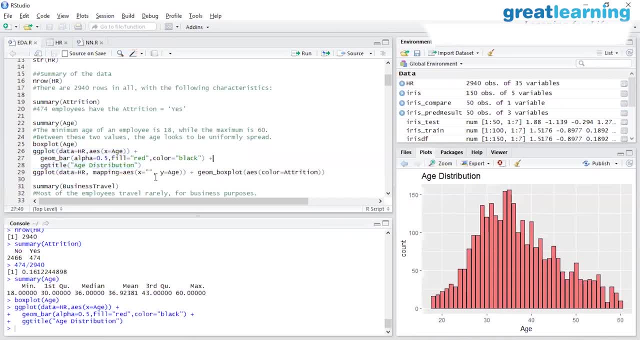 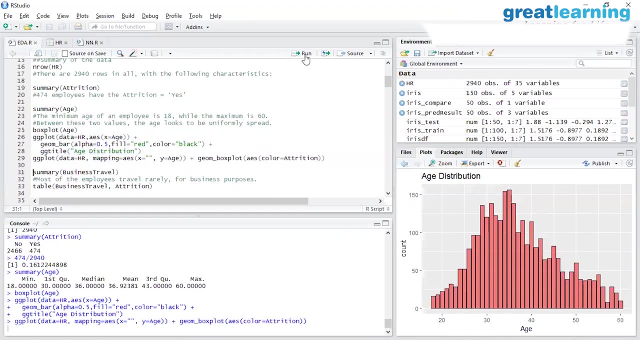 histogram to see the distribution of the age and finally, I'm again using ggplot to see the impact of age. so what I did here was for the continuous variables that were there with the data set. I'll try to see whether what is the impact that those variables have. so this is the continuous variables that were there, with the data set. I'll try to see whether, what is the impact that those variables have. so 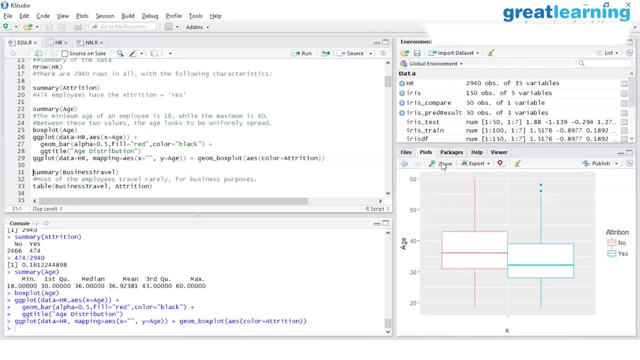 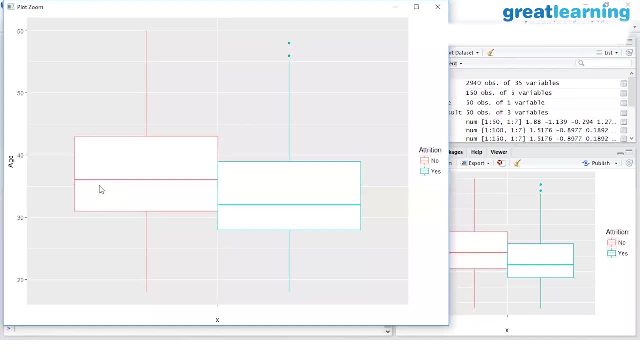 when I do a ggplot of the age, I get an output something like this: so what this tells me is: the pink color shows the employees that have an attrition and that do not have an attrition, and the blue color shows the employees that have an attrition. so what this tells me is that the people who have an attrition or 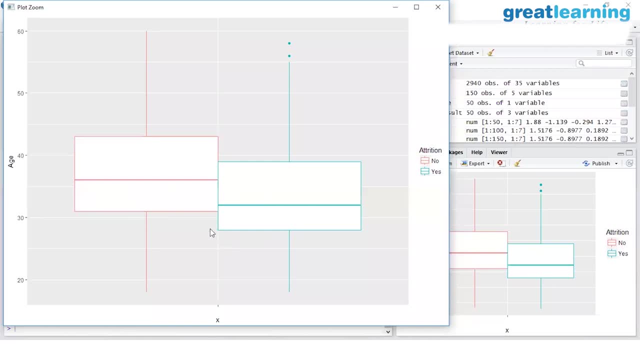 who had an attrition are belong belong to the age somewhere from probably 28 to 38 to 39, and the ones that who do not have an attrition have an age somewhere from 31 to, say, 43. what this tells us is that when you're 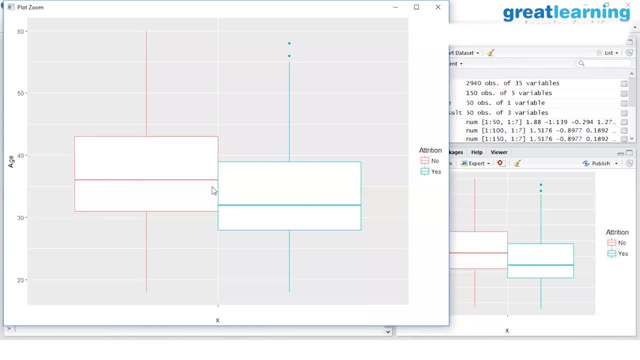 seeing just the age variable alone, there is a difference in the ages when the people have an attrition or not. so people in the smaller, in the younger age groups are more likely to have an attrition compared to people in the Illinois larger age groups. so this helps us understand that when we see the impact of age alone with 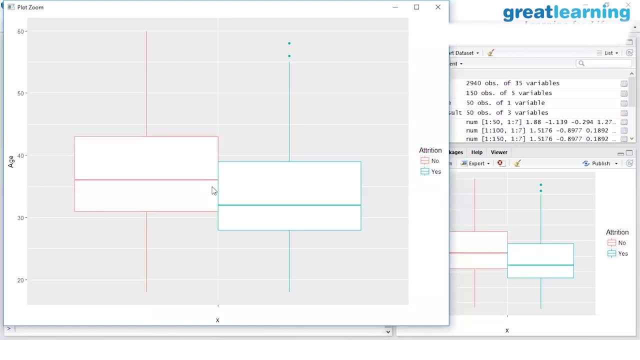 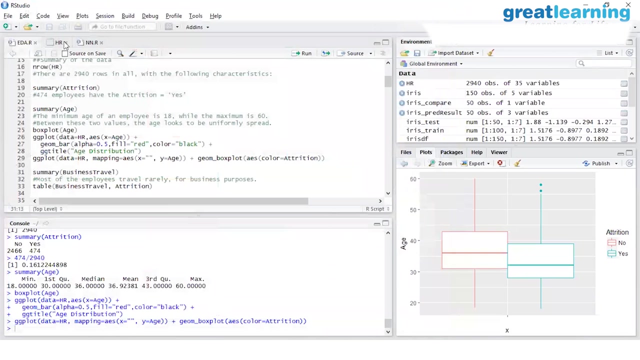 attrition. so age is an important variable when we are trying to study attrition, because there is a significant difference with this graph. so the age should be included as a variable, as an input variable when we are trying to do the modeling. okay, next we'll go to the second variable, which is business traveler. so it is a categorical variable. 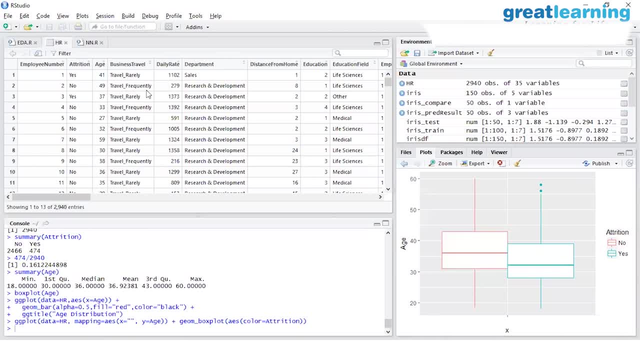 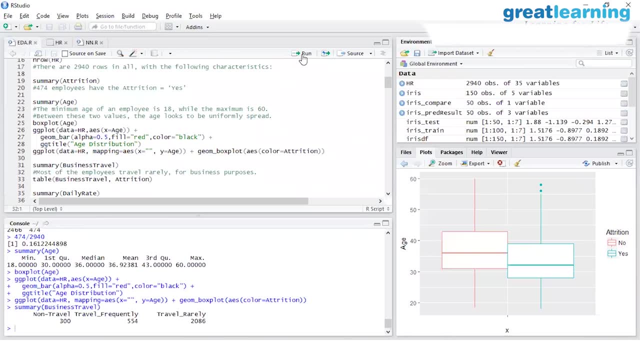 that tells us whether or not a person travels for business and how often he travels. so, out of the 2940 employees that we have, so we see that most of the employees travel rarely, and then we'll try to understand whether or not traveling happens has an impact on attrition. so since this is a categorical variable, i just created a simple 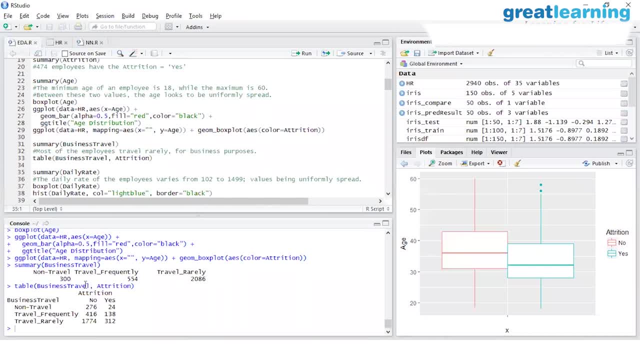 table to see if there is an impact of business travel and attrition. so we see the ratio that you see between the no and yes here. so for non-travel, the ratio of 276 to uh 24 and 416 to 138 and 1774 is 2312. this is almost similar. there is no much difference uh. 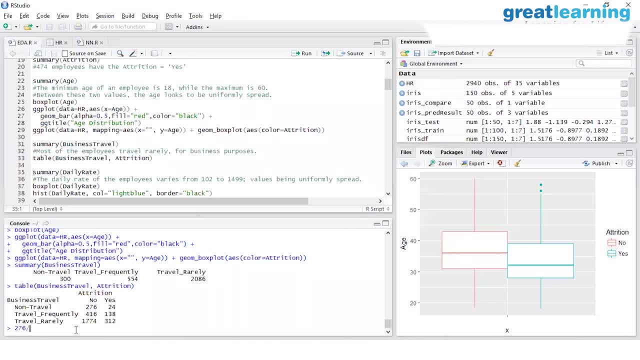 let me do actual numbers: 276 by 24, 416 divided by 138, 1774 divided by 312. so there's not much difference um in the people who travel um to see whether or not they have an attrition. so you can choose to ignore this variable because it doesn't look like um it is having an impact on whether 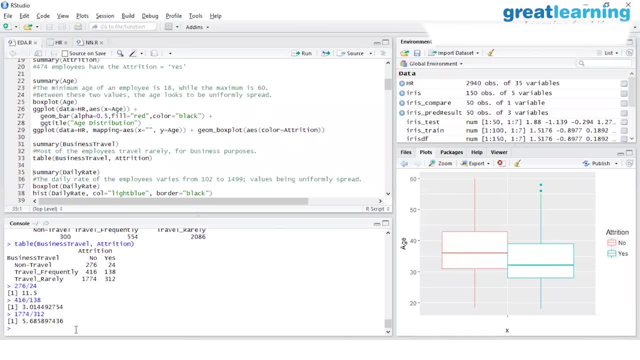 somebody or not has an attrition from the organization. okay, it, we saw, has an impact, but, uh, the business travel does not look to uh have a significant impact with. um, the business travel does not look to have a significant impact with attrition, so you can choose to ignore it okay. 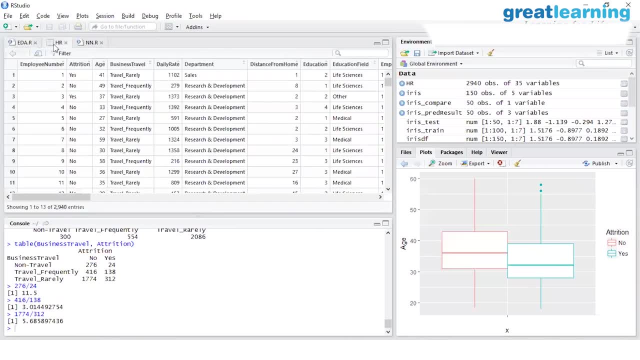 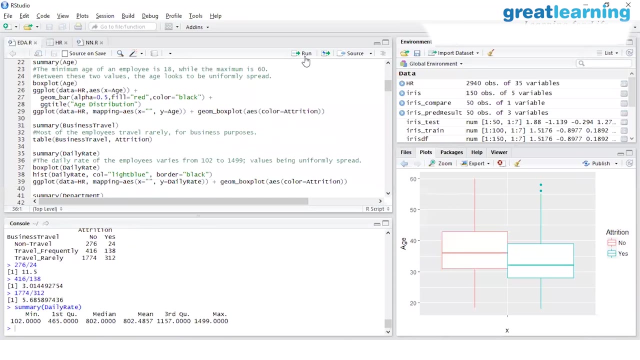 similarly, we go to next, um, the daily rate. so daily rate is again a continuous variable, uh, which shows the uh rate at which an employee is being paid on a daily basis. so when we see a summary of it, it is again a continuous variable, the minimum being 102 to a. 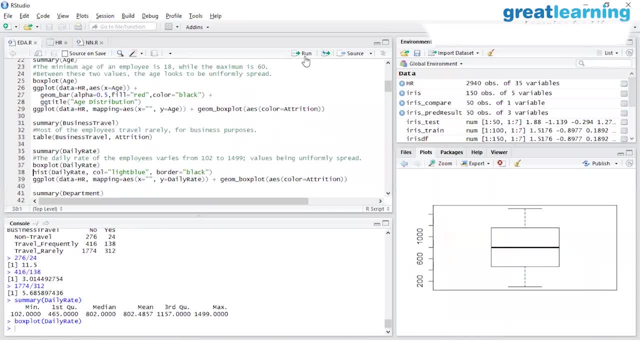 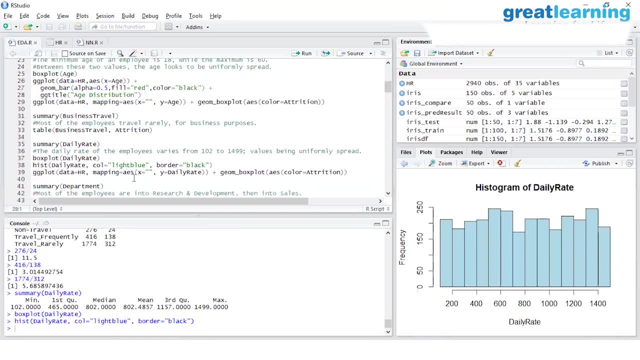 maximum being of 1500. uh, when i do a box plot it looks like a normally distributed data and you can also see that from a histogram as well. uh, but a good thing to see here is, if i do the impact of daily rate on uh attrition. probably the daily rate does not have a very significant impact. let's say: 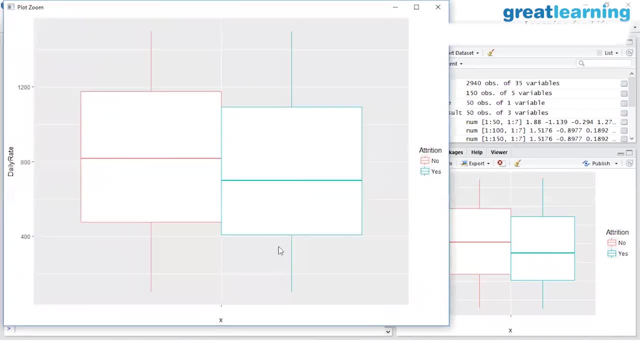 which is an esa graph here. so let us say i want to subtract, you know, between 8 and me, 0.6 energy free product input. on attrition, the day level is 113, so that is 5��, which is normal on an average, even if i plug about 125 or more would usually be ok. она if i compared to 21st, so which is in fact. 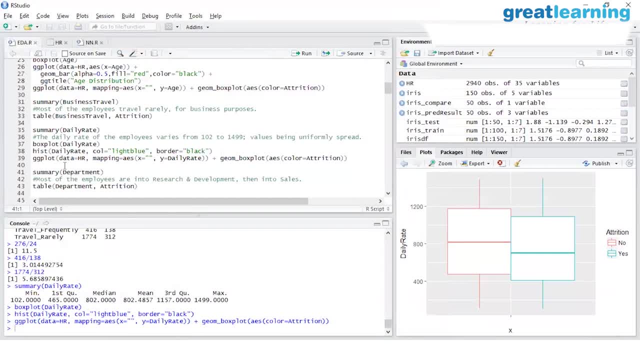 five times a day on your daily rate. so if i plug about 124 and you'd find out: pros are paprika of reason to plus cons. this is because preoccupation to a minimum freedom from first and to then you use inventory impact. Let me go back to the histogram again to show you. So see almost all of the daily. 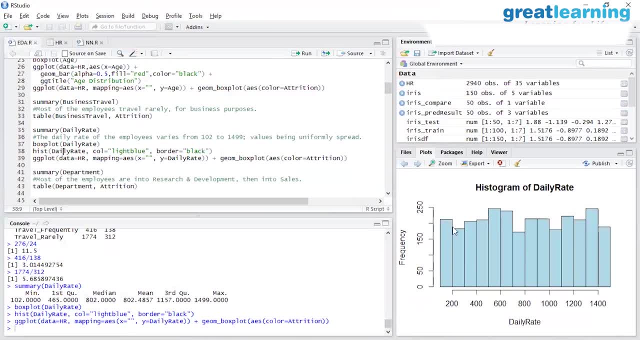 raters uniformly distributing, meaning to say that across all the 2,900 employees that we have, the daily rate was evenly distributed And when I did a comparison of people who were right or not from the organization based on the daily rate, there is no significant 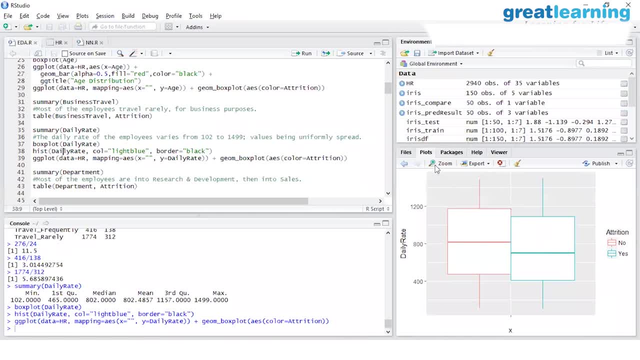 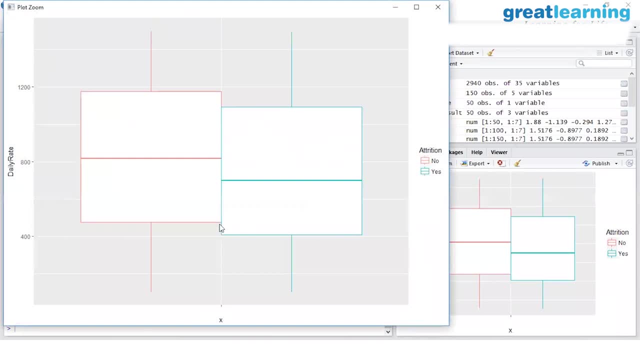 difference. There is a very small difference here. If I zoom it out, So this is 400 to 600.. This is somewhere around 450 or so. So there's not a very significant difference compared to the range of daily rate that I have. There is not significant difference. 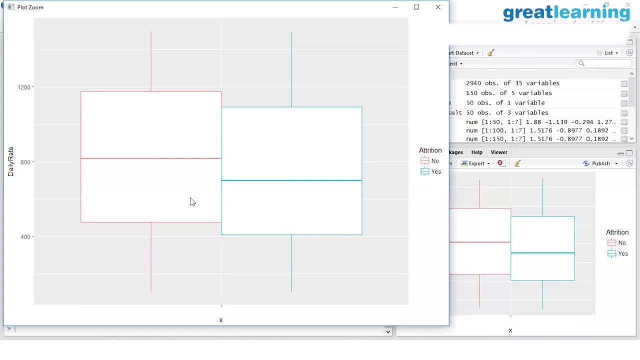 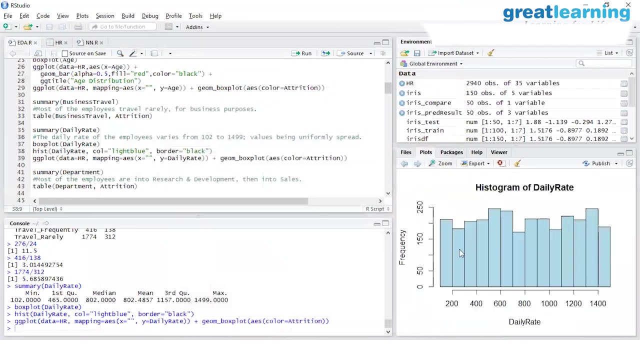 in the daily rates of people who have an attrition or not. So even daily rate you can choose to ignore when you're doing the modeling. With age we had a significant difference With daily rate. we do not have a significant difference And also we saw from the histogram that the daily rate is not very varied. It. 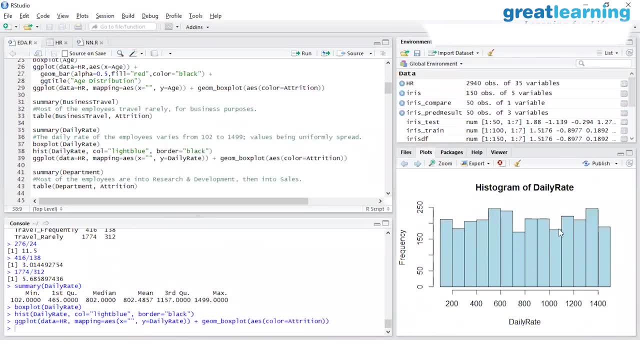 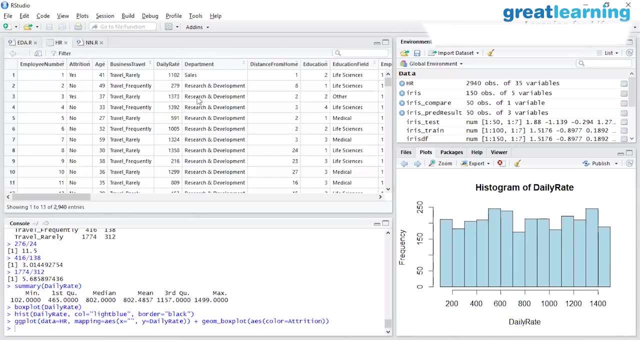 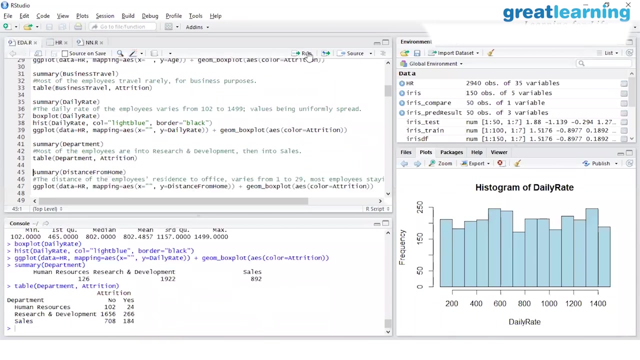 is almost constant. The frequency of the daily rate within the employees is almost constant, So it doesn't look like having a very significant impact. So you can choose to ignore the daily rate variable as well. Next we go To the department, which is a categorical variable. So we'll just see a summary of it. 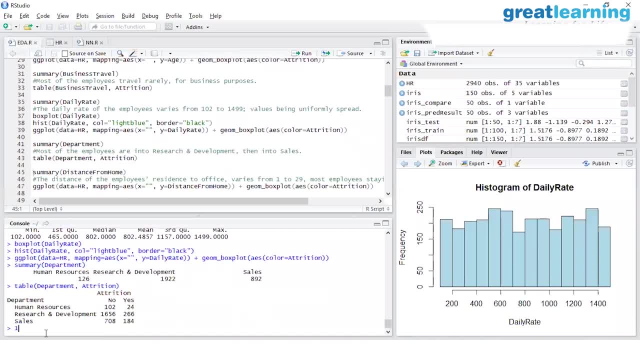 So see, this is significant here, with the human resources: 1656 divided by 266.. And so this is evident in the data as well, But I'm trying to show it more clearly. Okay, So with the department as well, the ratio between no and yes is almost similar, Okay. 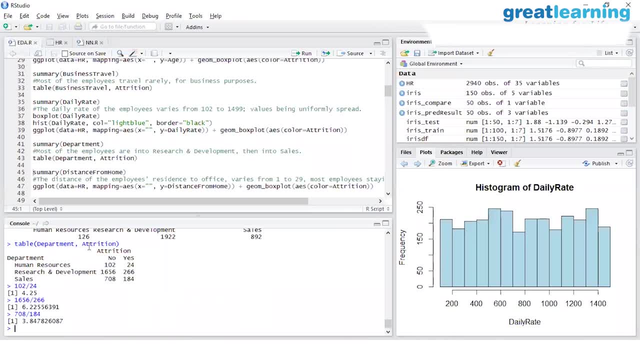 the people who are at right versus the people who do not at right is again similar. So, department: again, you can choose to ignore, because there is no significant difference with respect to Nothing, like people of a particular department have more affirmation compared to people of other departments, So you can choose to ignore this variable. 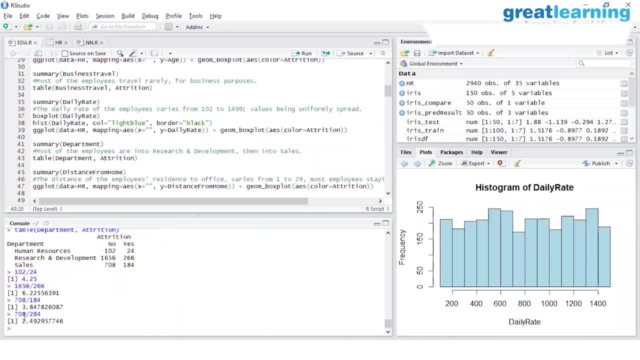 Well, okay, so then may be okay to 84 results: Okay. So then you'll see that there is a difference, significant difference, with the other departments. So if you see that for a particular department, The ratio between no and yes is even more significant with respect to the people of a particular department, maybe 384.. So there is a significant difference with the other departments. So if you see that for a particular department, the ratio between no and yes is almost similar to that of a part. 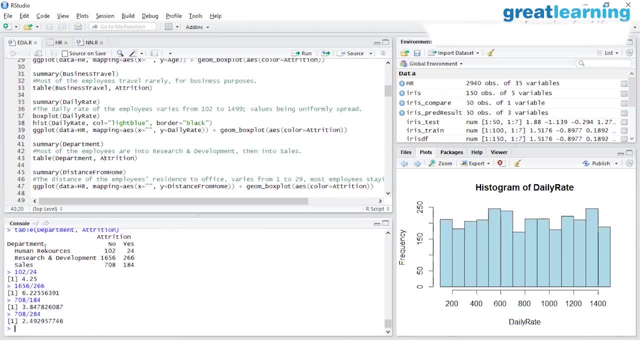 the ratio between no and yes is different for a particular department compared to other departments. So then you say that people of those that particular department have a more attrition rate compared to people of the other departments. So that will mean that that particular department has a significant importance. when you're sorry, yeah. when you're creating. 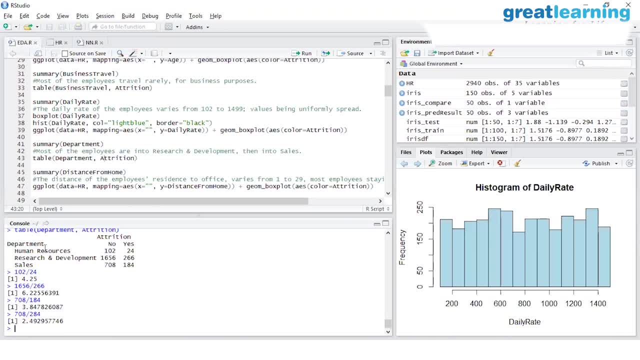 a model. that department variable has a significant importance and hence it should be included, But with the current data set that we have, there is no significant difference with each of the departments, So you're okay to ignore it. Okay, And this is what happens when in 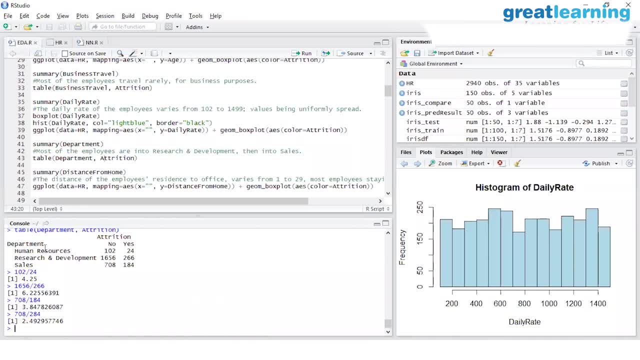 the industries when we are actually working. So this, this is again a data set with 35 variables, but this is again not huge. We had actually worked with one of the data set that had some around 170 variables or something like that. So we need to. you know, most of the time, most of the time gets spent in doing the 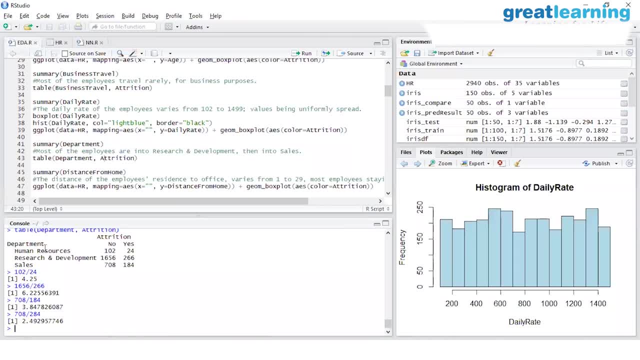 exploratory data analysis only because the models that you're creating, like the neural network I created here, is a two-liner command that you can execute within seconds. If the data is huge, that command will take a minute or maybe one and a half minute to run. 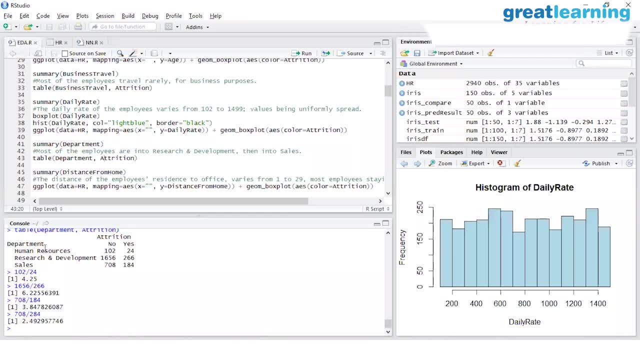 but then it's not a big deal. So it's not a big deal. So it's not a big deal. It is again a two-liner command that can be executed quickly. Most of the time that goes in, the organizations is doing the exploratory data analysis, and that needs to be done for. 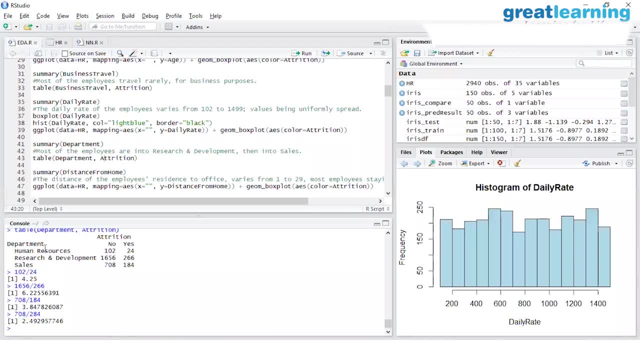 each of the variables here. So here, with this data set, I haven't done so. I had. I had seen an overview of what the summary was. So this, this doesn't look like a data which contains outliers. So in actual data, in the actual data that you'll see, there'll be outliers. 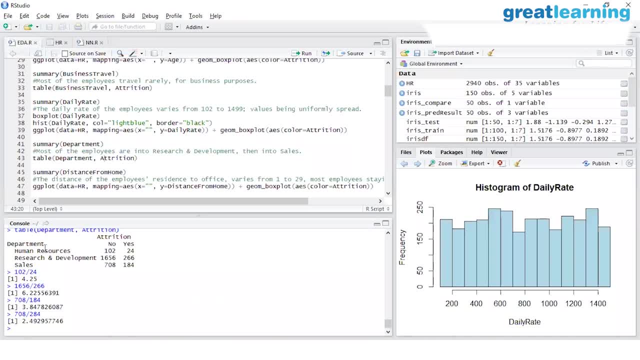 as well. So how will you understand what the outliers are? How will you understand the outliers? How will you understand whether or not the data has outliers is by studying the individual variables. Okay, you study the individual variables. whichever variable you see looks like having an outlier that needs to be treated If there's a missing. 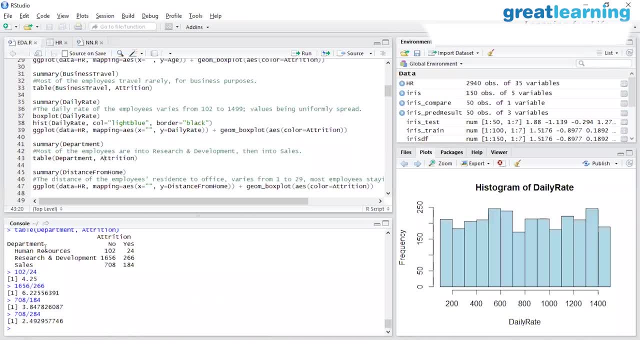 value within within a data set that needs to be treated. And finally, using the summaries of each of the variables, you need to decide whether or not that variable needs to be included in the data set. So I've done that for each of the variables. So I've done that for each. 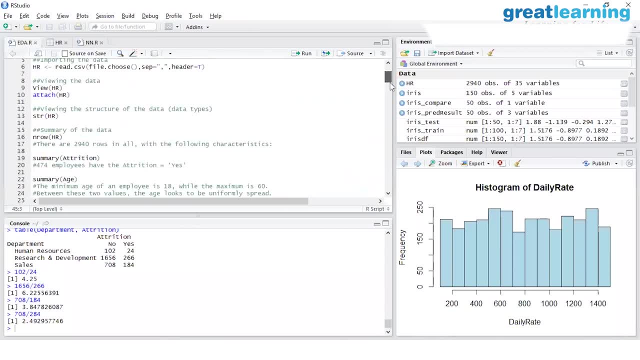 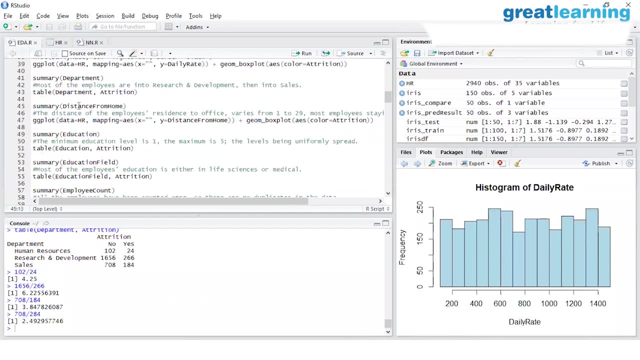 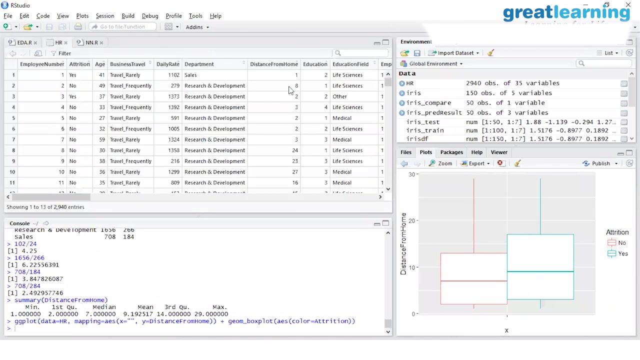 of the variables. Since this is clear now, I'll quickly run through all the variables. So when you do this exercise for the mini project that you're doing, repeat these steps in a similar manner for each of the variables. Then you also have this distance from home. 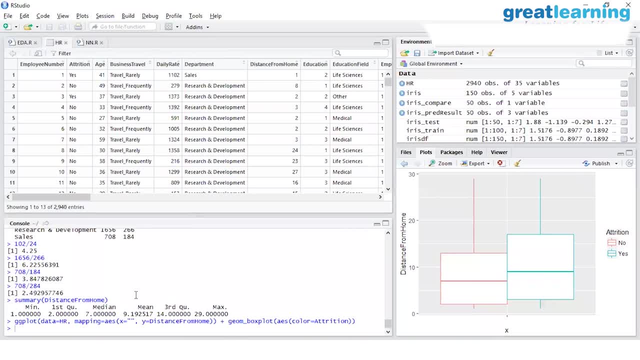 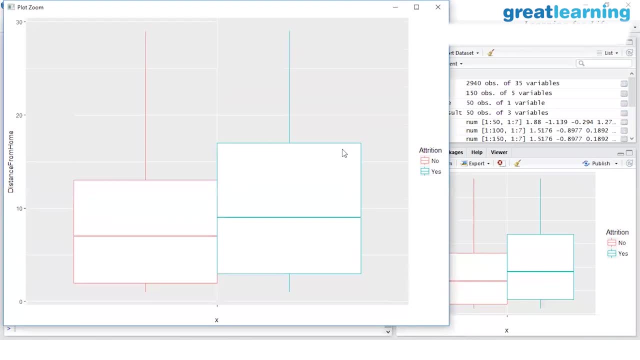 So that tells the distance of the employees home from the office, which is a number from one to 29.. And if you zoom this out, this is very, you know, intuitive as well that people who have so distance from home to your office is a significant factor And that is. 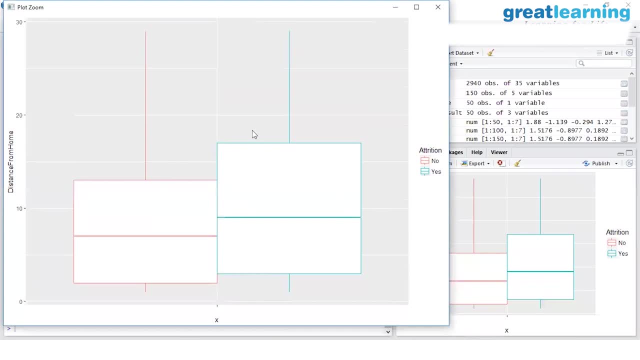 also evident from the data. So you see people who have more distances from home, like the yes is the yes is in the blue color. So people who have more distance from home are more likely to have an attrition compared to people who have more distance from home. So this: 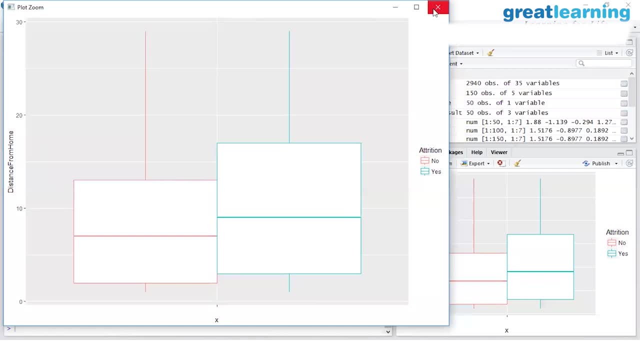 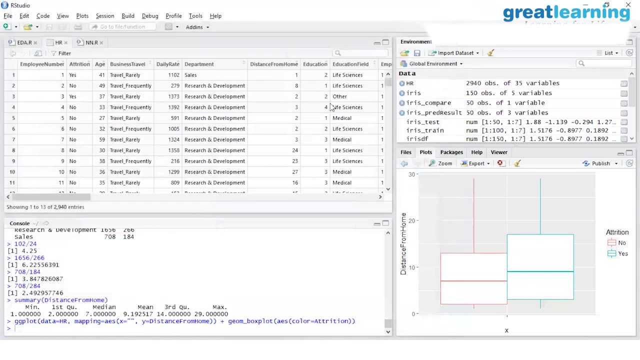 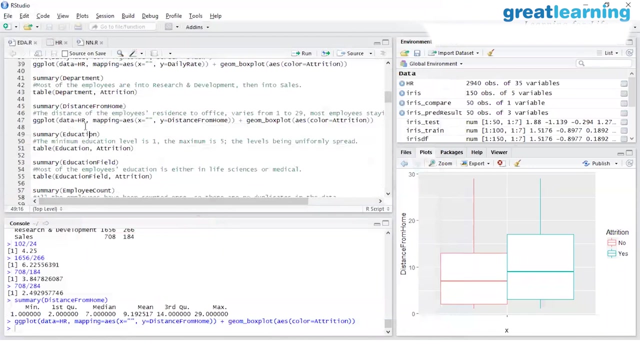 means that people who have lesser distances from their homes. so distance from home is a variable which should be used as a factor for impacting attrition. Next is the education level and the education field, which are categorical variables. So we'll just see a table of them. 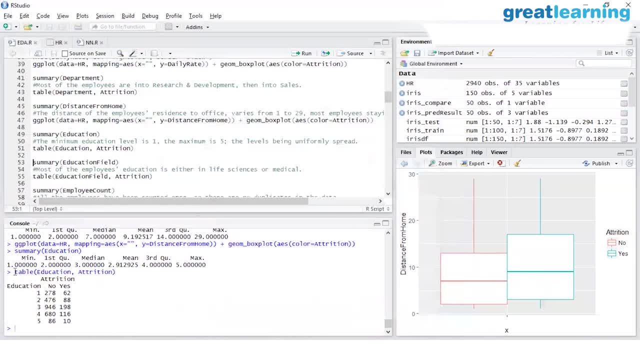 here. So with this table, I am not doing the actual ratios here, but do the ratios that you see here. So I'm going to do the actual ratios here, but do the ratios that you see here. So with this table, I am not doing the actual ratios here, but do the ratios that.